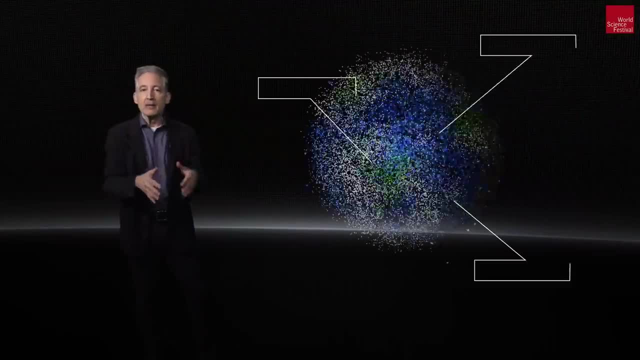 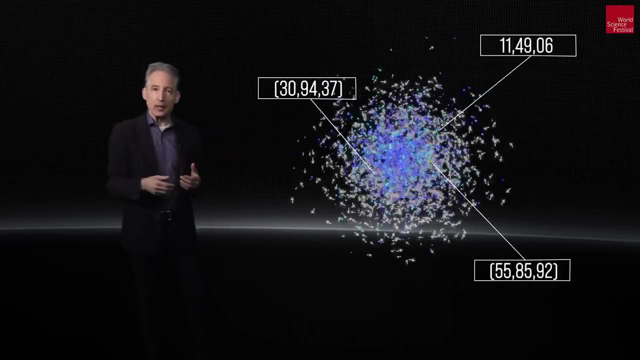 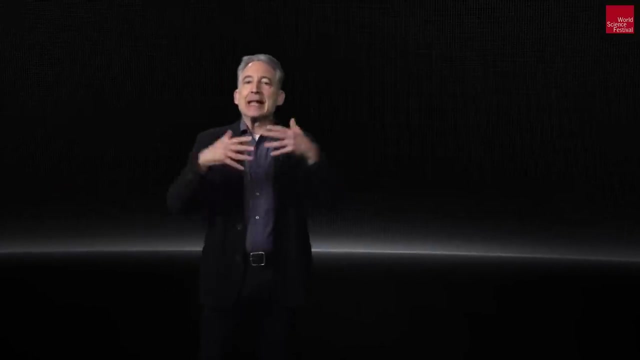 if you specify how the world is right now, the positions and velocities of all ingredients, and you specify the forces acting on those ingredients, the laws predict how the world will be at any subsequent moment. The framework: it's sleek, it's elegant, it's powerful and it's 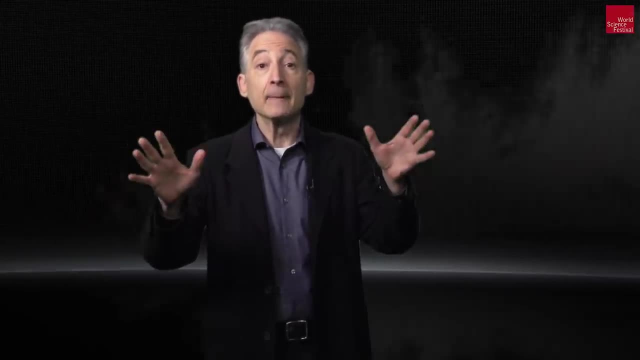 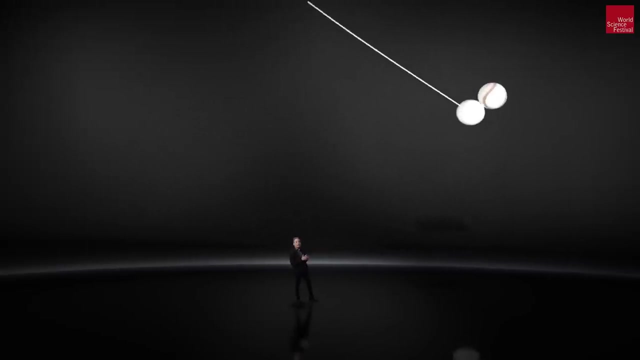 rigid in its determination of the future, And it worked. The predictions about the future wear off a pendulum: The world would be as it swung, where a ball would land when thrown, where the moon would be in its orbit around the earth. All of these predictions and every other that was made, all of them were. 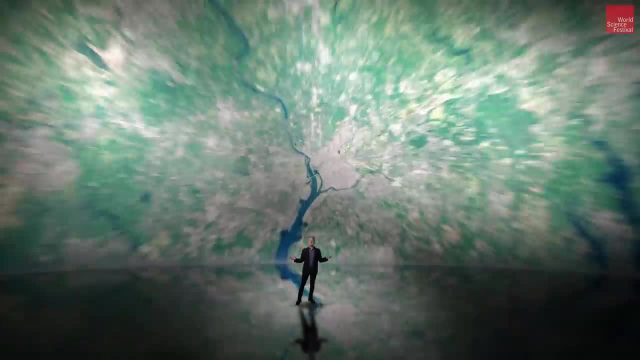 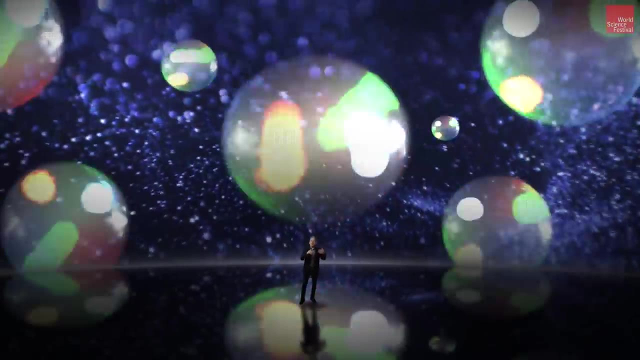 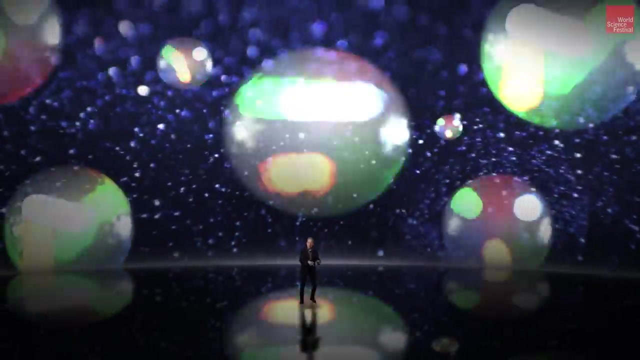 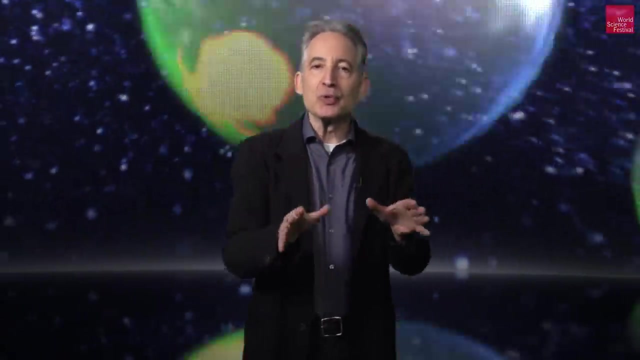 spot on accurate. That is, until the early years of the 20th century, when scientists gained the capacity to explore the micro world, the world of molecules, of atoms and subatomic particles, Because in this realm the predictions from Newton's math were they were wrong. The data revealed that new rules were needed to understand the microscopic realm. 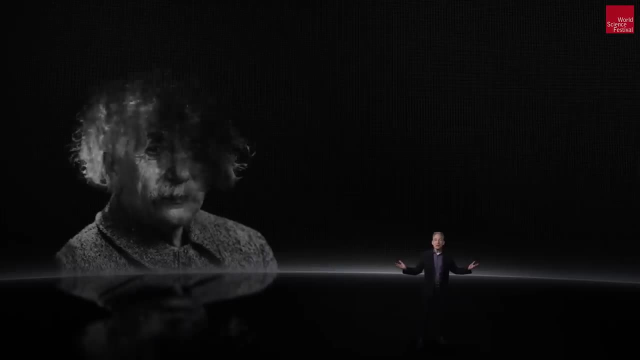 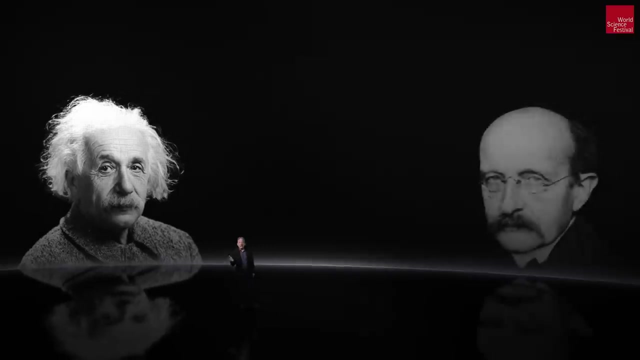 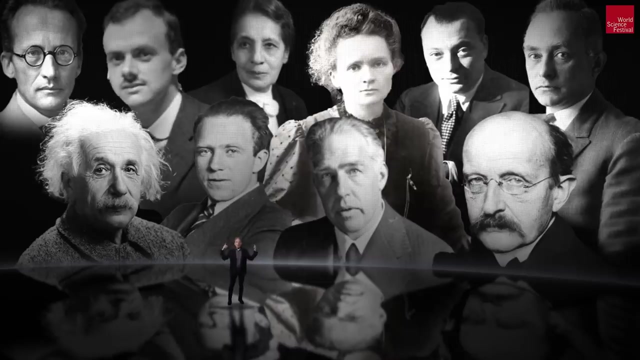 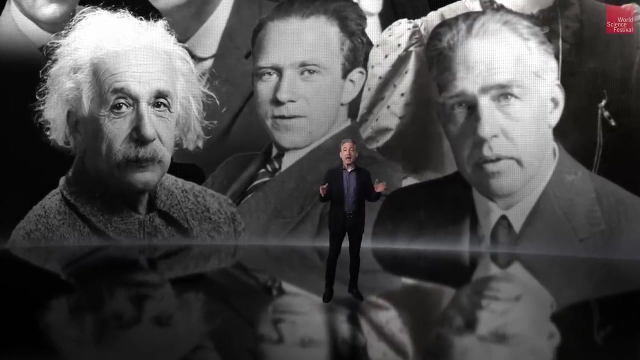 And, remarkably, within just a few decades, a generation of scientists, including the likes of Albert Einstein, Max Planck, Niels Bohr, Werner Heisenberg, Erwin Schrödinger, Max Born and many others brilliant thinkers, ushered in a new understanding called quantum mechanics. Now quantum mechanics. 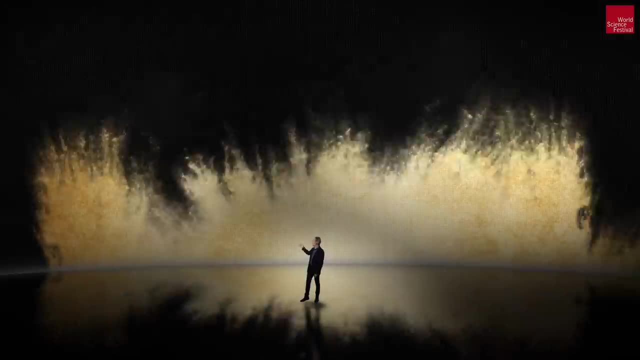 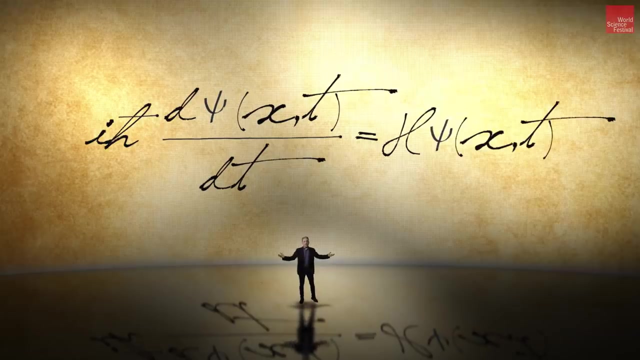 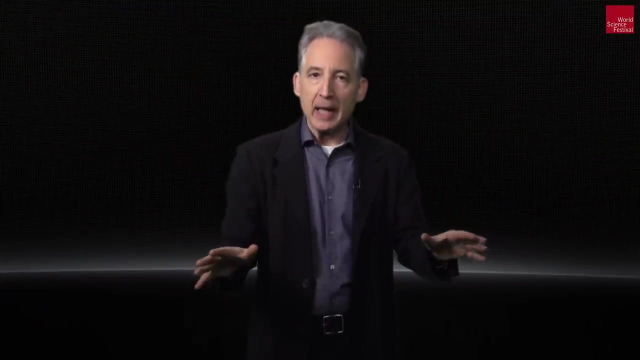 it comes with its own powerful mathematical formulation, But again, one can grasp the central new idea of quantum mechanics even without the math, Whereas Newton said: tell me how the world is now and I will tell you how the world will be tomorrow. 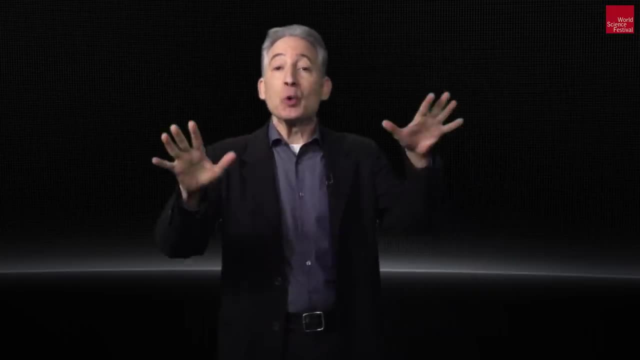 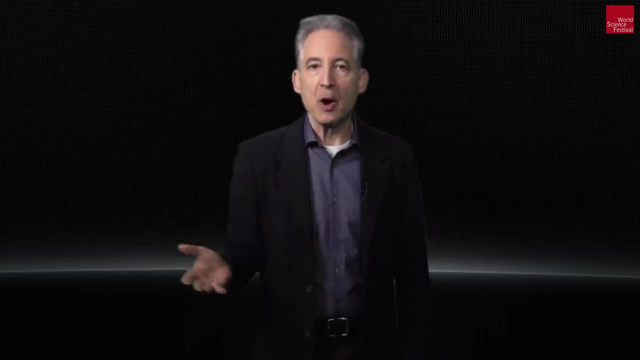 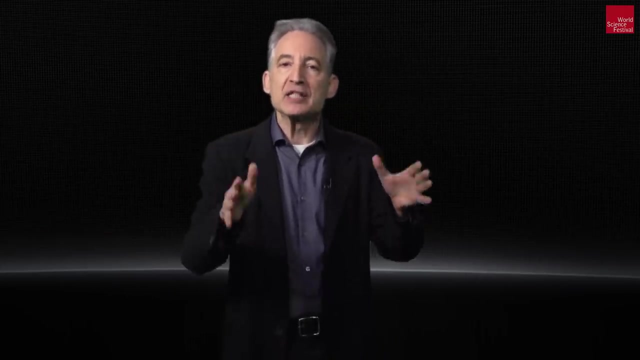 Quantum mechanics says: tell me how the world is now and I'll tell you the probability that the world will be one way or the other tomorrow. And, according to quantum mechanics, these probabilities provide the deepest and most precise description of the physical unfolding. Gone, completely gone. 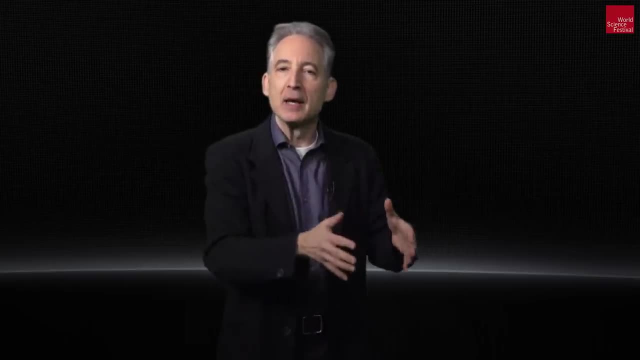 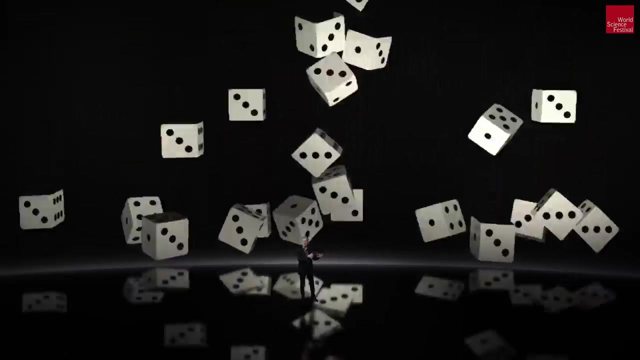 according to quantum mechanics, was the rigid certainty of the classical world. Now, much has been said about quantum mechanics, but it's not the only thing that's been said about quantum mechanics. Einstein's resistance to the probabilistic nature of quantum mechanics, the famous and 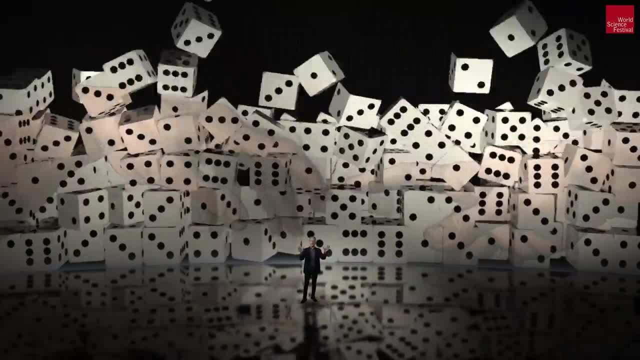 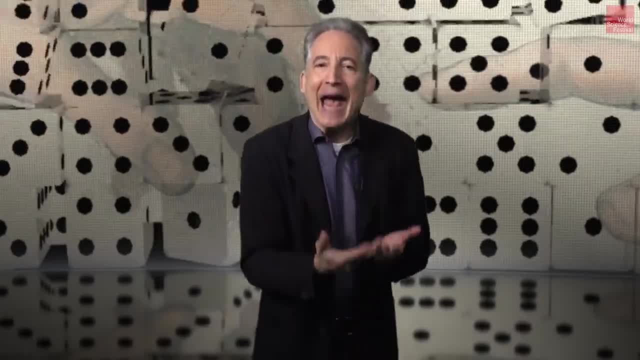 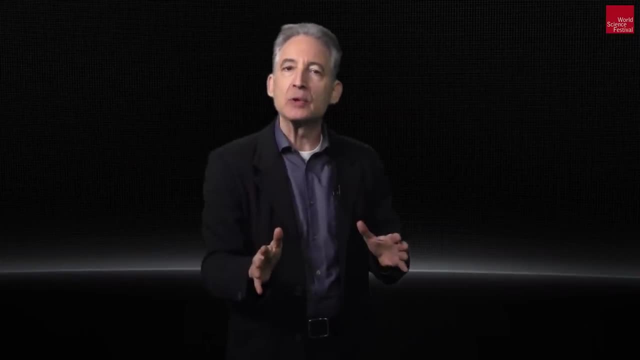 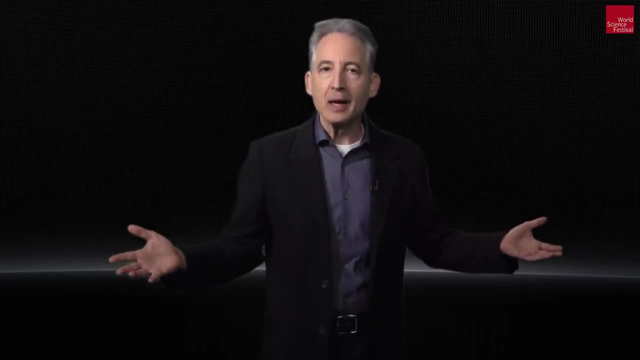 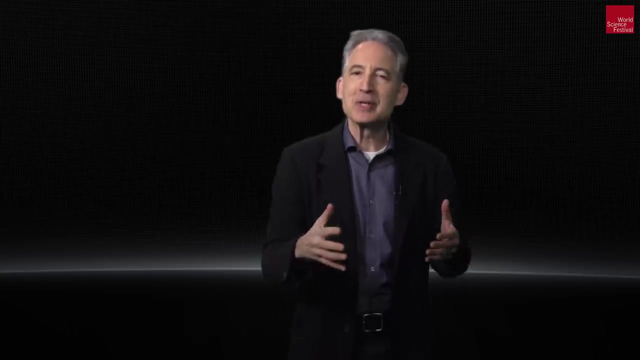 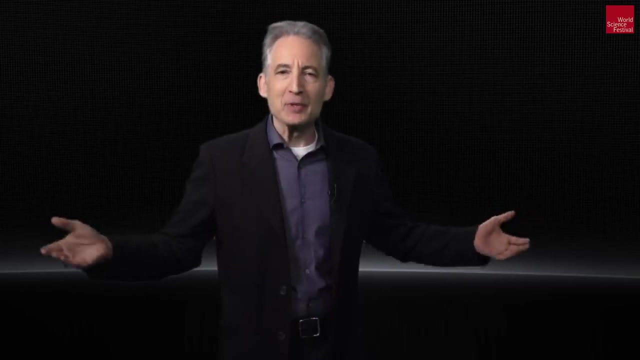 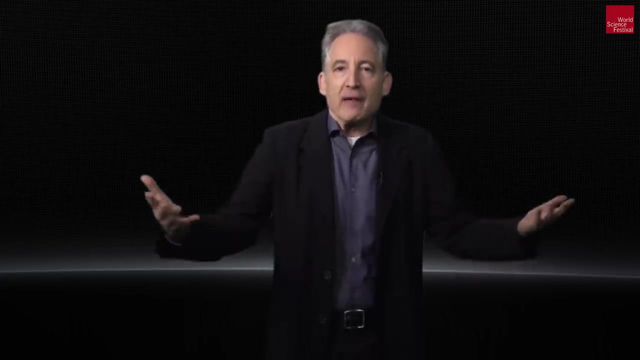 understanding that would not rely on probabilities. And toward this end, Einstein, he worked tirelessly to expose qualities of quantum mechanics that he hoped would be so obviously unacceptable, so counter to any reasonable person's expectation of how the world works, that everyone would have to agree with his view that quantum mechanics was not the final. 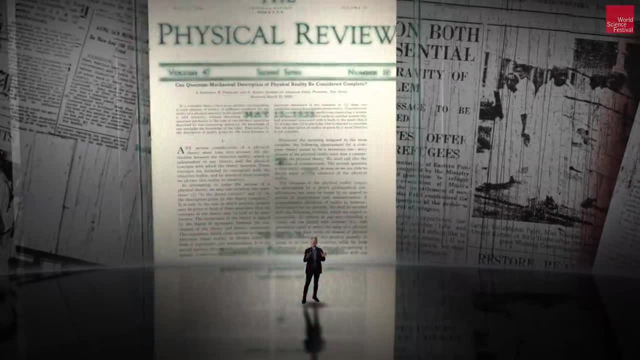 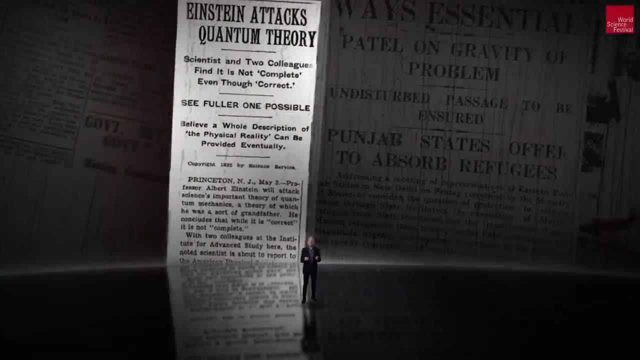 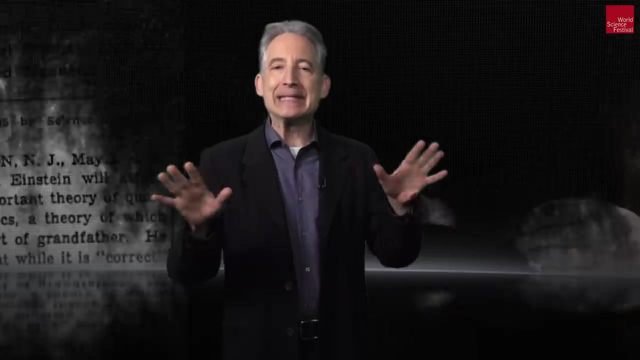 story And in 1935, with two colleagues, Boris Podolsky and Nathan Rosen, Einstein believed he had finally found the ultimate quantum mechanical Achilles heel, with a property inherent to quantum mechanics called quantum entanglement. Briefly put, Einstein and his colleagues found 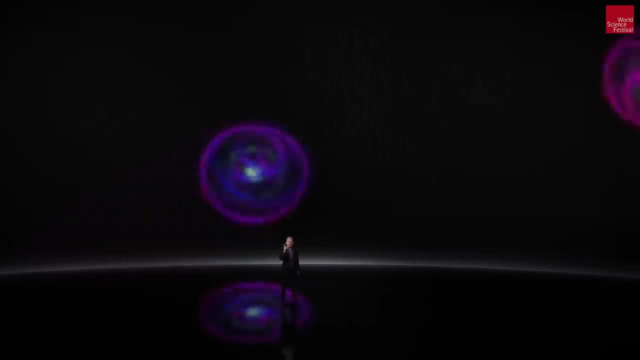 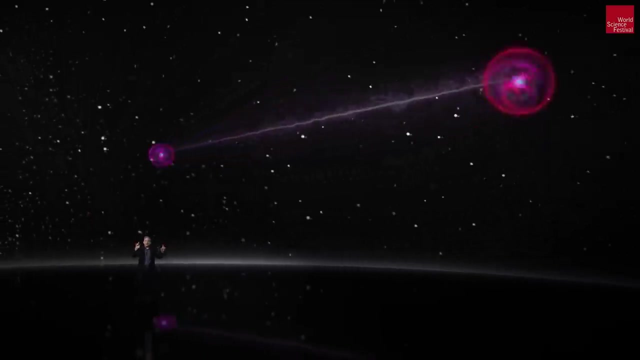 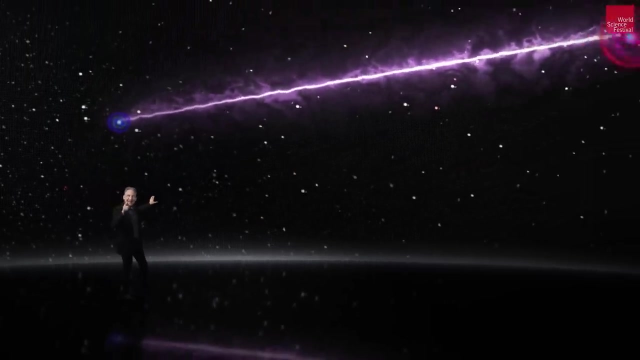 that according to the math of quantum mechanics, if two objects interact and then widely separate, a subsequent measurement presence on one object clearly mistakes the consistent mana of the other objects. But he made the first distinction: the гораздо more changeable the object comes out of, as 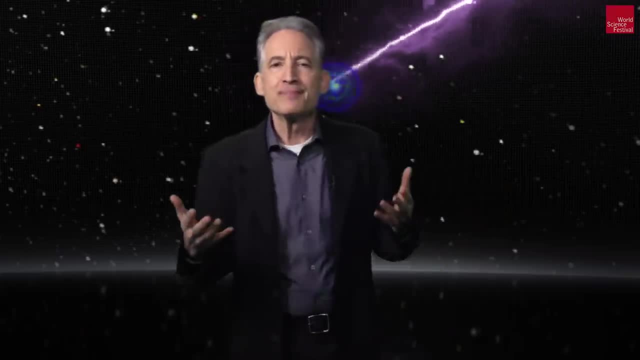 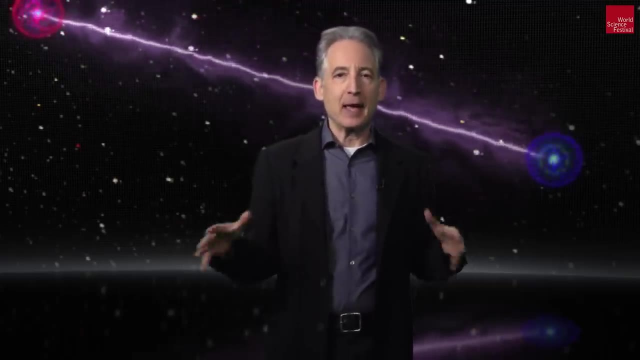 the object shoot, jumps in motion. Rather than mistakenly deserve the likes and dislikes of quantum mechanics, Einstein decided to invent a прочно shrimping technique that allowed isolated Norman feet to quickly distance and emptying it during an intangible of having multiple ophthalmicvedナ. Because we've already supplemented our diaries with bogika and other Noodles here- that it obviously doesn't alienate us from quantum mechanics just as much as anybody else does. However, półsteinines that we 몇 Chunkan in the laboratory have played as highly important. 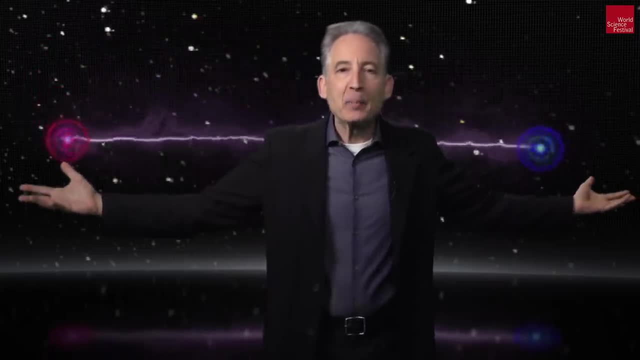 to ourкрäner monopolies than anything else in science and competence, and it was not kind of an attempt to solve the problem, thatford cooperation between players who were simplyianiated. a separate Intuitive belief was that widely separated objects are independent of one another. 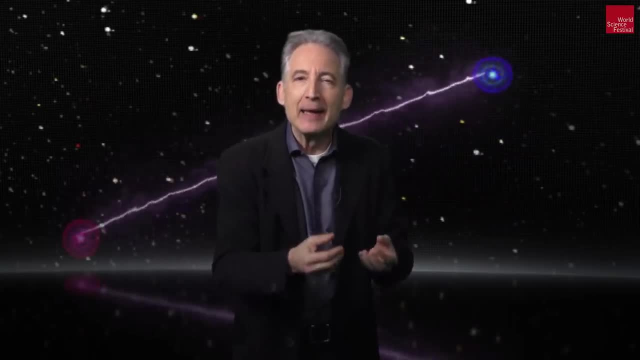 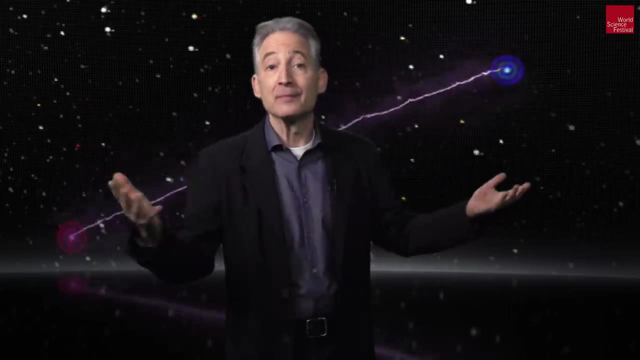 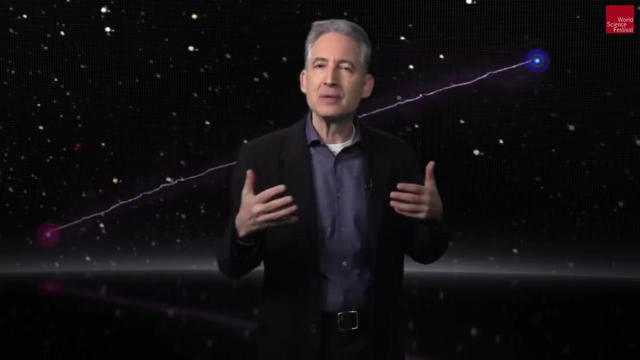 But quantum entanglement seemingly denied that by providing an invisible quantum connection capable of linking the distant objects together or, as the name says, entangling them. Einstein could not accept this quantum view of reality, and so he concluded that something had to give. 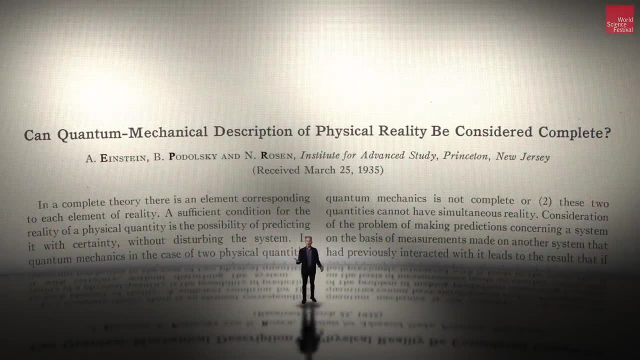 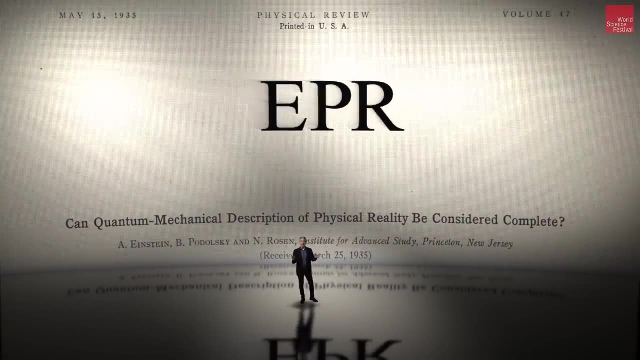 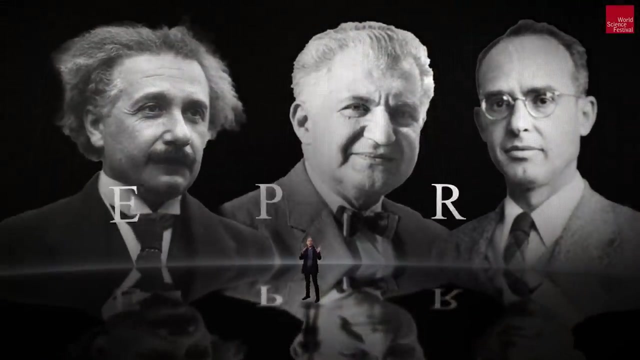 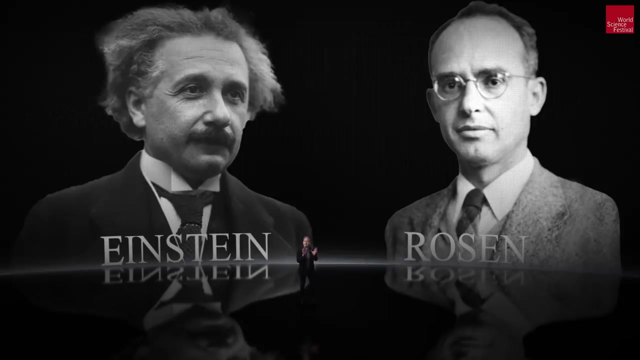 Quantum mechanics could not be the full and final story. That's the upshot of the 1935 so-called EPR paper. Now I want you to note the date on this paper: May 1935.. In July of 1935, Einstein and Rosen published another paper on a seemingly completely different. 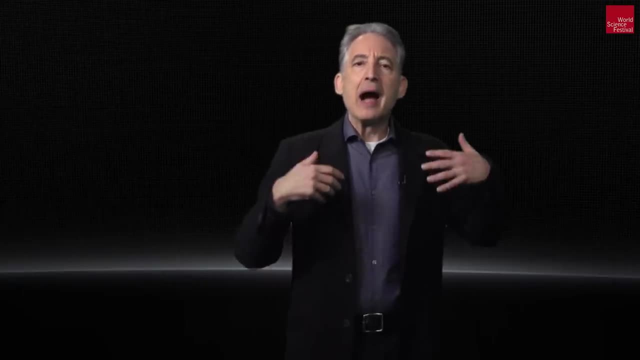 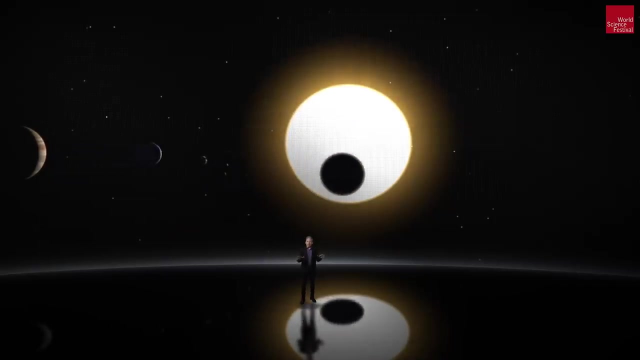 subject: Years earlier, in 1915. Einstein had ripped another rug out from under the Newtonian worldview, showing that Newton's approach to gravity needed to be replaced by his own general theory of relativity, in which the force of gravity, which Newton quantified but never explained, is finally. 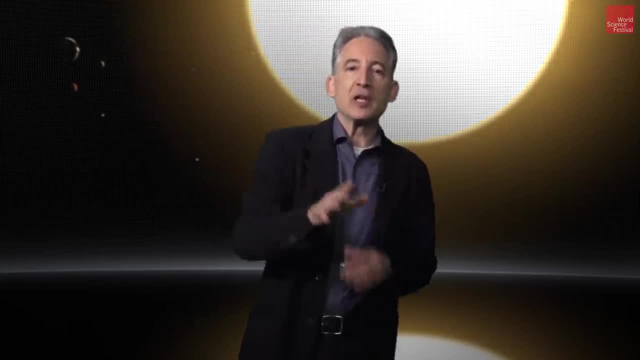 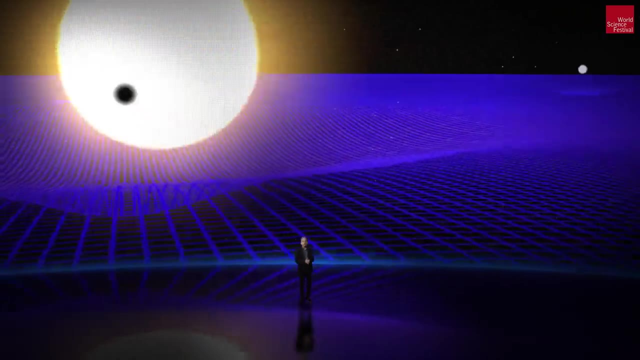 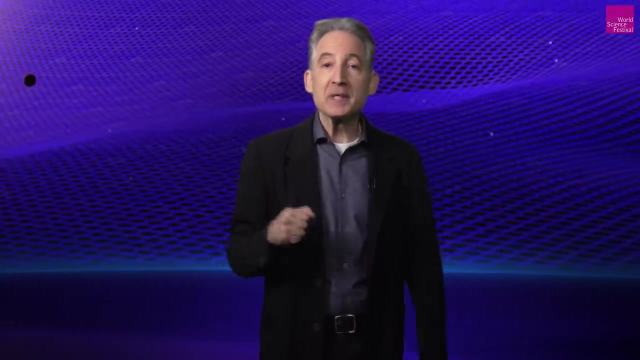 laid bare. To move under the influence of gravity, according to Einstein, is to surf the warps and curves in spacetime. Now, Shortly after Einstein announced this general theory of relativity to the world, a German scientist named Karl Schwarzschild found the first exact solution to Einstein's new 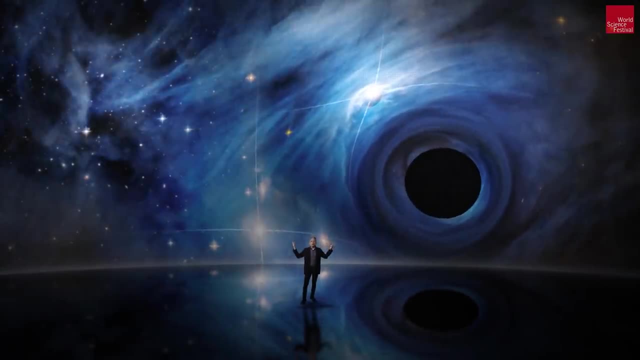 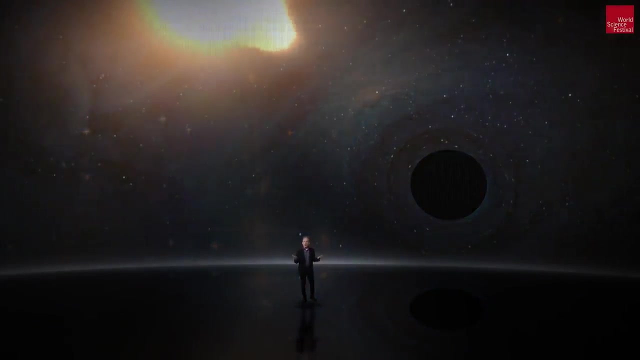 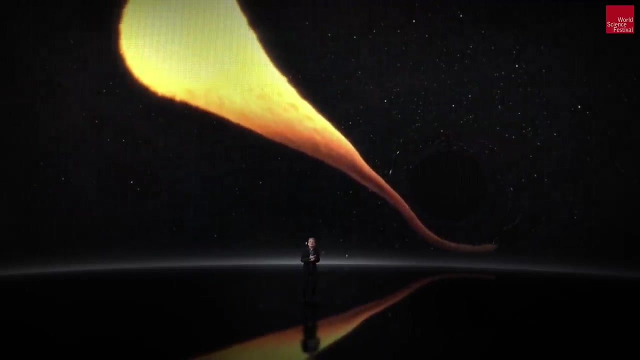 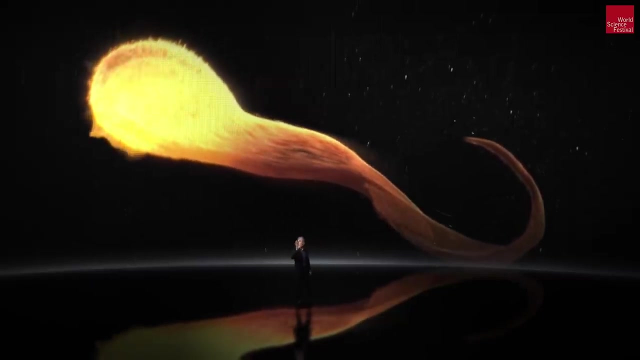 equation showing how a spherical body, like a star, warps its environment And within that solution is a startling realization. If a spherical body is crushed to a small enough size, the spacetime curvature is so extreme That a kind of point of no return forms if anything crosses this so-called event horizon. 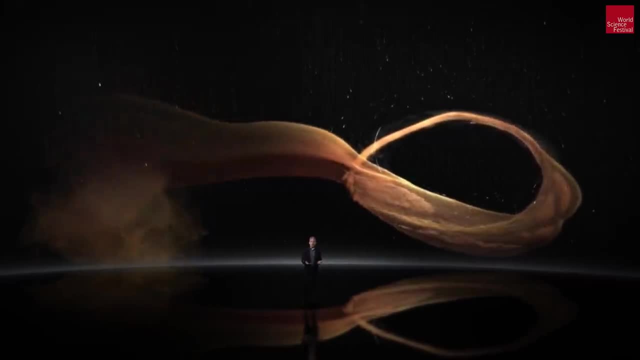 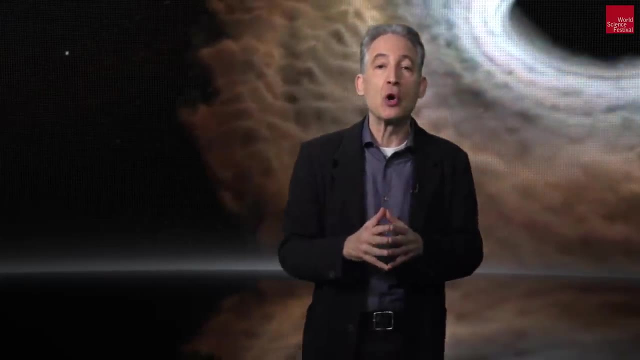 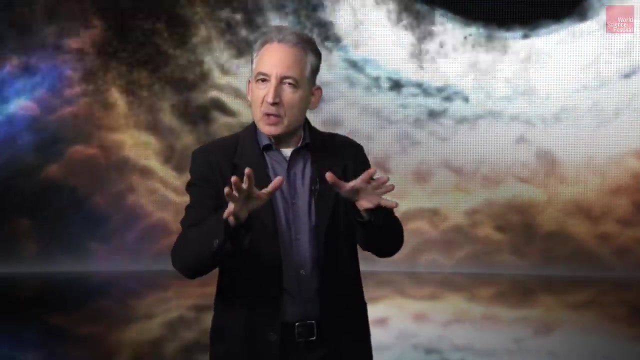 it's impossible to escape the gravitational pull. Even a beam of light can't escape, so the region appears dark. We have what in modern parlance is called a black hole. In his 1935 paper with Rosen, Einstein wasn't actually thinking about black holes, but it. 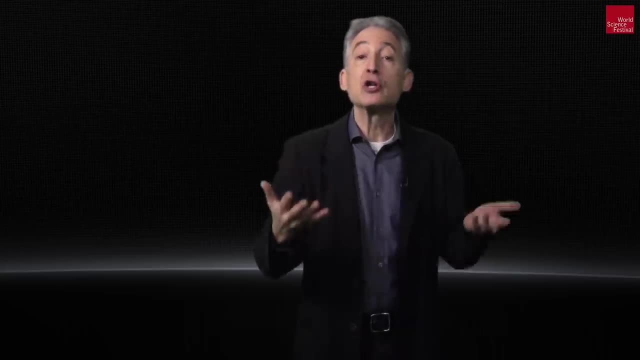 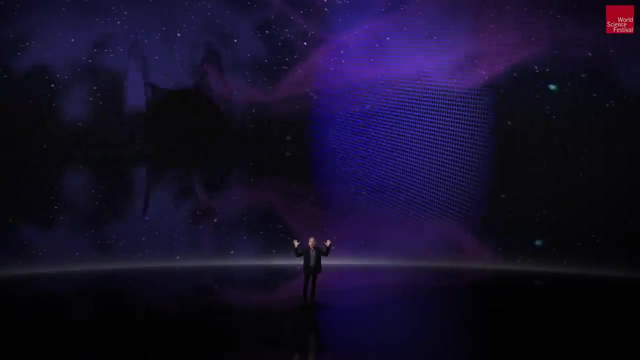 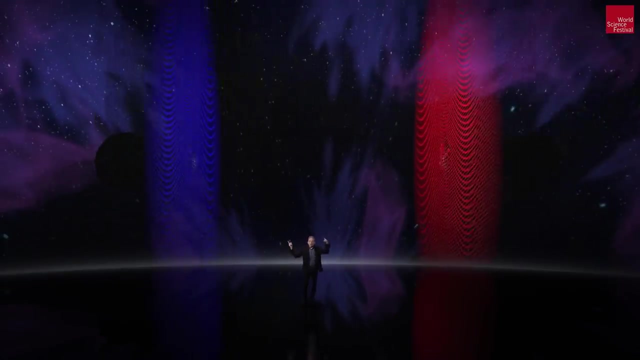 turns out, Black holes provide the right language for the modern interpretation of their result, which is this: Einstein and Rosen found that two black holes can be joined together in spacetime, connecting one region of the universe to another through a kind of bridge. 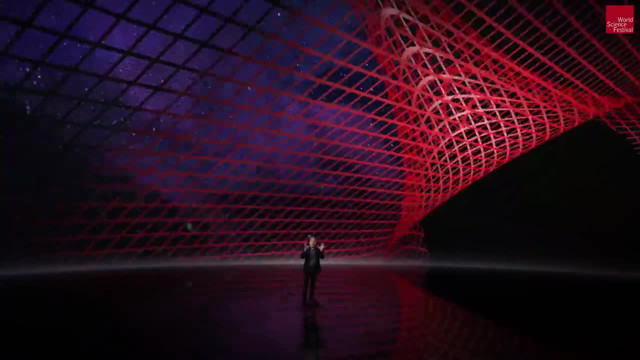 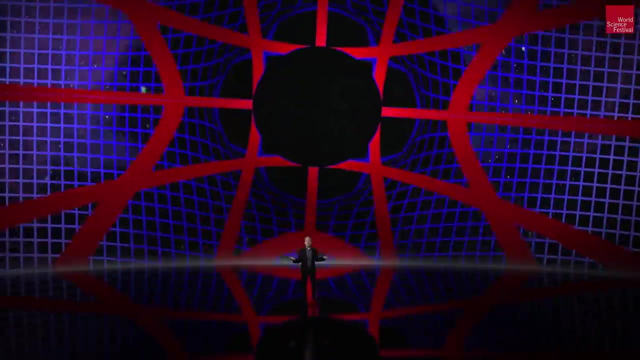 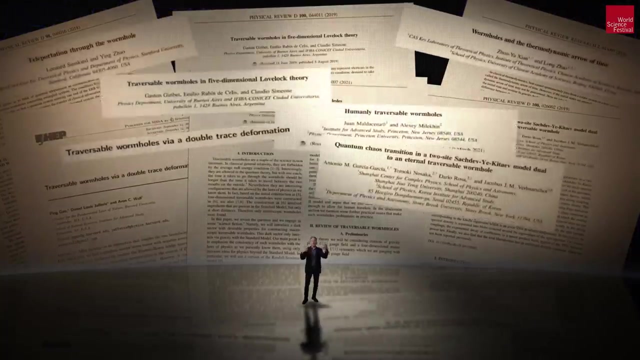 What we now call an Einstein-Rosen bridge, or perhaps, in more popular terminology, a wormhole. Now, These wormholes have been a staple of science fiction, but they're also an arena of scientific study, Although they are still surely fully hypothetical. theoretical physicists have learned a great 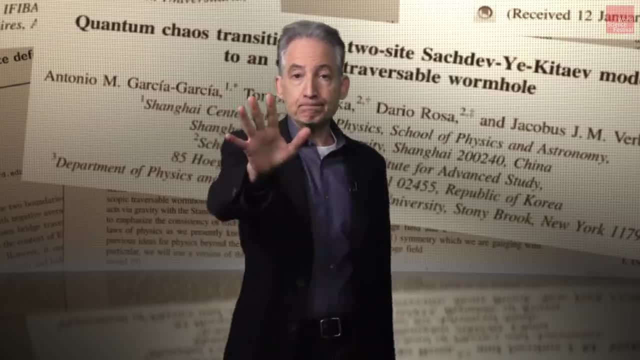 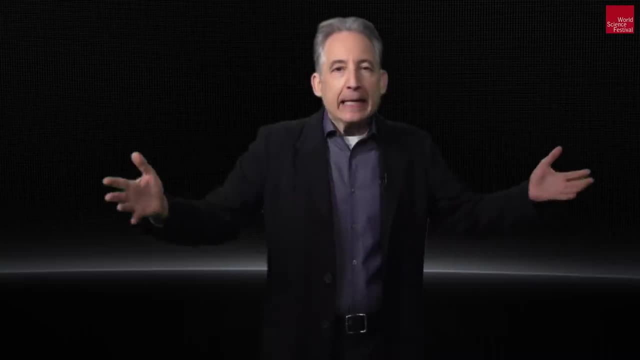 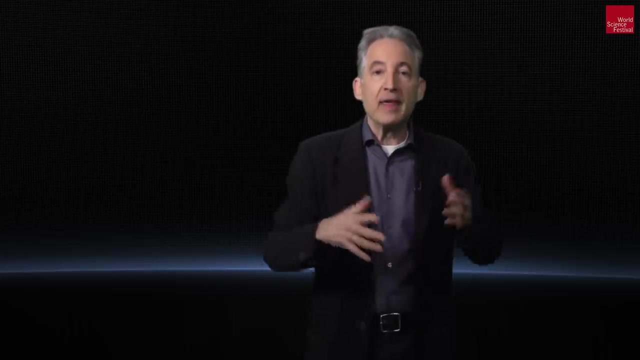 deal about wormholes in the intervening decades. But here is the thing: Were you to have asked any of those researchers if there was any connection between wormholes and Einstein's other 1935 paper, the one on quantum entanglement, They would have said no. 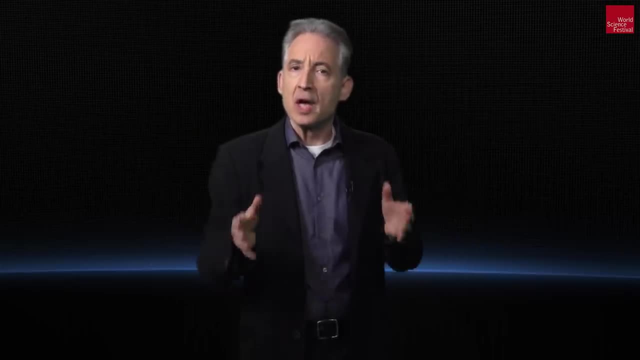 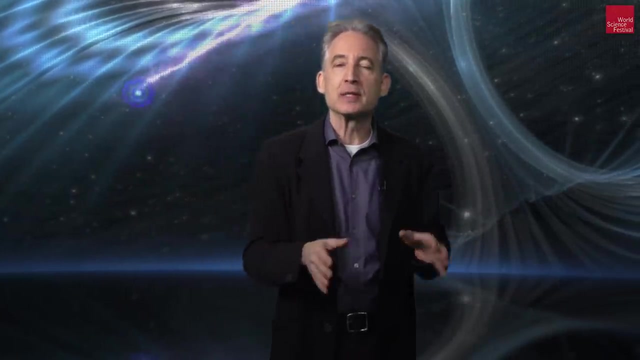 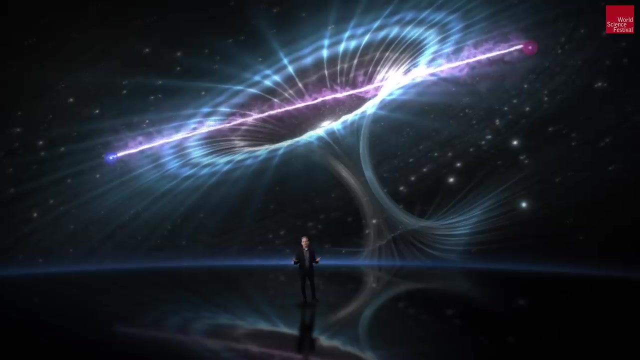 At least until very recently, as a surprising new connection has been proposed, a proposal with potentially far-reaching consequences, not just for black holes, but even for the very structure of space and time themselves. Tonight, we are honored to have three guests who will lead us through the wonderful worlds. 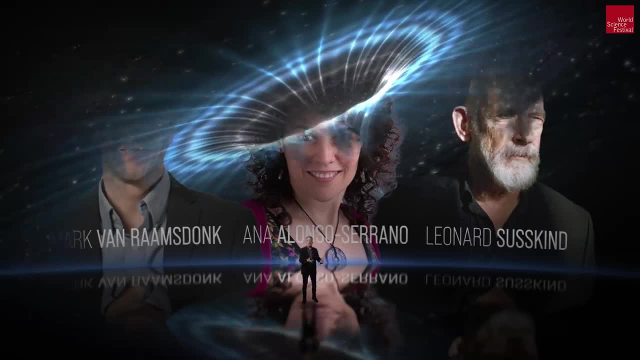 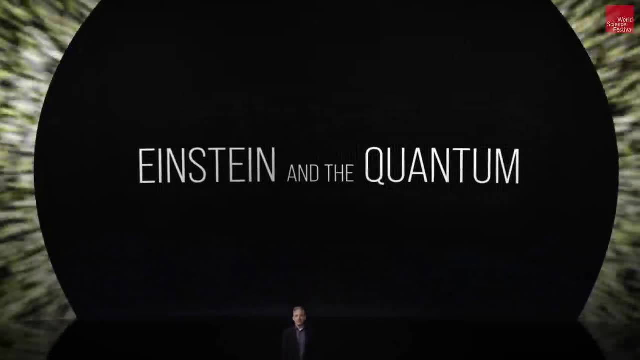 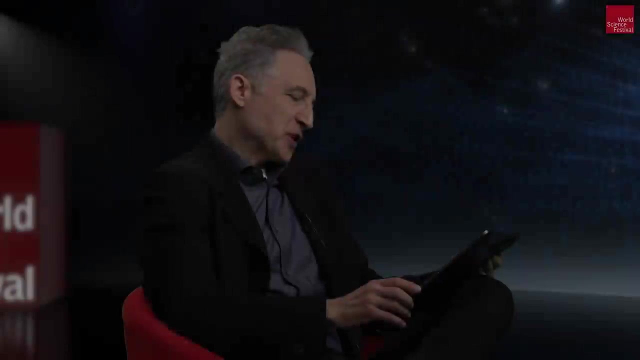 of general relativity, quantum mechanics, black holes, entanglement and some of the cutting-edge developments that may link these ideas together. Our first guest is Mark von Ramsdank, who is a professor of physics at the University of British Columbia. 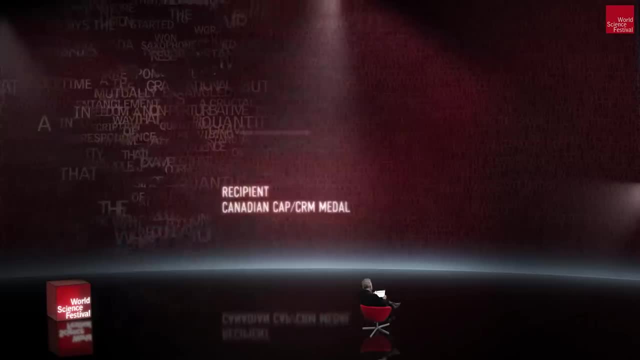 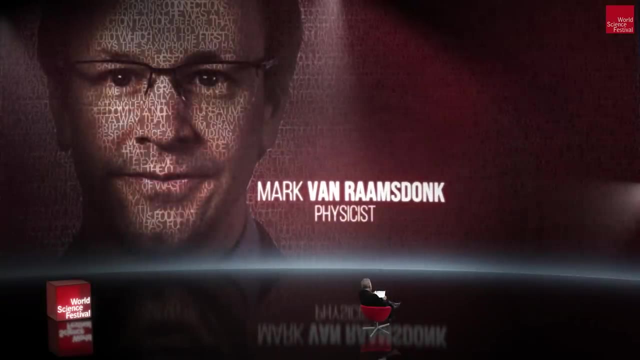 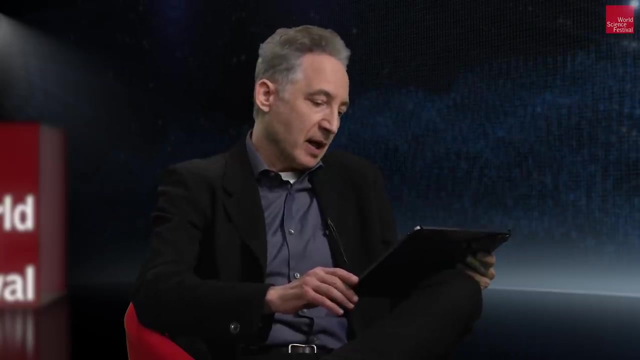 He was a Canada Research Chair, a Sloan Foundation Fellow, is currently a Simons Investigator and is a recipient of the Canadian CAPCRM Medal in Theoretical and Mathematical Physics. He joins us now from Vancouver. Welcome Mark. Next we have Ana Alonso Serrano, a post-doctoral researcher at the Max Planck Institute for 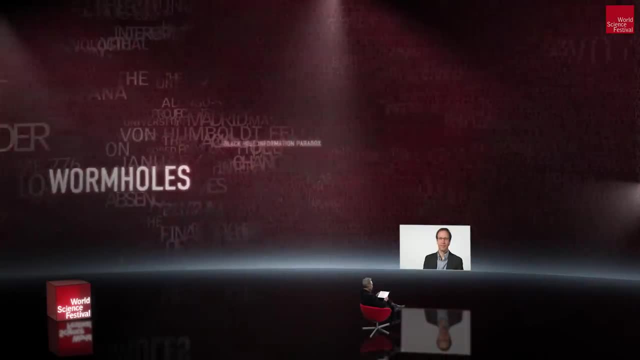 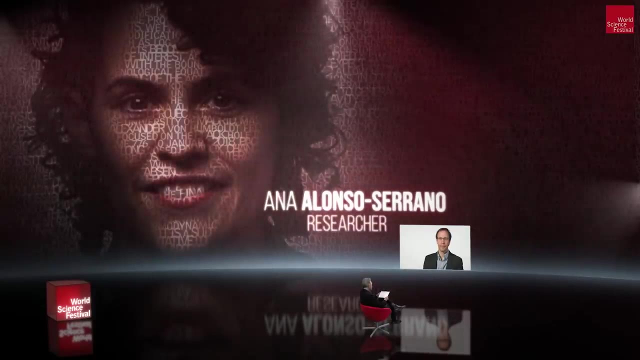 Gravitational Physics. Her work lies at the interface between gravitational theory and quantum theory, including aspects of the black hole, information paradox, thermodynamics of space-time, as well as notions of entropy, quantum cosmology, quantum field theory and wormholes. 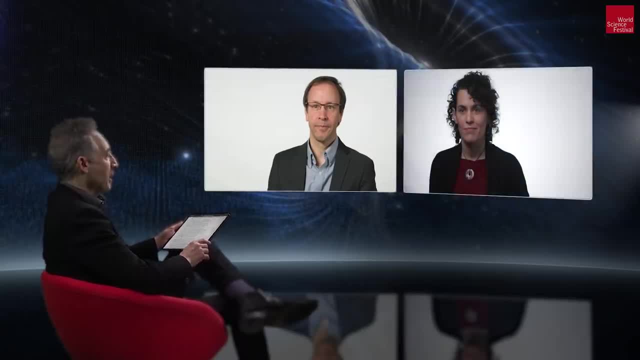 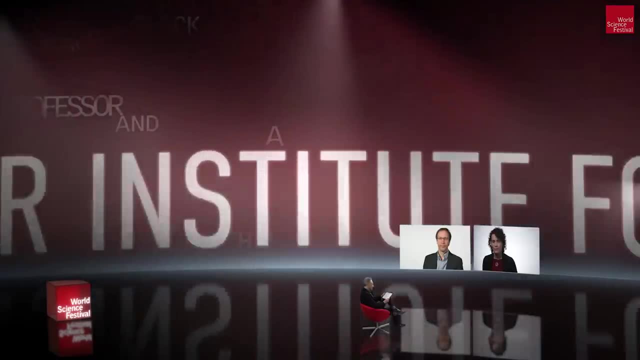 She joins us from Berlin. Welcome, Ana. And finally, London. We have Leonard Susskind, the Felix Bloch Professor of Theoretical Physics at Stanford University. He's a member of the National Academy of Sciences, the American Academy of Arts and Sciences. 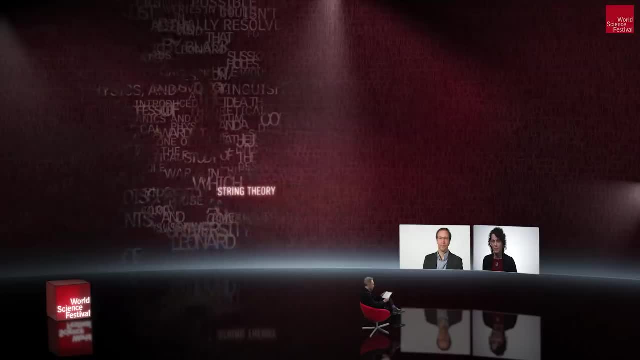 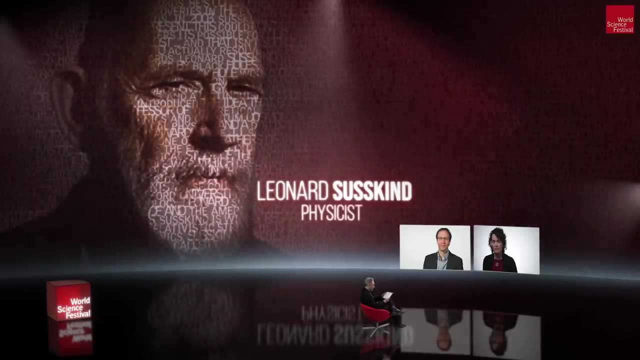 an associate member of the Faculty of Canada's Perimeter Institute for Theoretical Physics and a distinguished professor at the Korea Institute for Advanced Studies. Susskind is one of the founders of string theory and is widely regarded as one of the most influential physicists of our time. 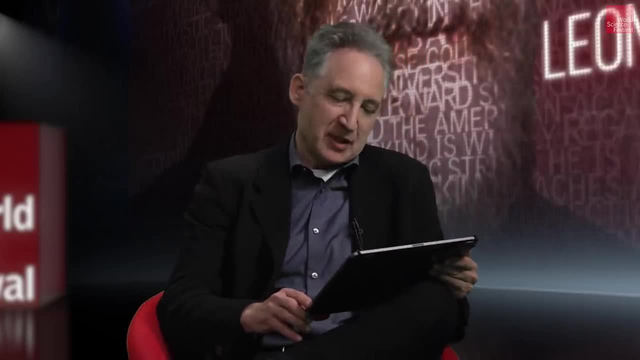 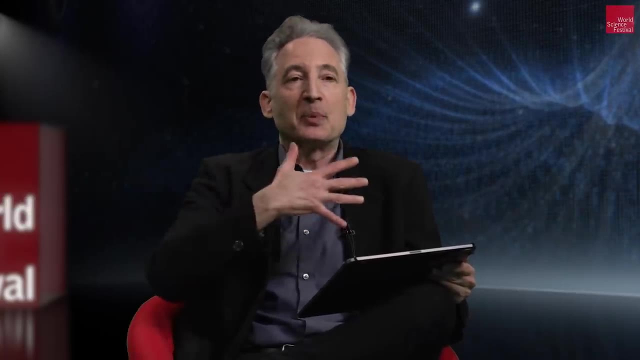 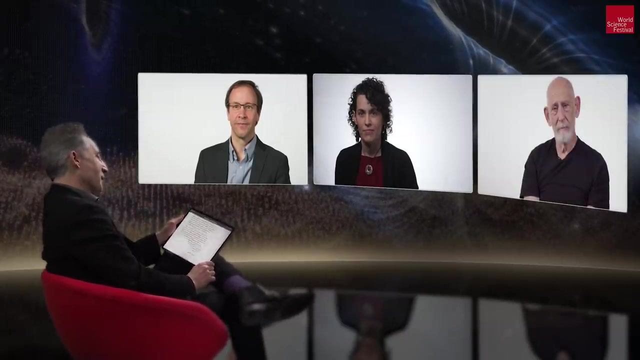 I could go on, I could go on, But suffice it to say that without Susskind's profound contributions, many of the key ideas that we will be discussing here tonight, simply put, they would not be known. He joins us from his home in Stanford, California. 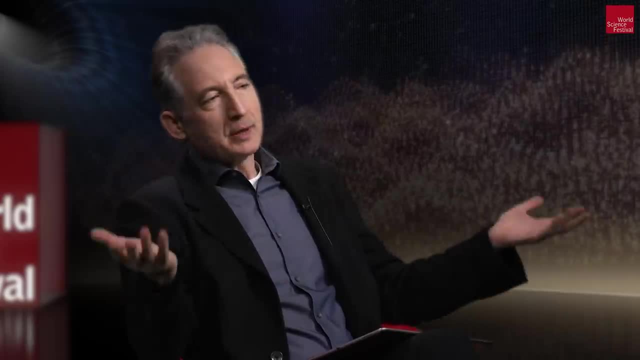 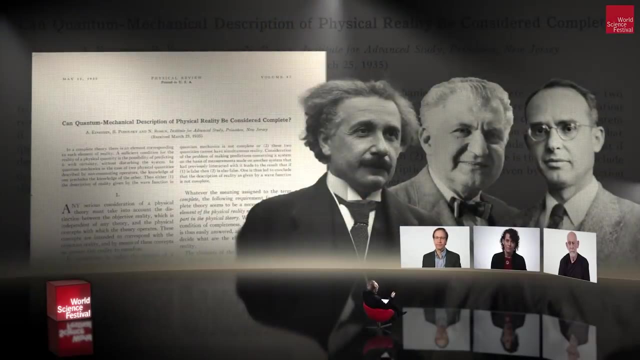 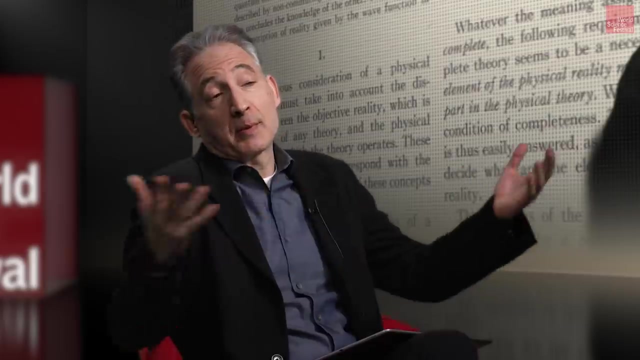 Welcome, Lenny, and welcome to you all. Let's jump right in and discuss Einstein's 1935 paper on quantum entanglement. And so, Mark, what do you think? What motivated Einstein to write this paper? Was he trying to advance our understanding of quantum mechanics? or perhaps was he trying? 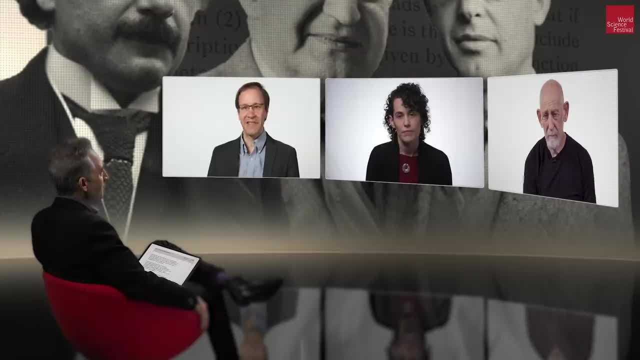 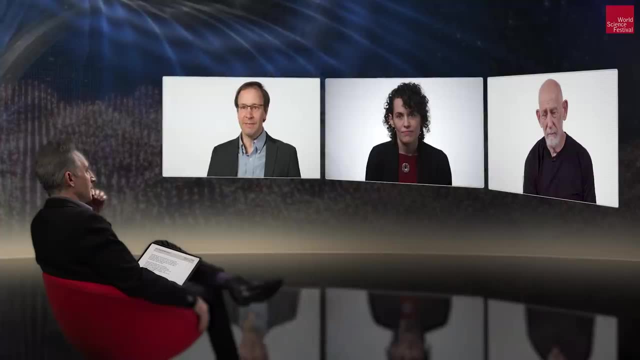 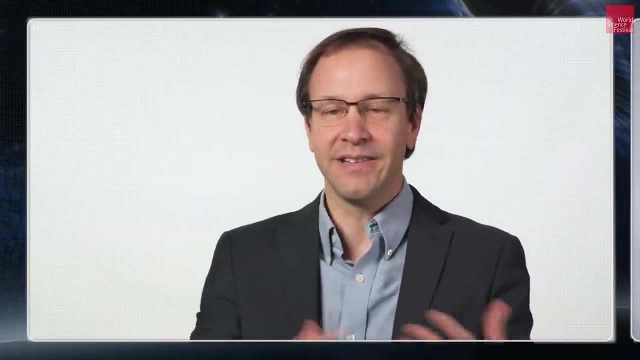 to kind of undercut it entirely. Yeah, I mean, I was looking over that paper again last night and it's really clear that he's uncomfortable with some aspects of quantum mechanics. He's trying to show, in a sense, that the current understanding of quantum mechanics 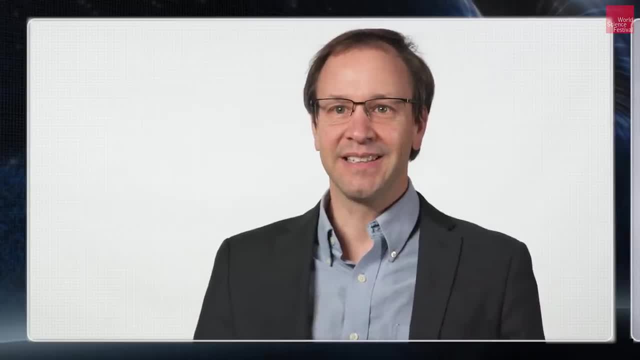 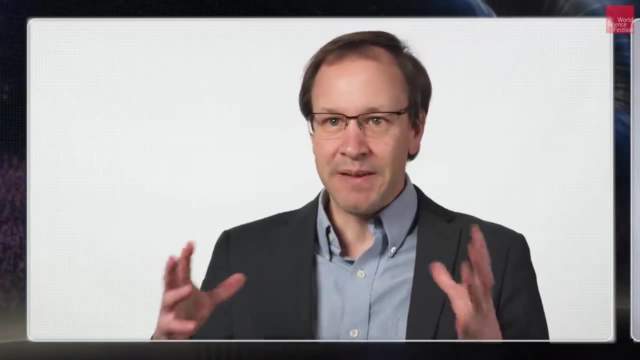 can't be complete. He, with his colleagues, feels that. He feels that maybe there's something wrong with it and it's like they've found the thing that will maybe prove that there's got to be something more there, that maybe there's. 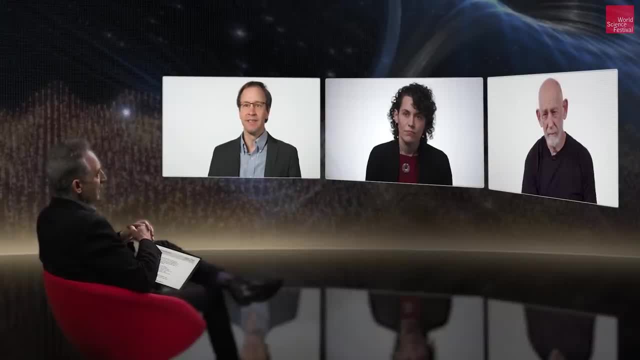 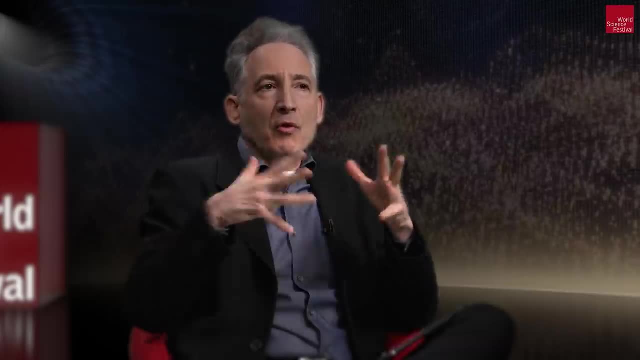 some extra information in addition to the wave function? Yeah, So, Lenny, you know. there's this interesting historical fact that Schrodinger, long before the 1935 paper, he said something like- I don't have the exact words, but he said something. 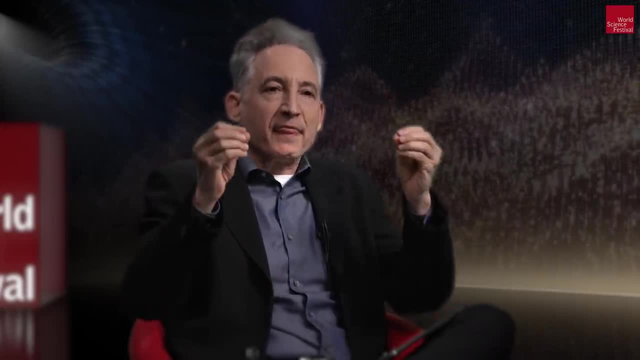 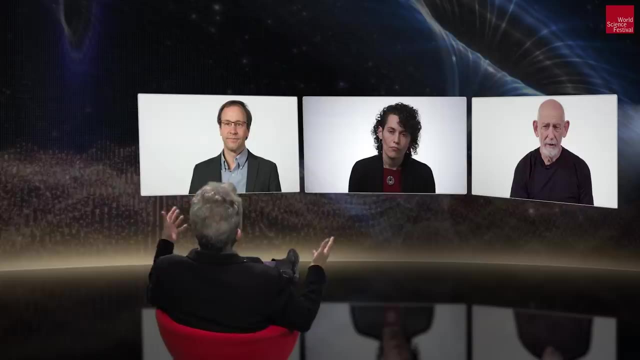 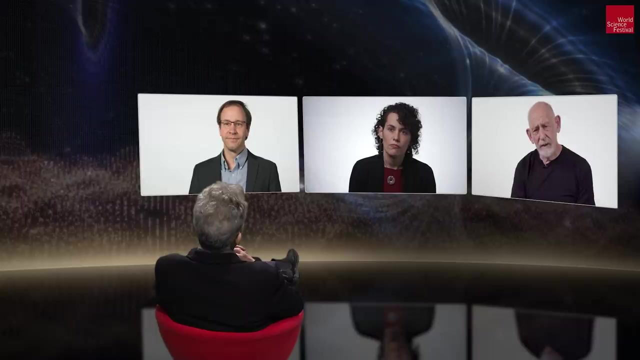 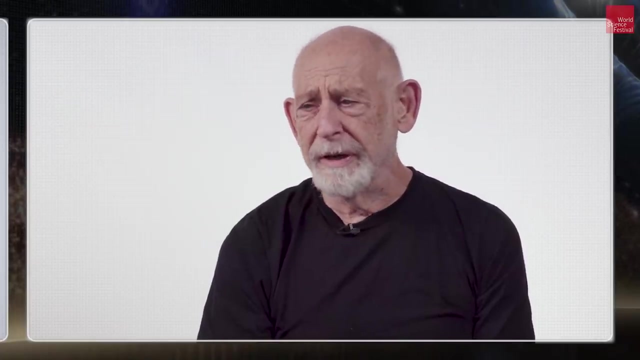 like He said, entanglement is not one, but the feature of quantum mechanics that distinguishes it from a classical worldview. Do you agree with that assessment of entanglement? Yes, I think that's fair. I think that's fair to say that entanglement, it's certainly the most peculiar and different. 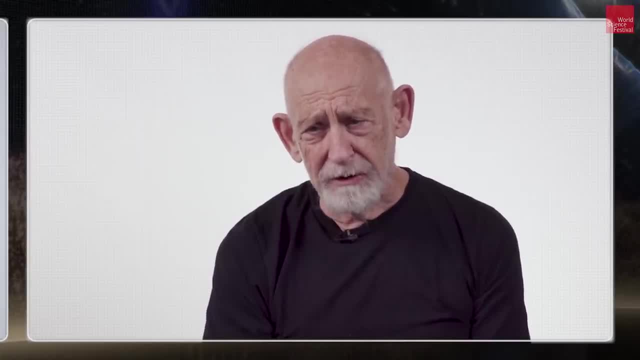 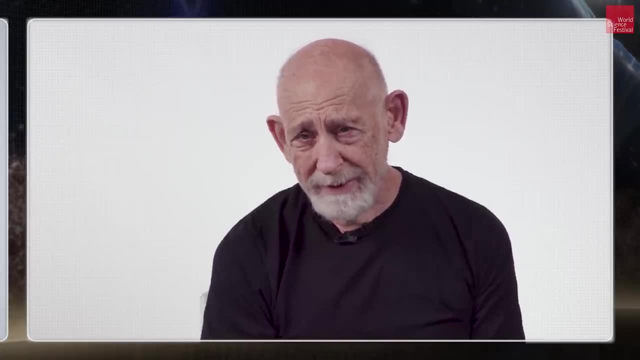 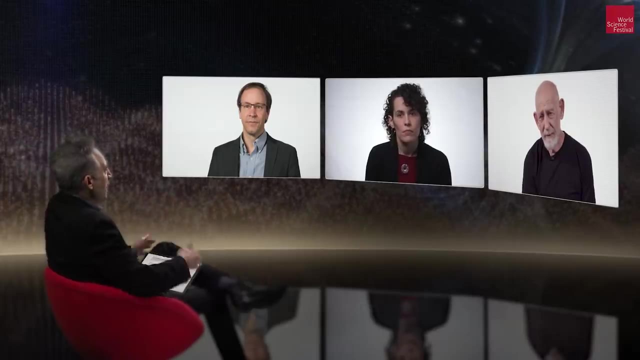 thing about quantum mechanics. I think it's fair to say It's the central core of the difference between classical physics and quantum mechanics. So, Ana, I'm just curious because I think, of all the folks participating in this conversation, I think you and I have perhaps the greatest age differential. 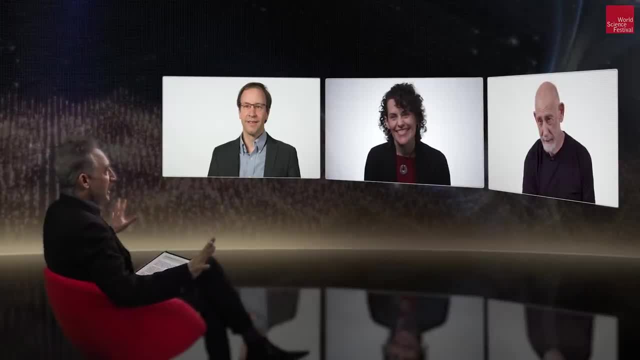 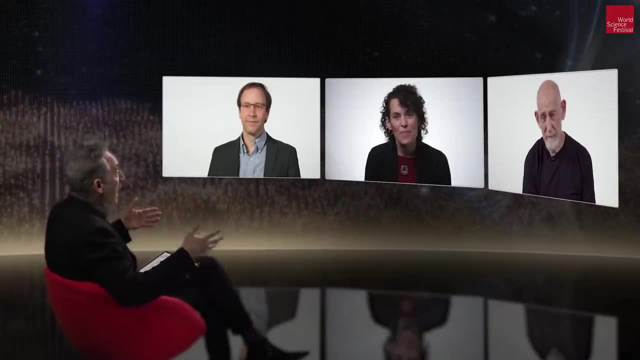 When I was an undergraduate, entanglement never came up. It wasn't in the lecture and it was a good class, I went to a good place. It wasn't in the textbook. How about for you? Did you learn entanglement in your first course in quantum mechanics? 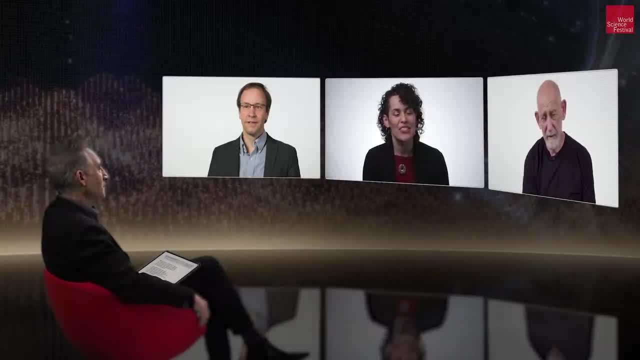 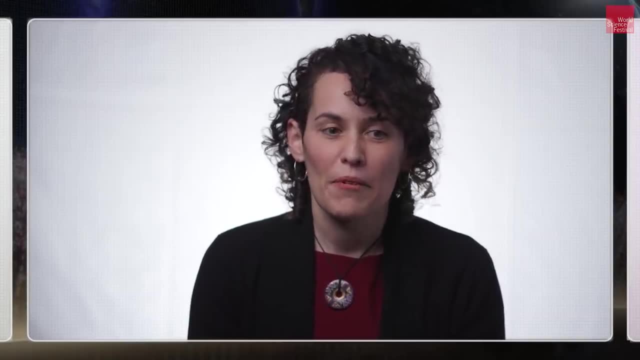 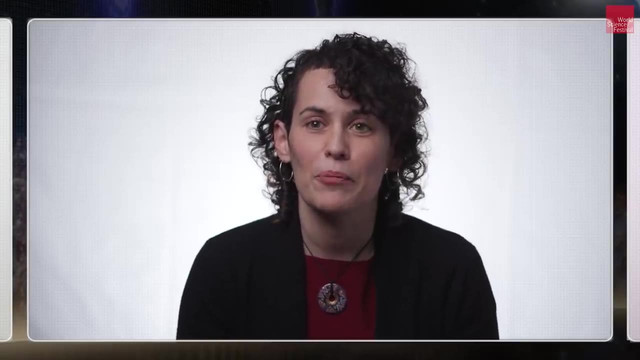 Yeah, that's a great question, because it was something it surprised me a lot. In fact, not really at the beginning. It was something that appeared pretty late for what it is, as was said before, that being the most peculiar and characteristic point was not so much mentioned. 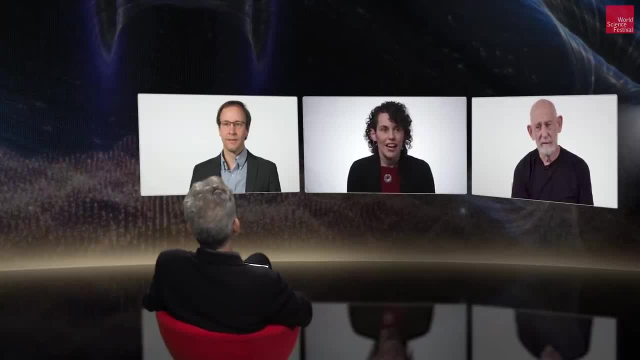 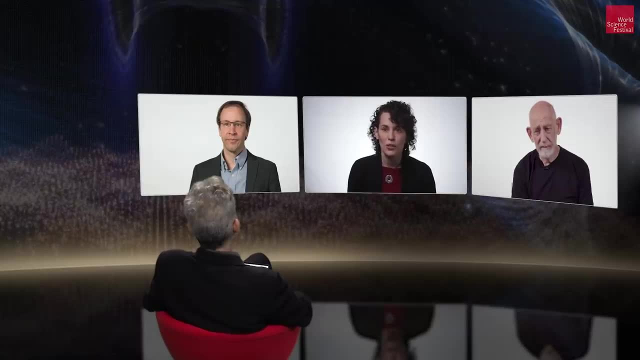 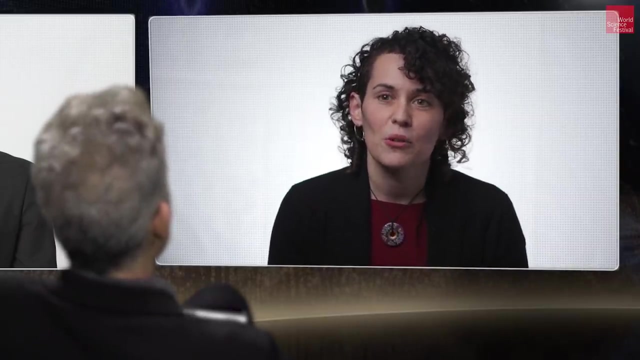 And I was also surprised, Like neither any. Oh yeah, Yeah, I think that the history of how quantum mechanics was developed and this point that was raised by Einstein and the different ideas about interpretation of quantum mechanics- it's not something that you are teaching right now, neither in a bachelor degree. 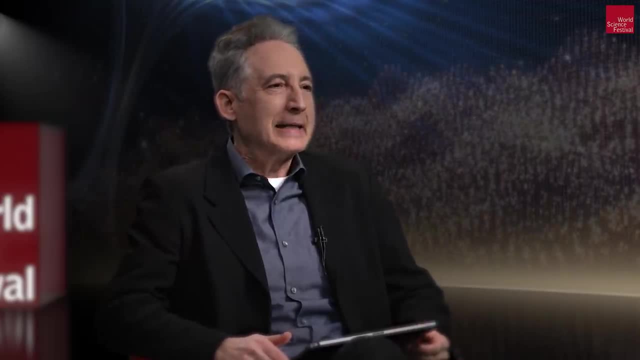 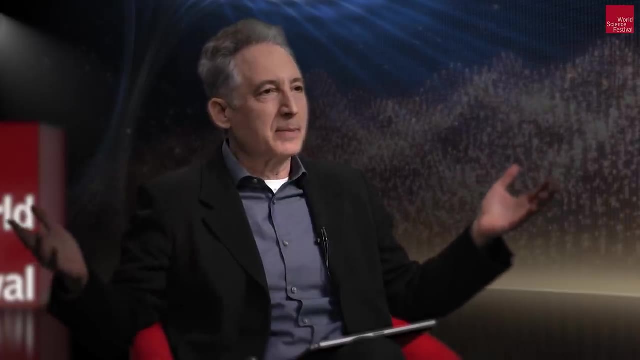 So yeah. So, Marc, we've said a few words about entanglement. We haven't actually said what it is, So can you just give us your best description of what quantum entanglement is actually all about? Yeah, absolutely. 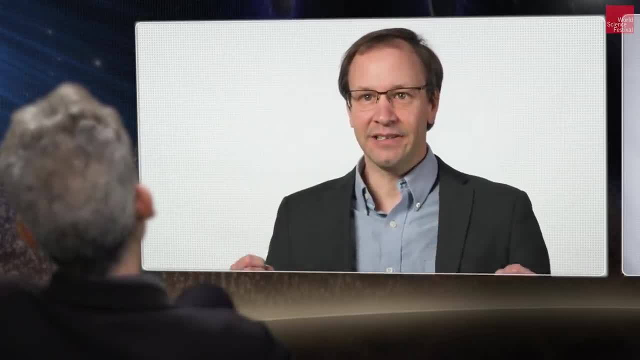 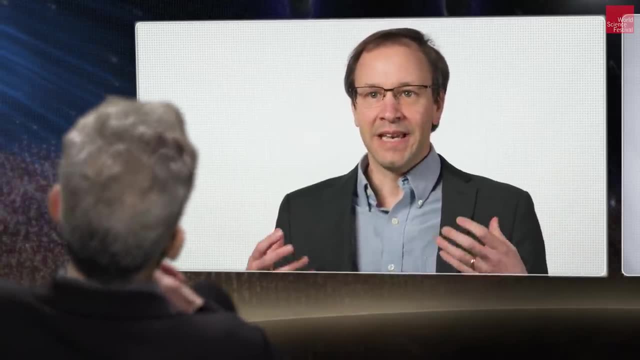 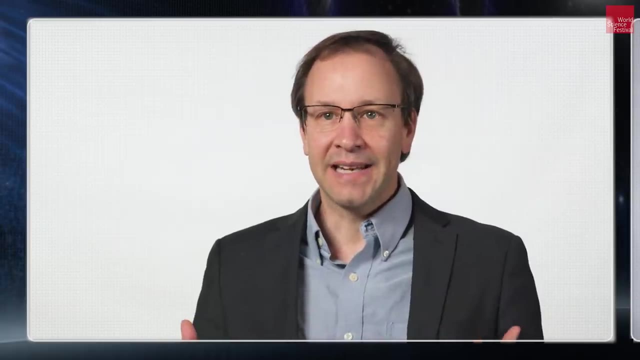 So I think the underlying idea here is the quantum superposition idea. I would say that in some sense is the core of quantum mechanics, that if you have a physical system and it can exist in two different configurations, then quantum mechanics says that it could. 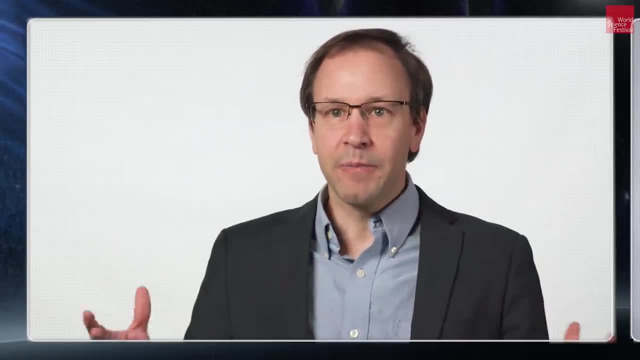 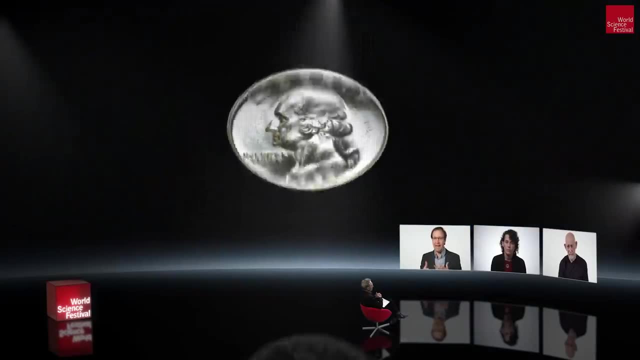 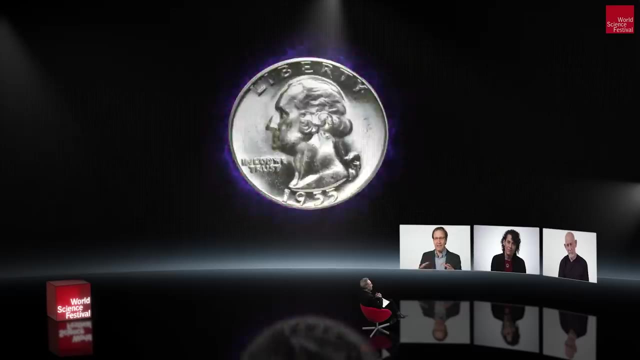 also exist in what we call quantum superpositions of those configurations. So let's say I had a classical object like a coin. It could. You flip it, It could be heads, It could be tails, And in quantum mechanics what we say is that, well, it could also be in all of these other. 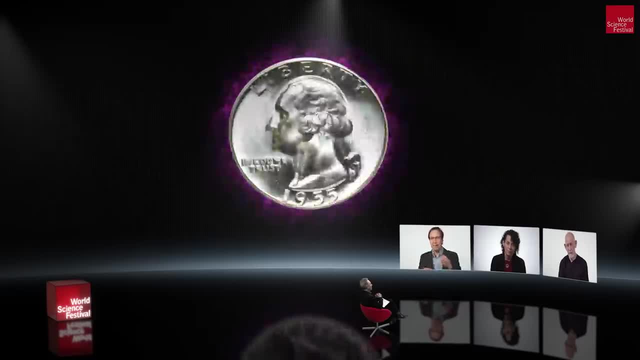 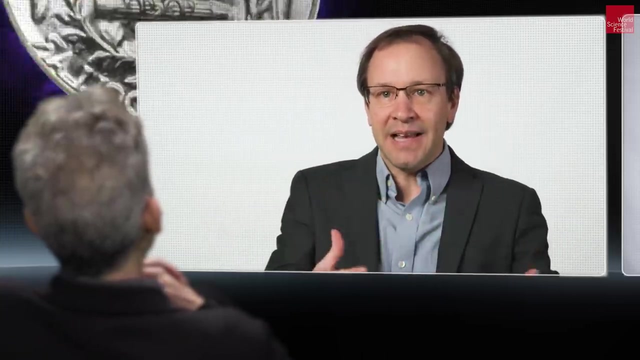 configurations that are part heads, part tails. They don't have a definite result until you go and you interact with that system and measure it to see if it's heads, if it's tails. So that's sort of the basis And then with quantum entanglement it's just applying that to systems that have multiple. 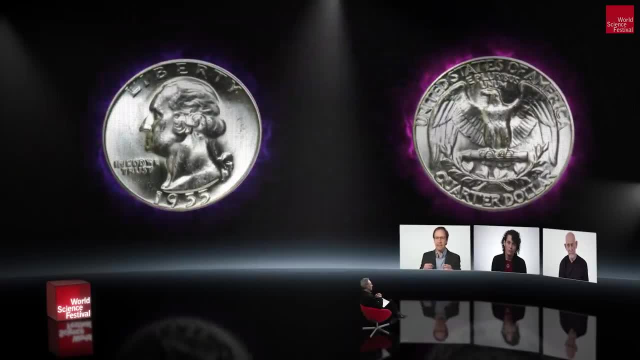 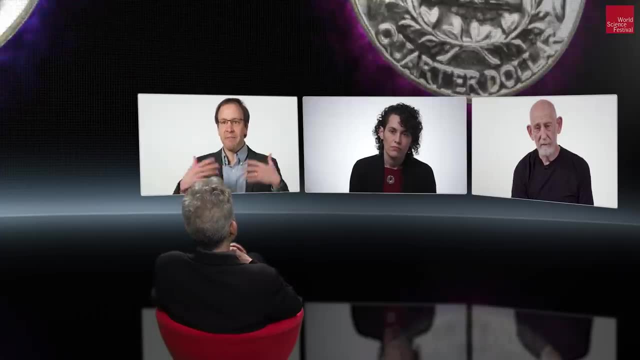 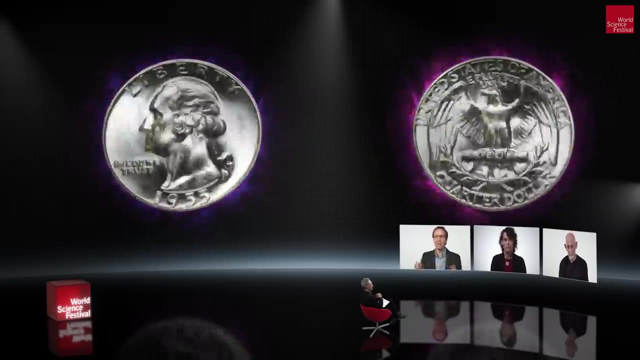 parts. Yeah, So you look at two of these coins now And if you flip both of those, then in quantum mechanics you could have weird combinations like partly heads tails, partly tails heads. So there's all these different combinations. 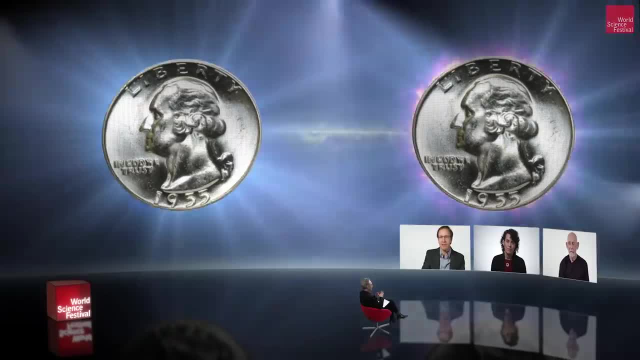 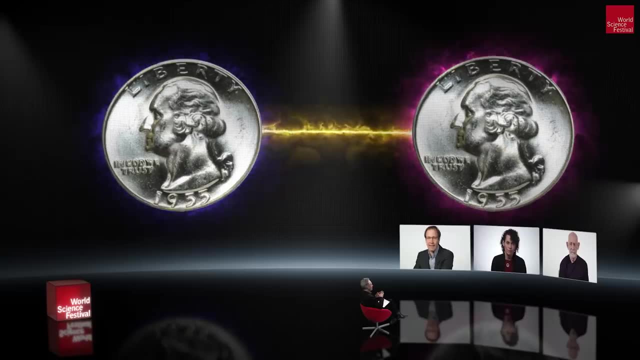 And the idea with quantum entanglement. if you go in and measure that, you go and look at what are the coins saying, then if you find heads for the first one, then you're definitely going to find heads for the second one. 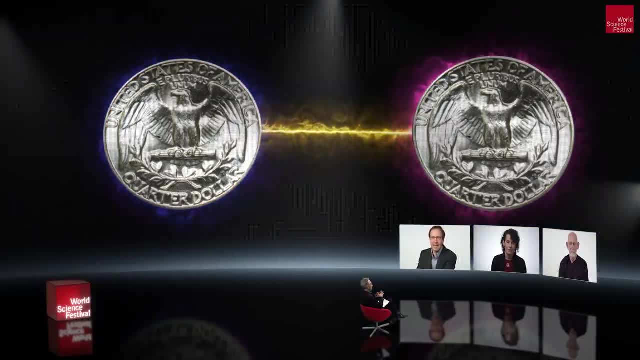 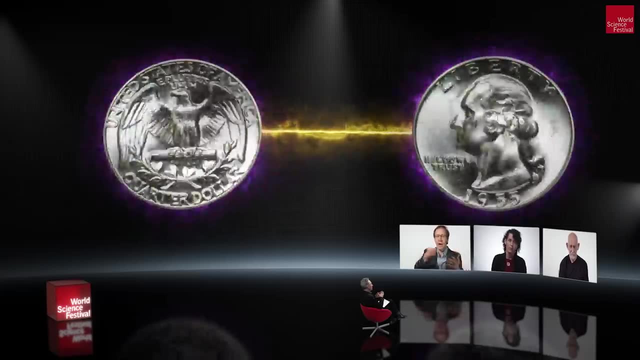 If you find tails for the first one, you'll definitely find tails. You'll definitely find tails. Yeah, definitely find tails for the second one. So it's this correlation between the two states, even though either one of those things is uncertain. 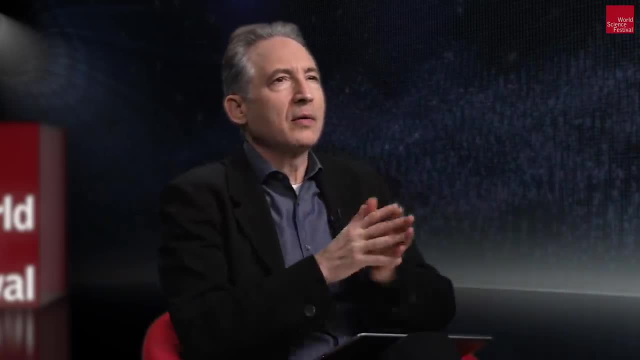 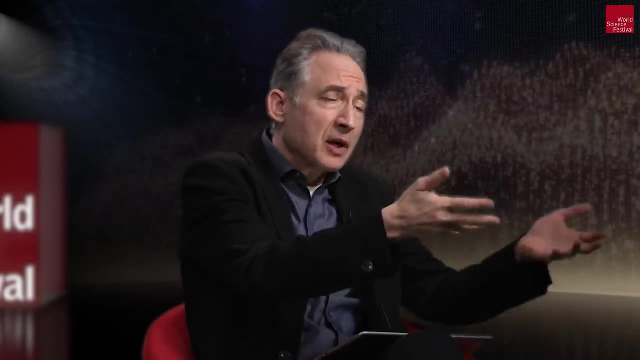 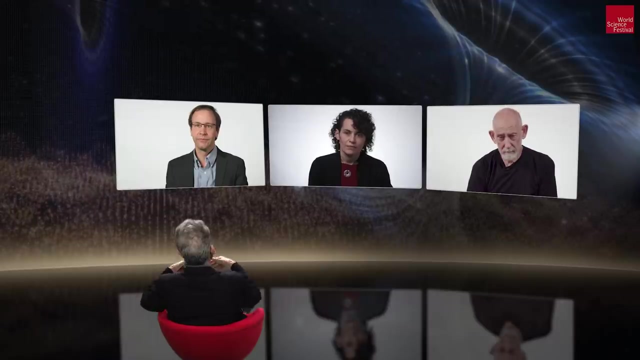 ED HARRISON, Right, right, And because these correlations they hold, regardless of how far apart the objects may be. Einstein famously described this as spooky, as spooky action at a distance. right, You do a measurement on one of these coins or one of these particles and it has a kind 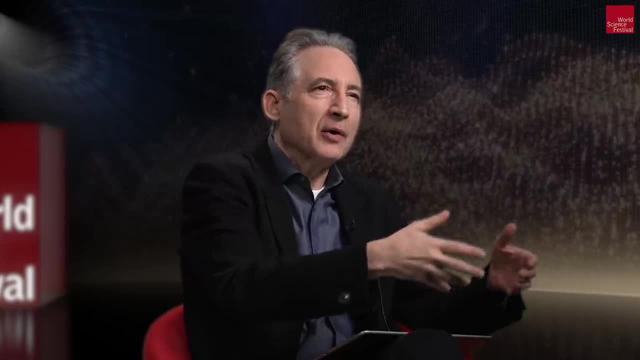 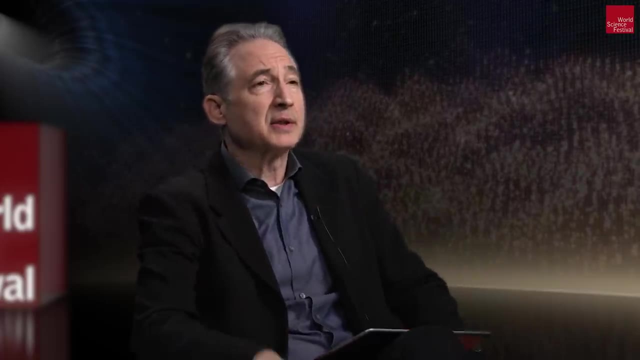 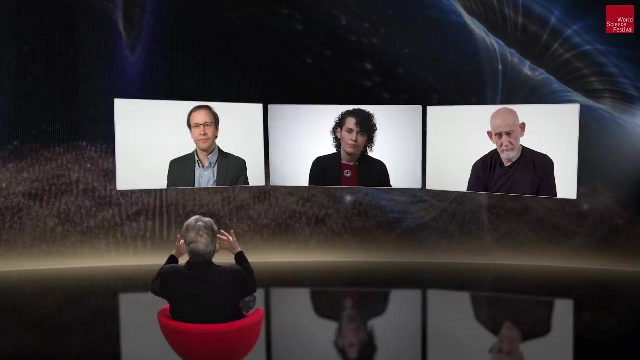 of instantaneous impact on the partner. You measure one coin, you find heads. The other one is definitely heads or definitely tails, whatever the configuration of the objects may be. But Einstein himself seemed to focus on another aspect, a related aspect of quantum entanglement. 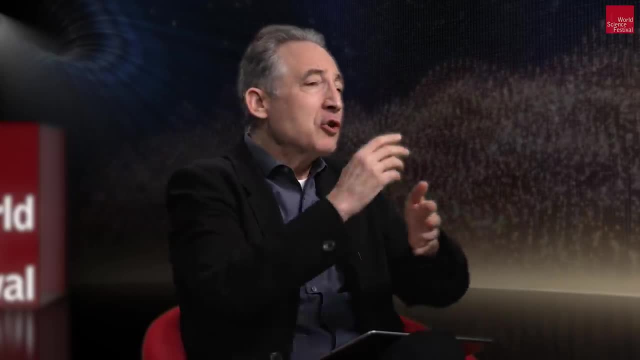 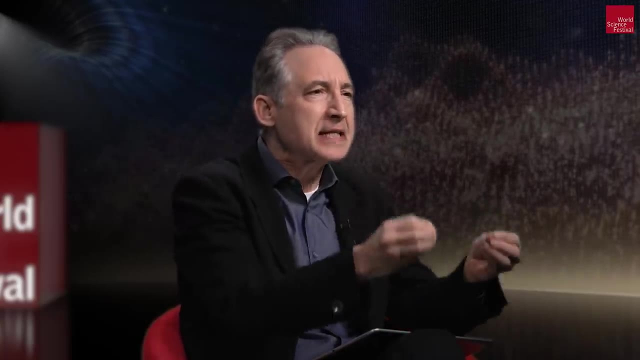 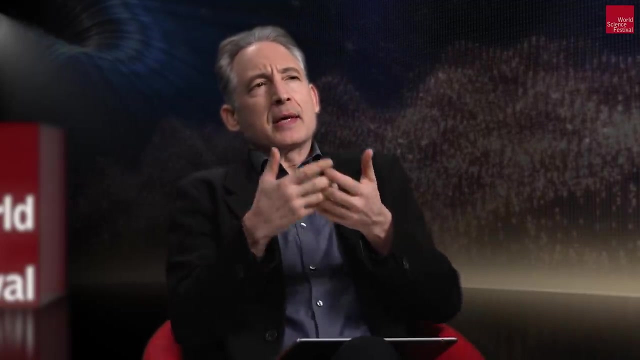 which is this: In composite systems, you can know everything that there is to know about that composite system. You cannot know anything specific about the individual pieces. Now, Lenny, is that a part of entanglement that you think is really more at the essence? 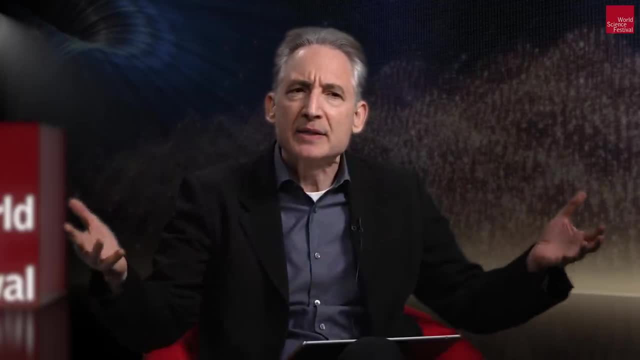 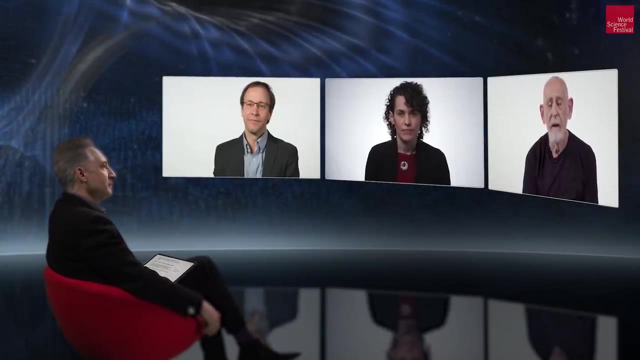 of quantum entanglement than spooky action at a distance. LENNY GRIFFIN. Yes, that's exactly the way I think about entanglement and what's weird about it that you have two systems, my two hands. You know, God gave us thumbs. 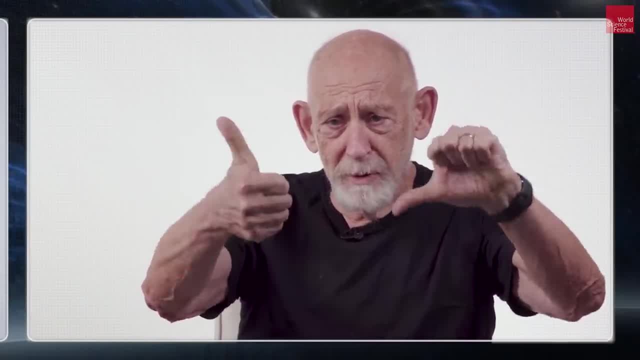 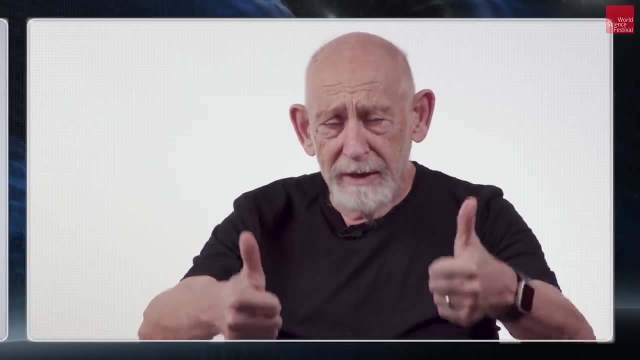 What a lucky thing. One up, one down, or one down, one up and so forth. OK, An entangled state of my thumbs is a very peculiar thing. Both of them can be up, both of them can be down. 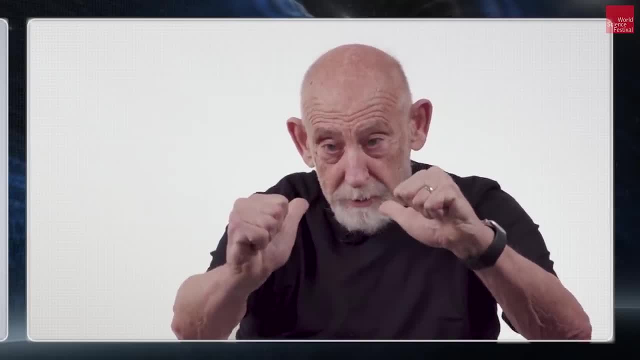 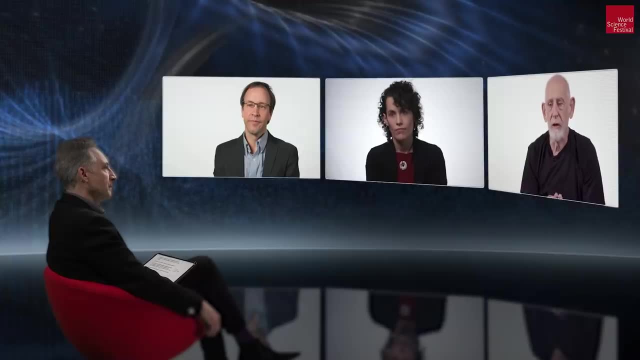 They can be pointing toward you, They can be pointing away from you, and so forth. An entangled state is exactly what you said. It's a situation where you can know everything that can be known, everything that can be known- The nature. 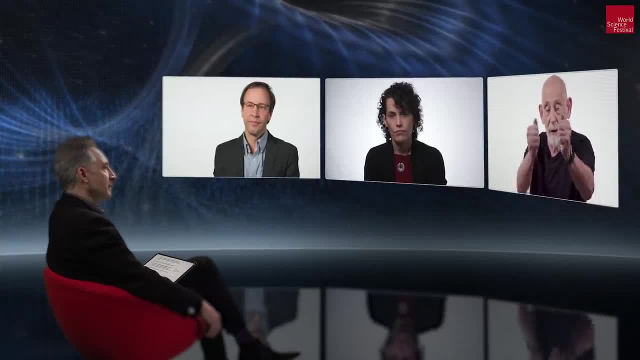 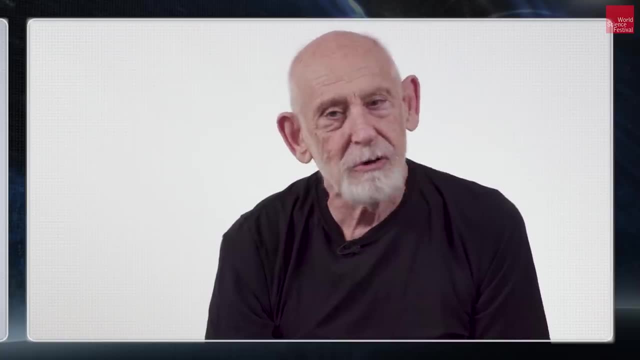 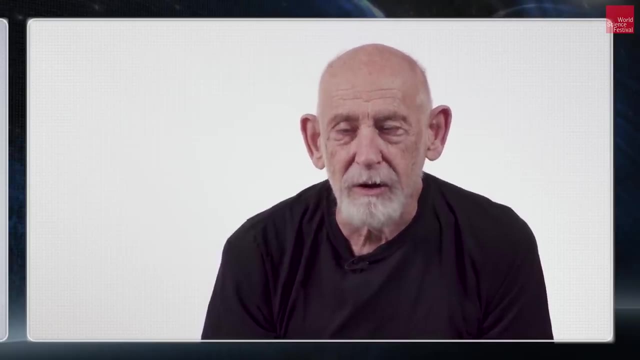 Mechanics say that you can know. You can know everything that can be known about the composite system and know nothing at all about either of its parts. Now, how can that be? I am absolutely certain that that's what freaked Einstein out. How can it be that you know everything that can be known about the composite system and 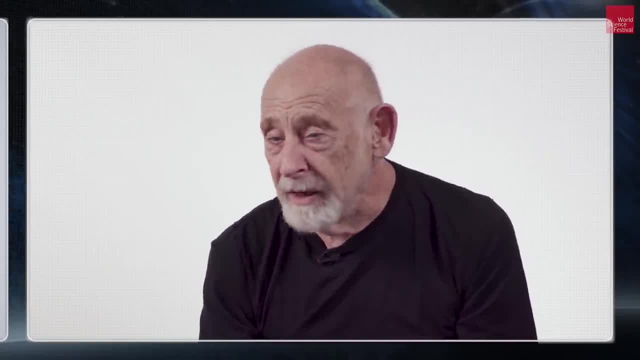 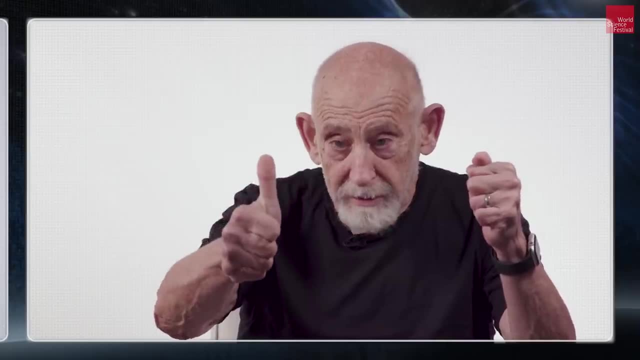 know nothing about the parts. What do I mean about not knowing anything about the parts? Well, you simply…if you make a measurement on one…on this…on this…on this…on this…on this thumb- here it's randomly up or down. 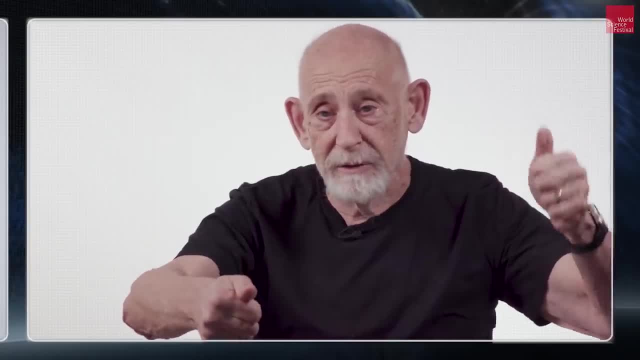 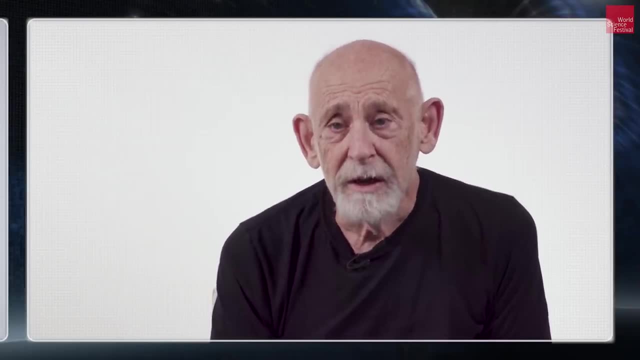 If you make a measurement on the other thumb, it's randomly up or down. You know nothing about it. On the other hand, you know something else. You know correlation. You know that if one thumb is up, then the other one is down. 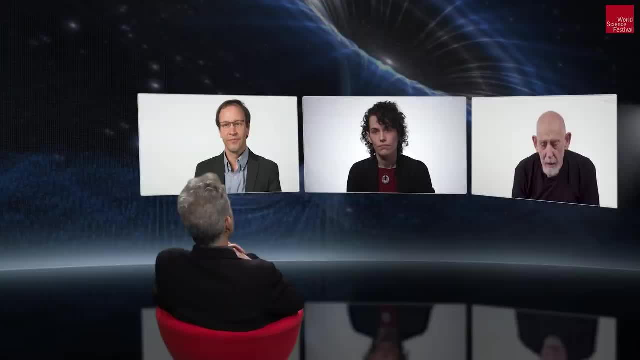 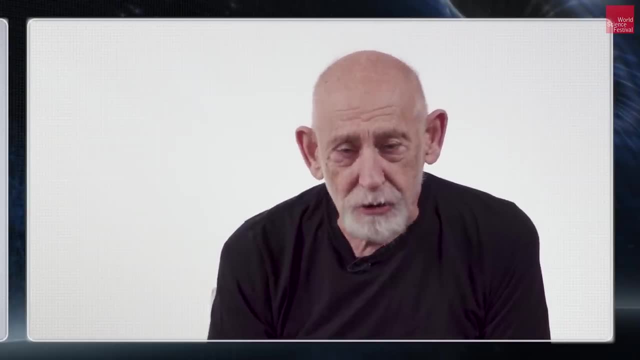 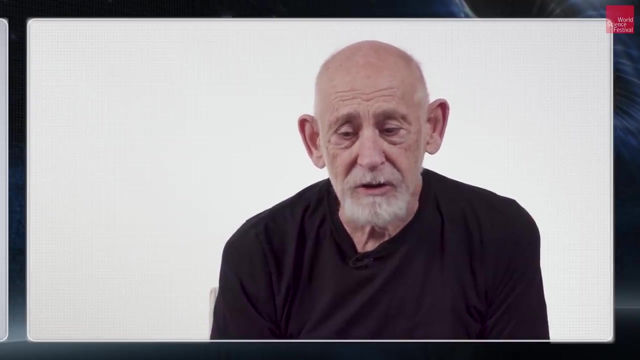 If one thumb is down, then the other one is up, or something like that. So Einstein felt deeply that this could not be the end of the story. He understood quantum mechanics. There's no doubt that he completely understood this and wasn't in the dark about what. 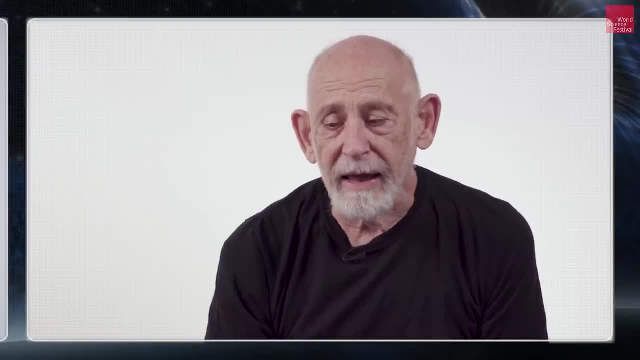 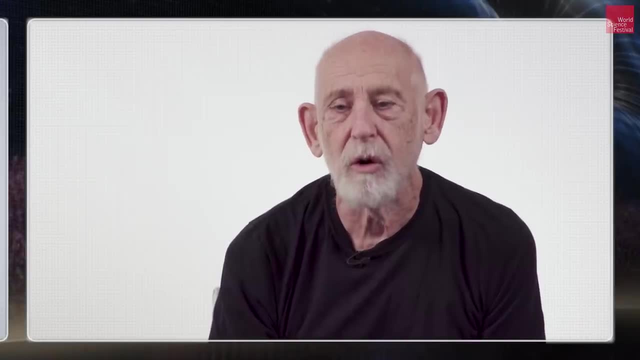 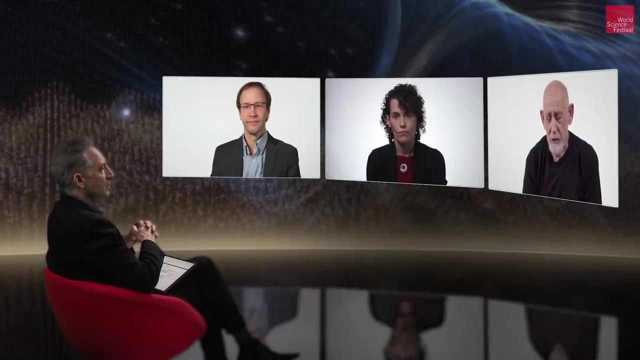 all this meant He simply couldn't…he couldn't come to terms with the idea that you could know everything that can be known about a system and know nothing at all about its parts. That was deep, That was extremely deep, and we're still seeing the repercussions of it today. very 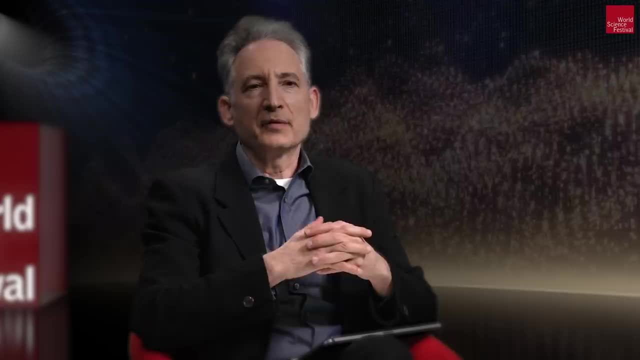 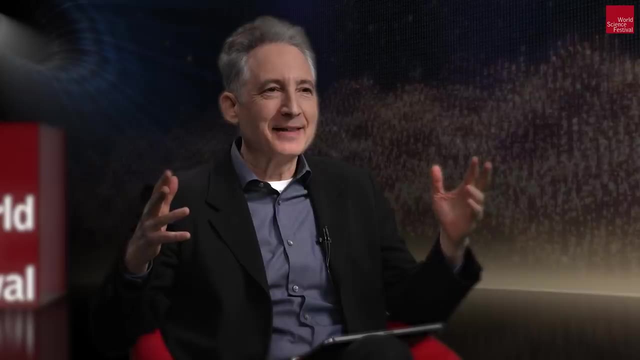 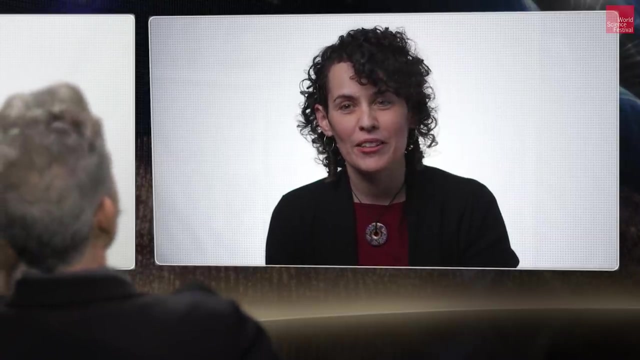 much so, in fact. And so, Anna, if it freaked out Einstein, right, does it freak out you, this idea that quantum mechanics describes composite systems in this strange way? Yeah, of course, I think nobody that have learned quantum mechanics can say that was not freaking out first time. 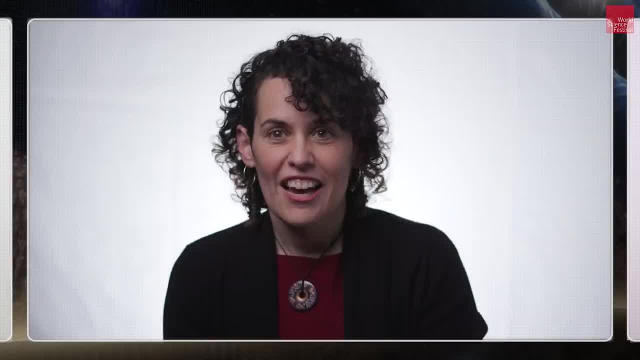 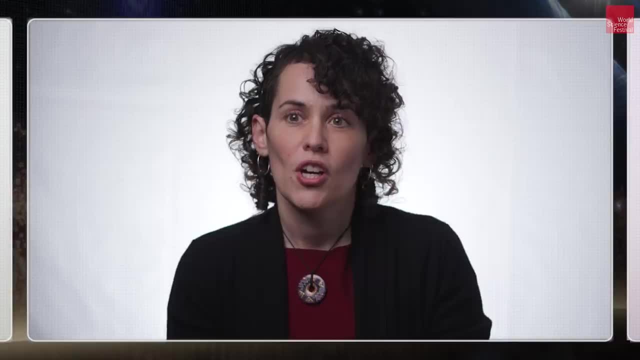 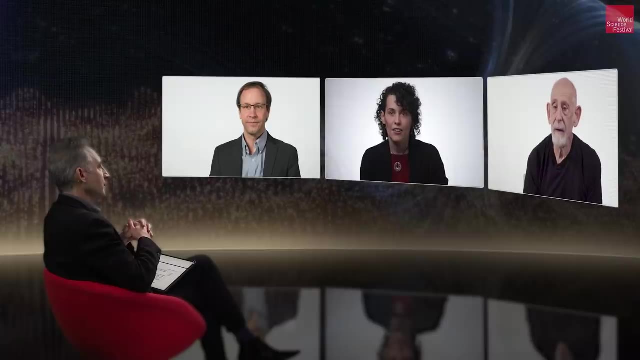 that was learning these things And… I think, getting the…. in our classical world, where we are used to think and to have intuition, it's not easy to change our minds to learn how to take intuition of that. I think it's a change of the tip. 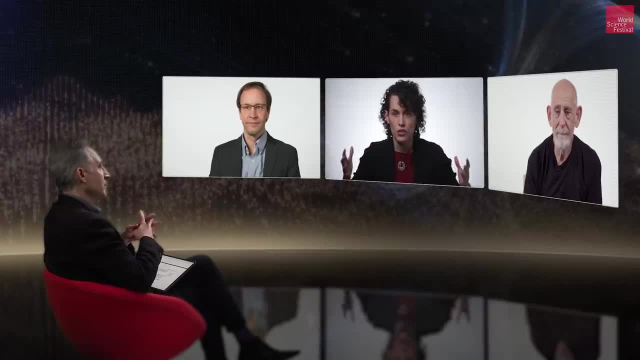 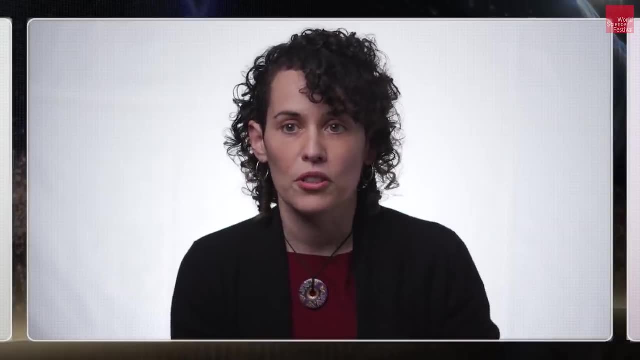 Thinking about that system that they say that is a non-separable system is…that's the…one of the key words is the non-separability there of the…of the whole system. So then you cannot know individually anything completely So, Marc. 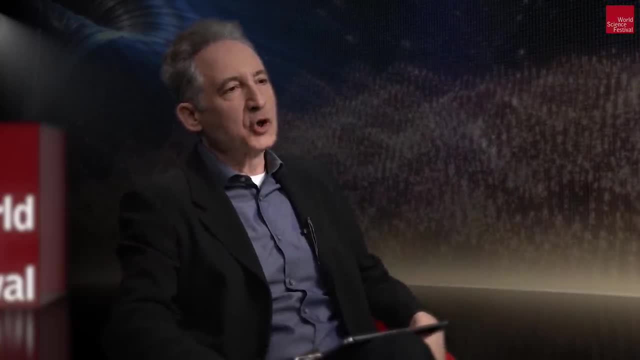 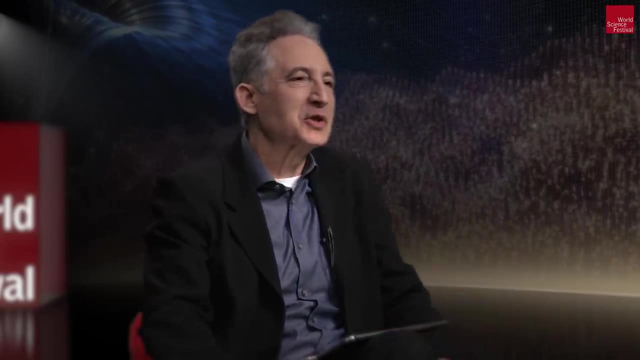 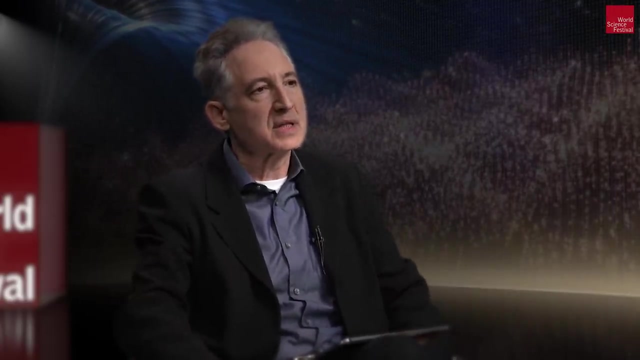 Historically speaking, what did Einstein do with this freaked out reaction to quantum mechanics? Did he just leave it at that? Did he have a potential solution? Where was he hoping he could push the field by emphasizing this weird quality of quantum systems? 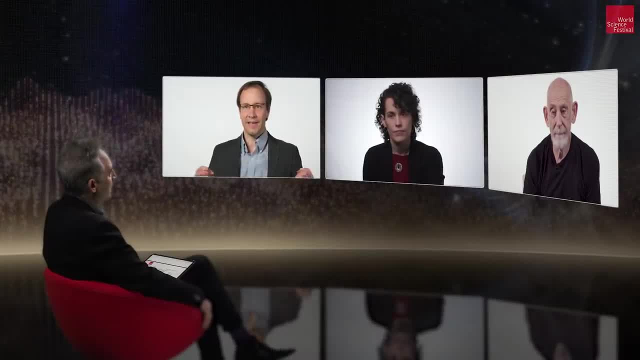 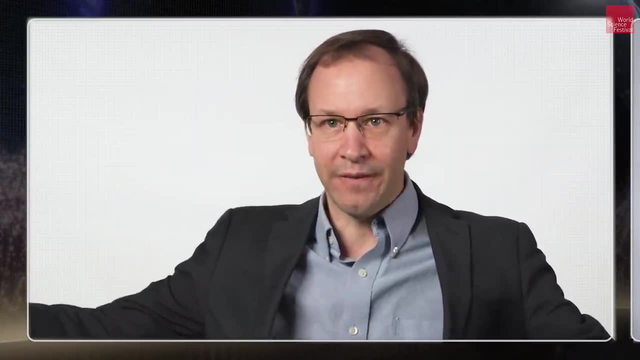 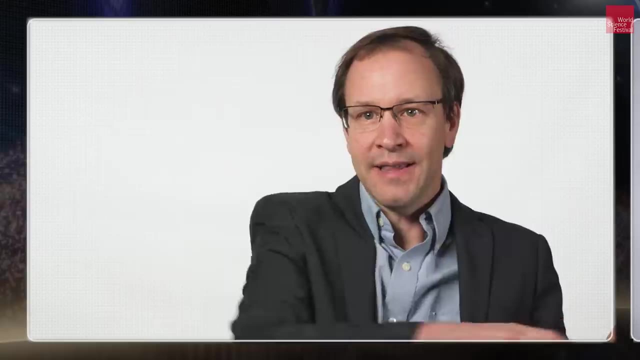 Yeah. So Einstein thought that this idea that you could have an entangled state widely separated…there are the two parts. The two parts were so far apart that they weren't interacting at all. So then the idea that you could measure one part and then immediately know what's going. 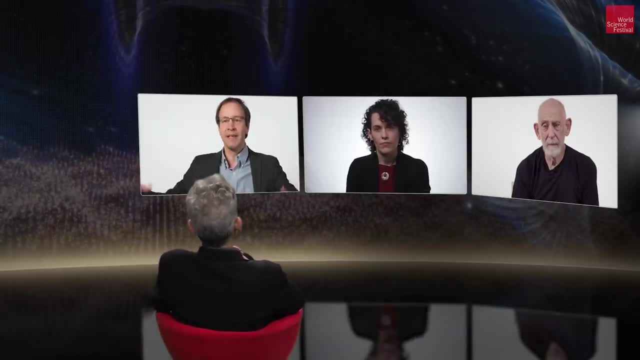 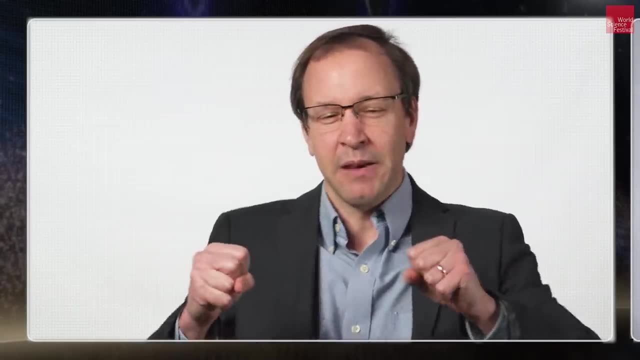 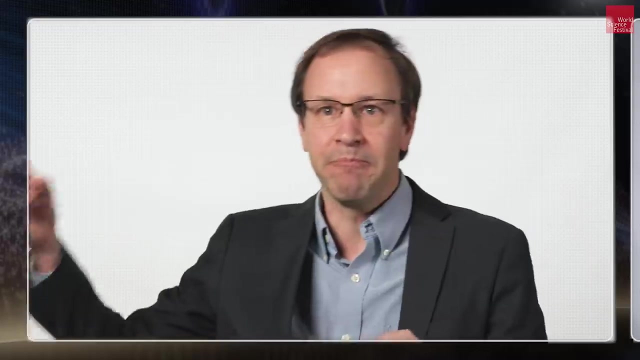 on with the other part. Specifically in the paper, they just tried to show that…they tried to show a contradiction that the standard story in quantum mechanics with a pair of particles…so there's the Heisen uncertainty principle statement that you can't know the momentum and the position. 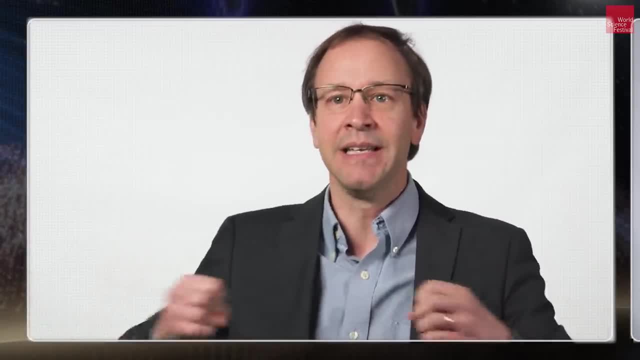 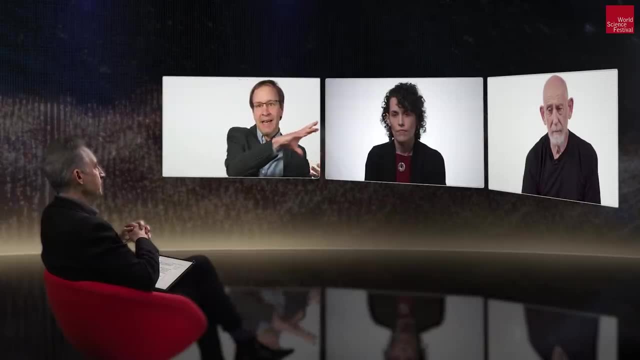 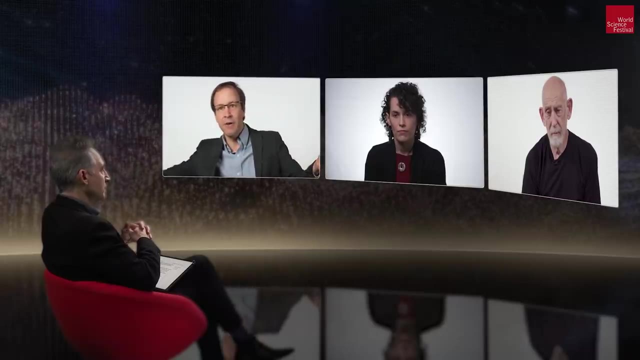 at the same time They wanted to set up kind of a contradiction to show that if you have one of these entangled pairs of particles, then by looking at one of the two particles in different ways, you could either say look at the momentum and then you would know the momentum of the other. 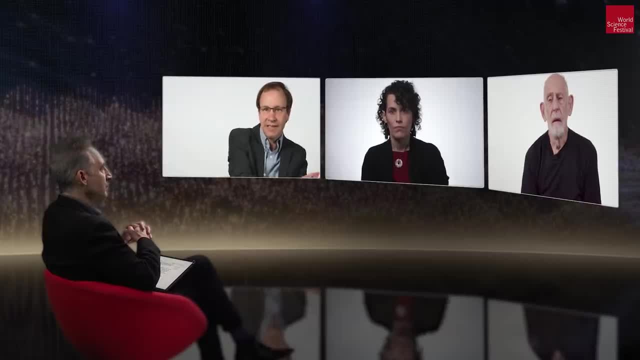 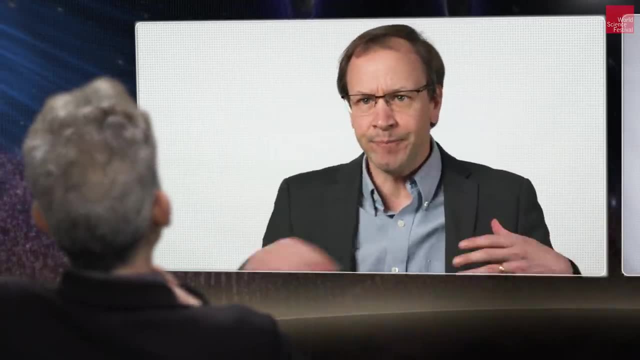 one because of the entanglement, Or you could look at the position and then you would know the position of the other one because of the entanglement. And then they go on to say that, well, because I could have done either one of those things. 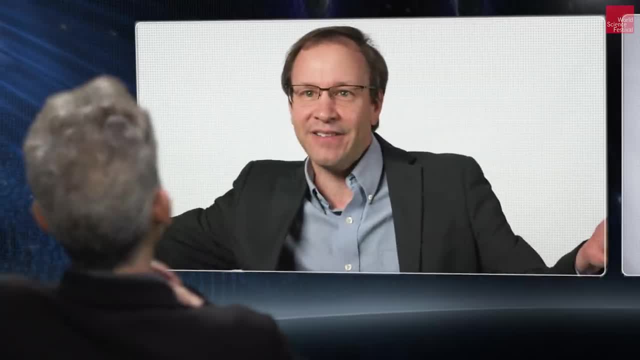 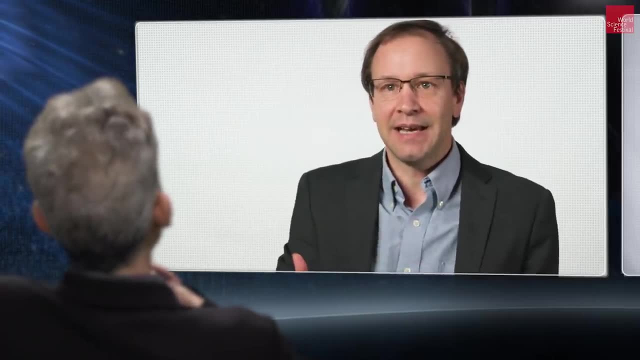 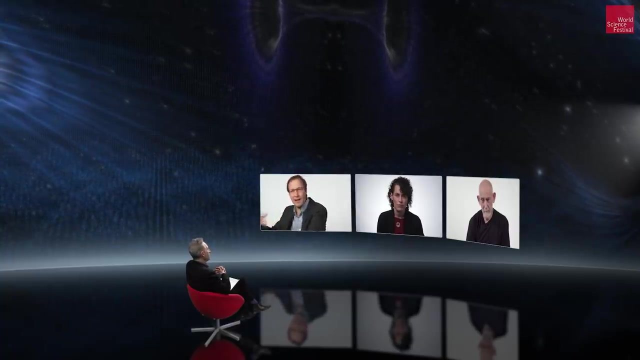 and because, well, there's no way that that could have an effect on the other side because it's not interacting, it's too far separated. Then they suggest that, well, that sort of shows that you could know both the momentum and the position of the other one, and that's sort of a contradiction with the Heisenberg. 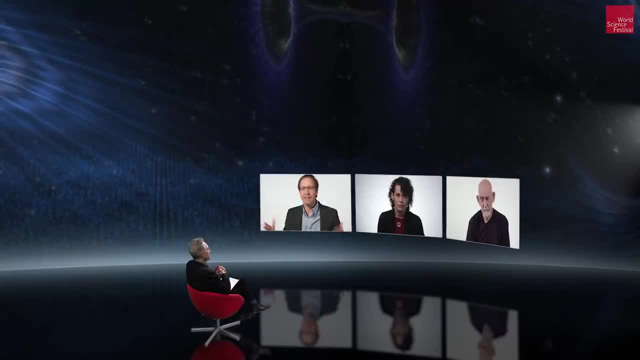 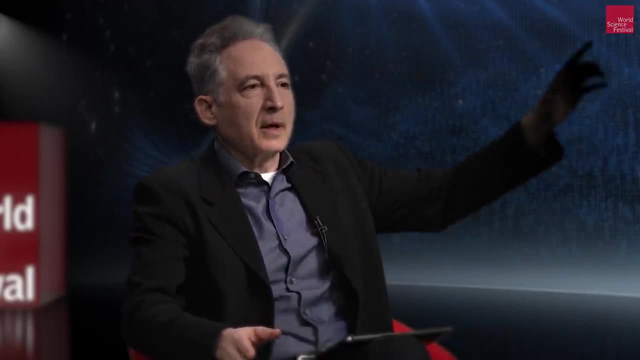 uncertainty principles. So things just don't seem self-consistent, Right, I guess, with the idea being that if somehow a measurement in New York is telling you something about a particle in Los Angeles, then it must be according to Einstein and colleagues. 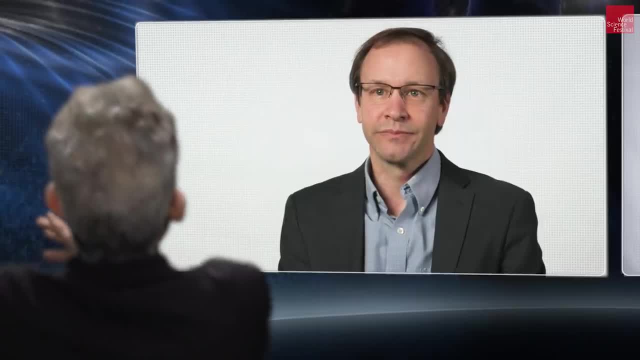 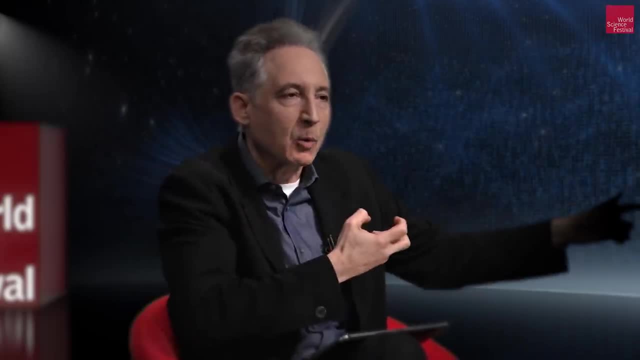 that the particle in Los Angeles always had that quality, even if quantum mechanics wasn't able to tell you what that quality was. It can't be that what you do in New York is literally bringing that quality to a definite circumstance. That just seems kind of crazy. 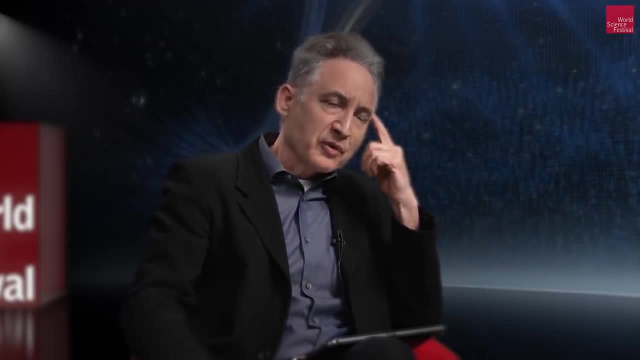 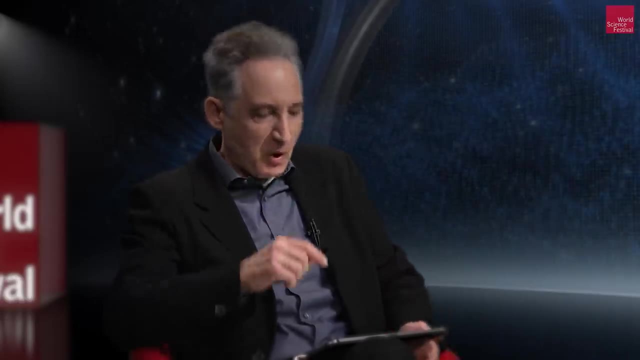 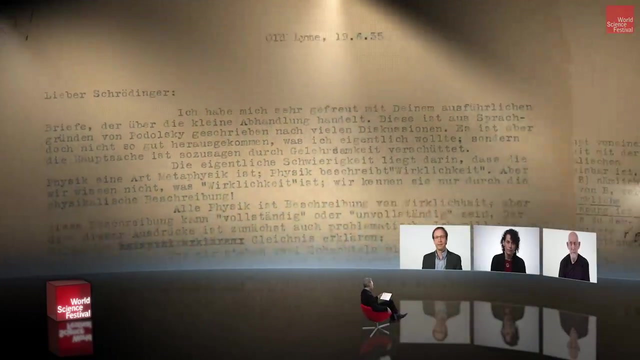 And it's an interesting historical fact again that's worth noting. Einstein wasn't very happy with the EPR. There's this wonderful quote which I happen to have here, because Schrodinger wrote Einstein a letter after the EPR paper kind of congratulating him on it, saying it was a really good observation. 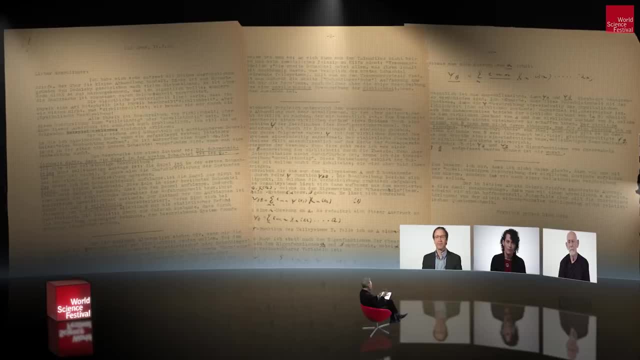 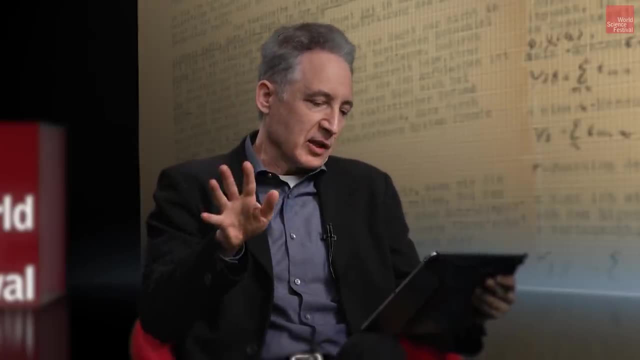 Einstein then writes back to Schrodinger. Here's what he says. He goes: I was very pleased with your detailed letter which speaks about the little essay, the essay being the 1935 EPR paper. Then Einstein goes on. for reasons of language, this was written by Podolsky. after many 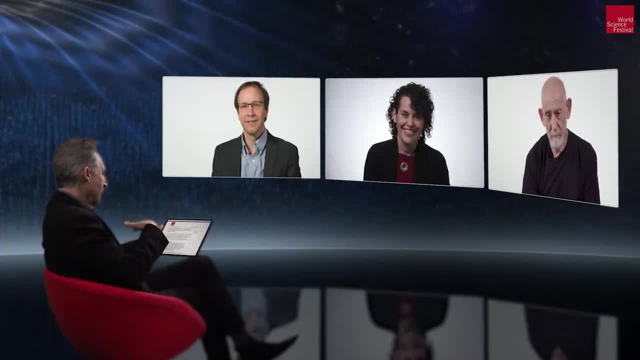 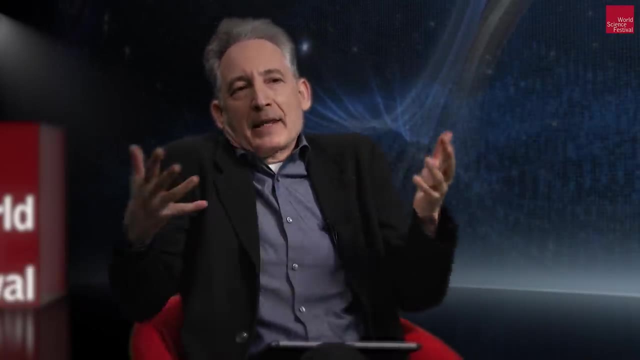 many discussions, but still it has not come out as well as I really wanted. On the contrary, the main point was, so to speak, buried by the erudition. So he wasn't thrilled with how this paper turned out And, Lenny, I think it's because Einstein wasn't pleased, as Mark recounted that the EPR paper 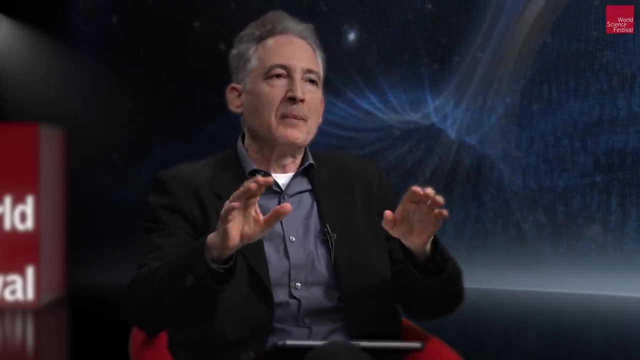 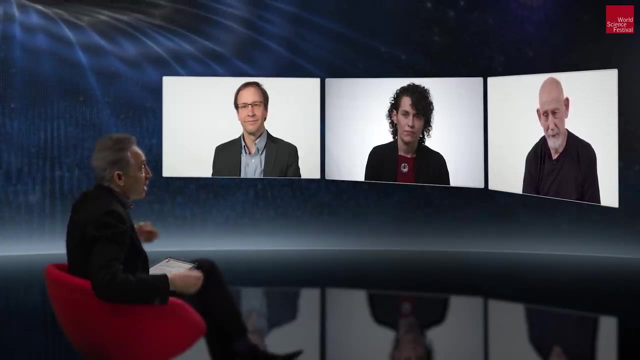 focuses on Heisenberg uncertainty principle. It focuses upon a counterfactual Right. It imagines that you could measure this or you could measure that You know. a contrarian could say: well, you can't measure them both. on the first particle. 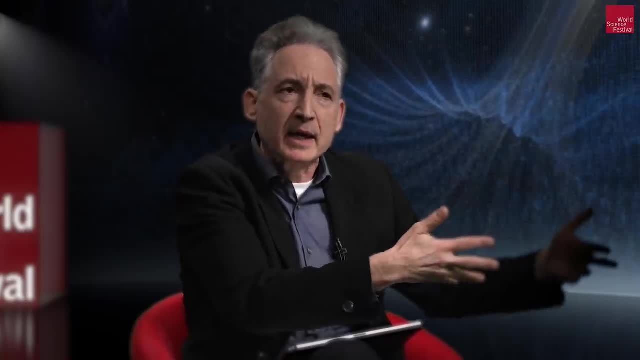 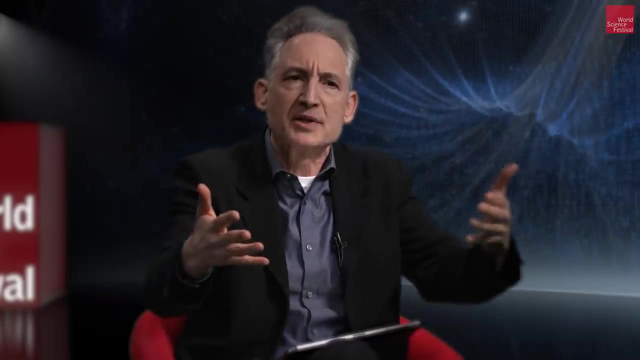 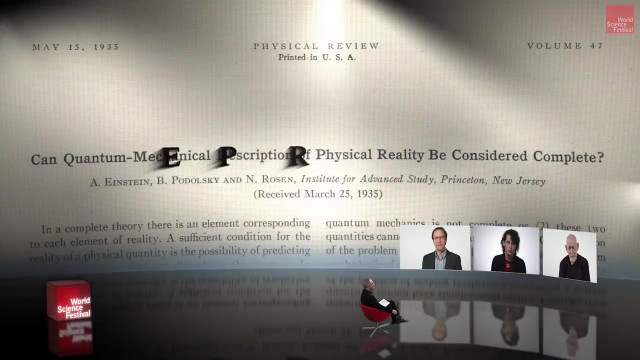 so can you really draw any inference about the qualities of the second? So he saw this as much more general, I think, than what the EPR paper even discussed. Is that your take on it as well? Yeah, very much so. You know the letters E-P-R. we all know what they stand for, right? 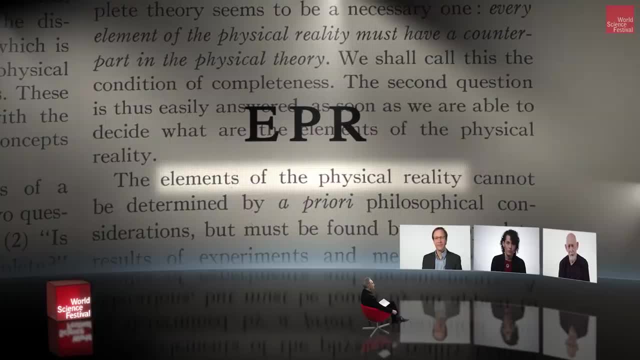 When I first learned about it, I was told that EPR stood for elements of physical reality, which is a term that appears in their paper. When I learned about EPR, it was elements of physical reality, And it was very clear that that was what was bothering Einstein. 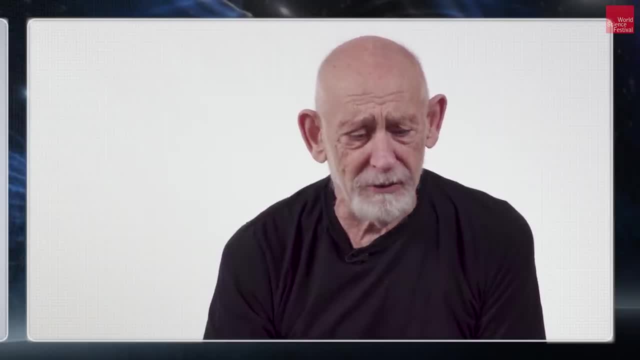 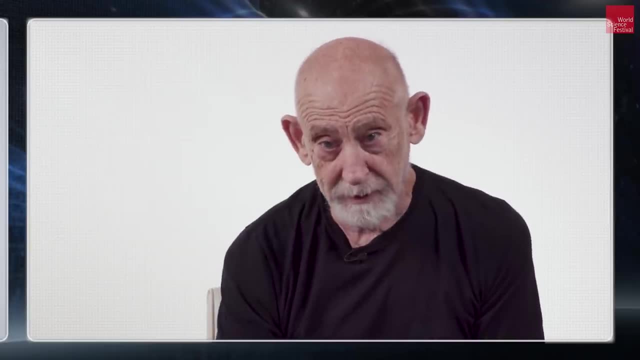 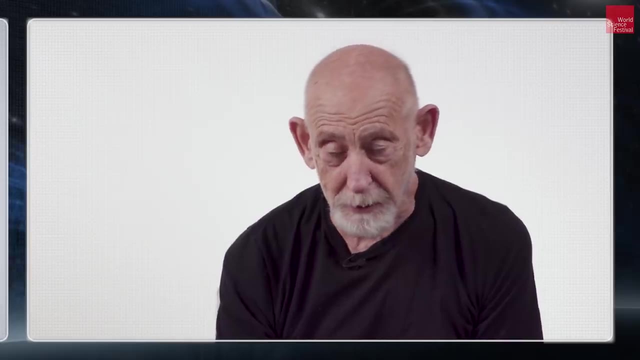 What is real? What is real, What is at the bottom of everything, What is really unambiguous, What is objective As opposed to what's in our minds, Right And what we decide to measure and don't decide to measure, and so forth. 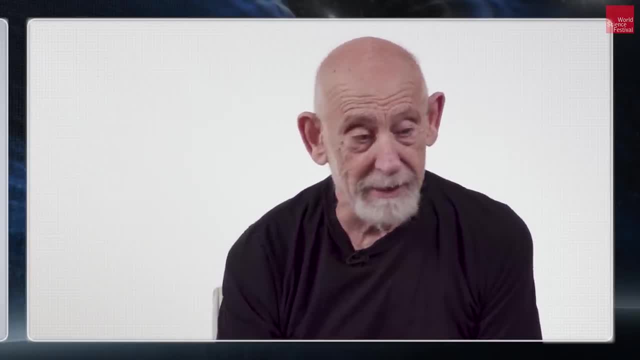 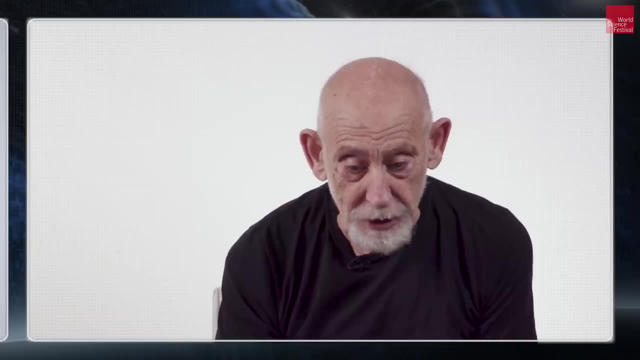 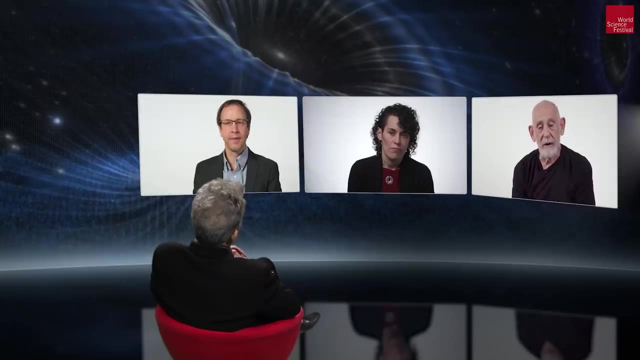 What is real. Einstein was a realist. I mean, he was a realist in that he believed deeply that there's something real and something underlying that is objective, almost classical. Yet he knew that quantum mechanics didn't work that way. I don't know that Einstein was trying to overthrow quantum mechanics or that he was trying to. 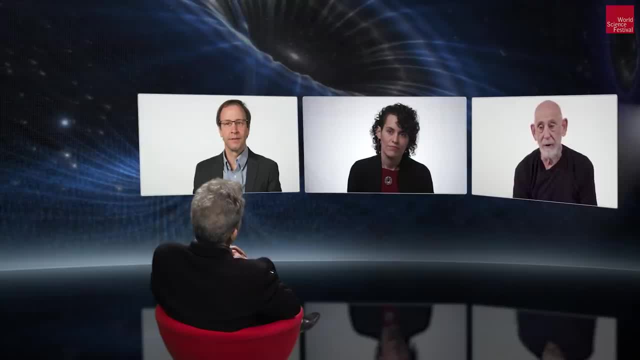 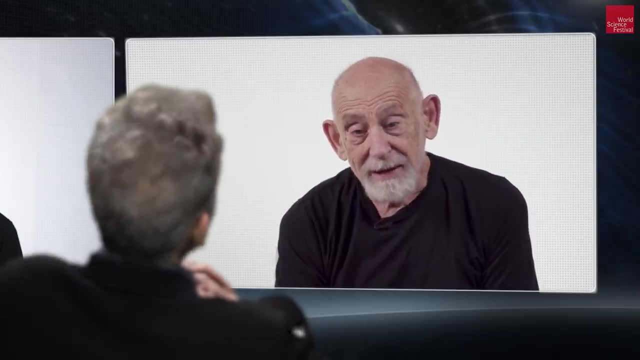 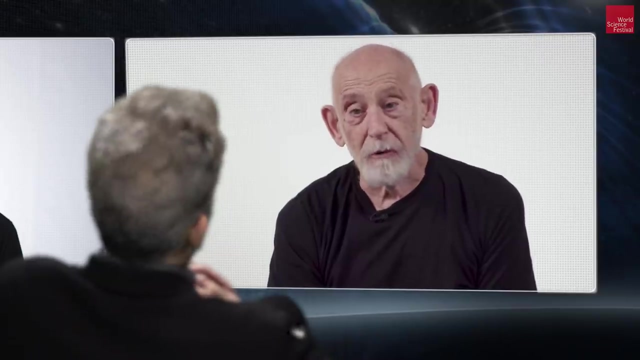 find a contradiction. I more or less read the paper as just saying: Isn't this very weird? This can't be the end of the story. That's more or less the way I read it, And with no particular prescription about where it was going to go from here. 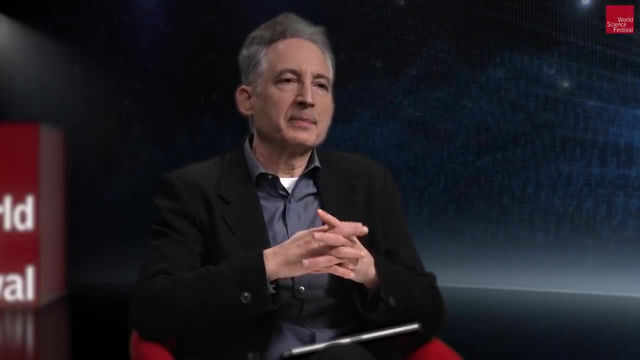 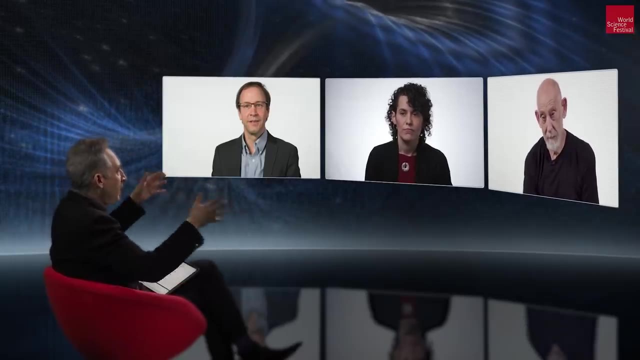 So I mean this is probably the same with all of you, but if I was to count up the number of times that I've been asked by members of the general public, okay, do you really understand quantum entanglement? I think it's the question I've been asked more than any other question. 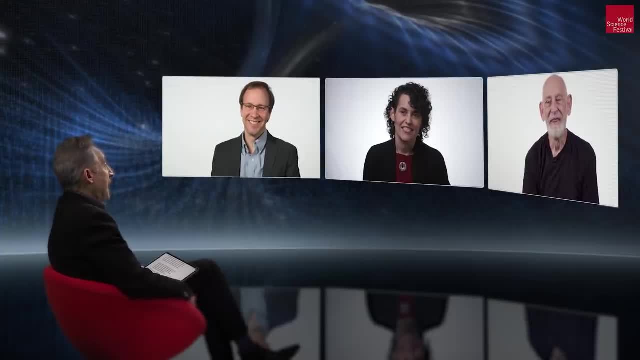 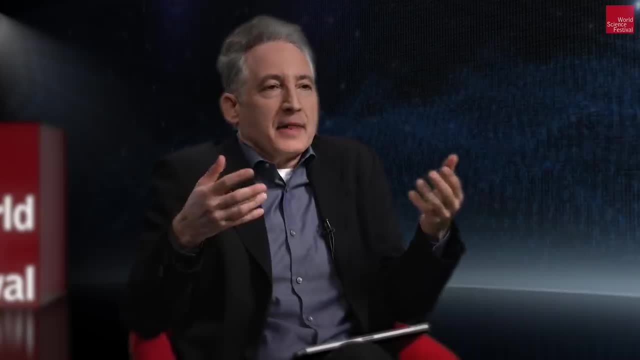 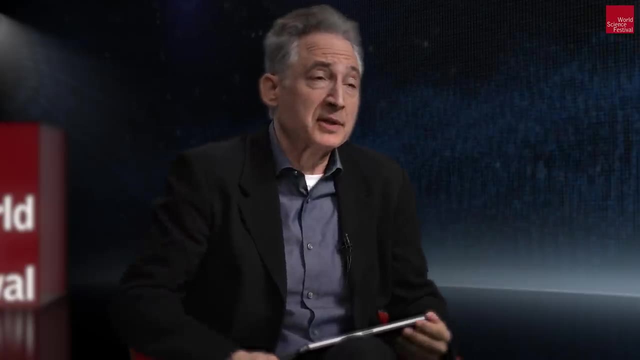 And I don't mean to get all meta on this, but I think the answer in part depends on what one means by the term. understands, right, We can make predictions on it and so forth, but I mean, Ana, what's your view? 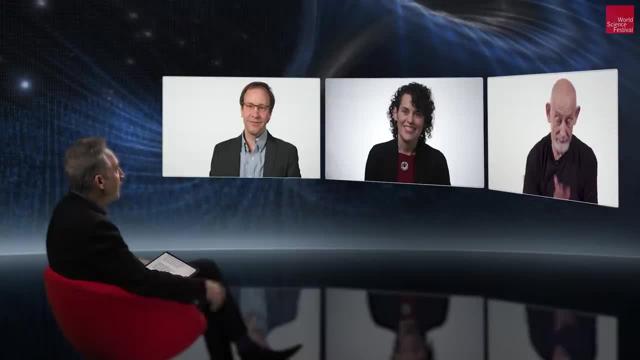 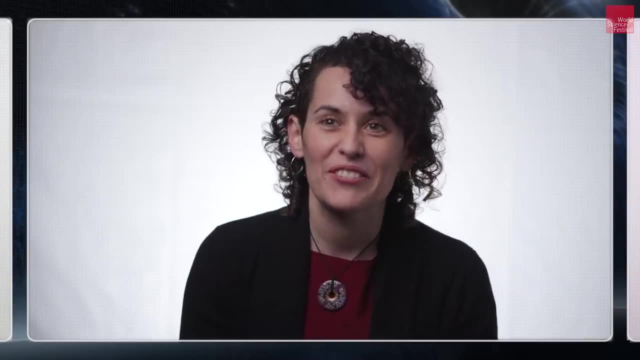 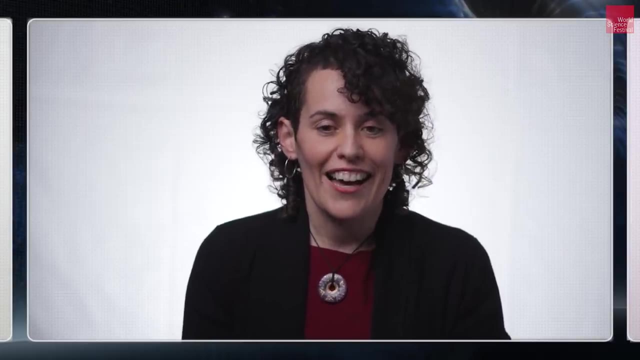 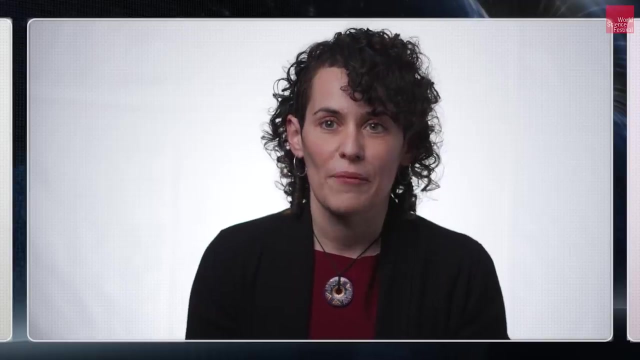 If someone interrogates you and says: do you understand quantum entanglement, What do you say? Yeah, In fact, this is something that I've been asked a lot of times by family, friends and in several talks And, as you pointed out, it's very interesting the point that how do we understand the understanding? 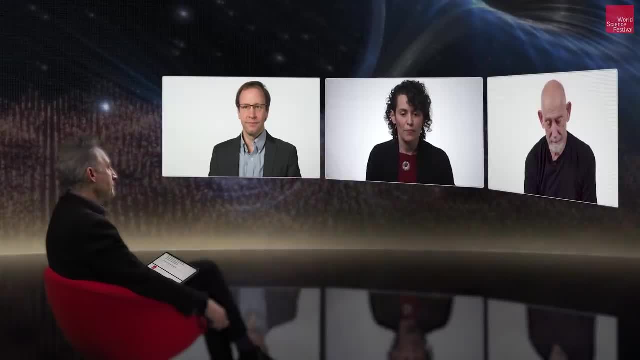 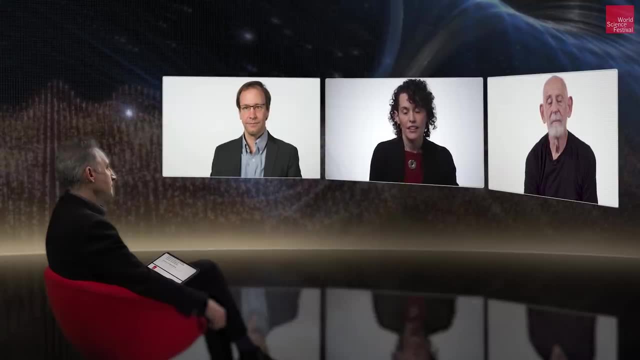 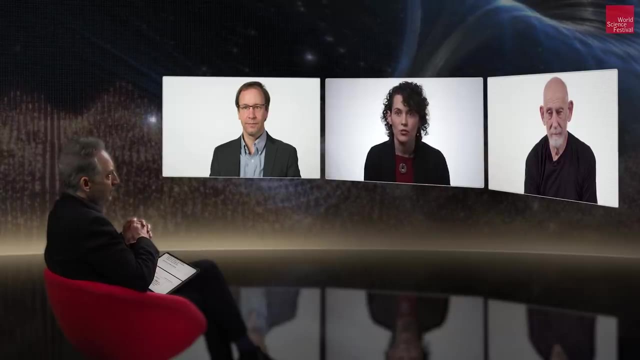 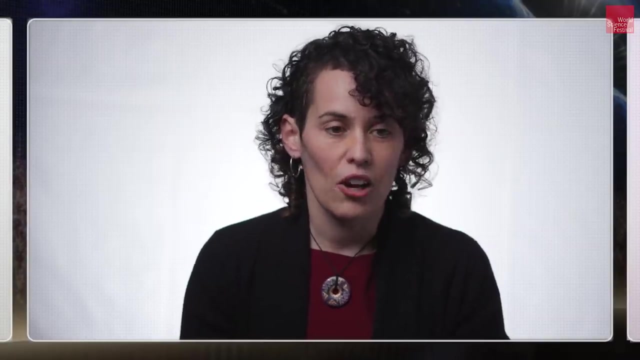 of the quantum mechanics, Because sometimes the most powerful part of these theories of quantum mechanics and the developments further in the future, like quantum field theory and everything, are the extremely accurate predictions, Yeah, That they have given us. It's incredible how well they work, how they allow us to make things work even in our 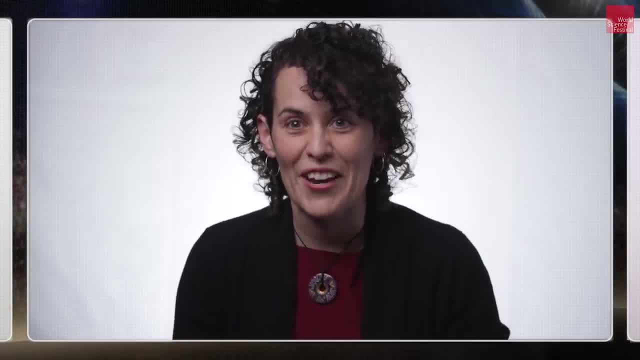 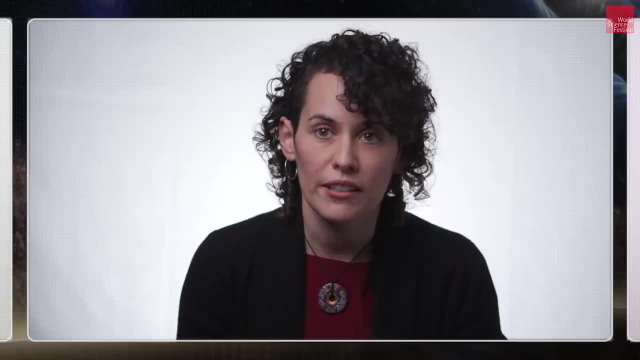 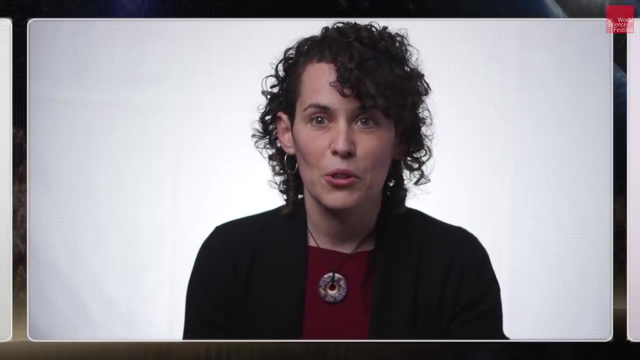 normal life, the devices that we are using for this conversation and everything. So I think that's a real understanding how we can use this to predict and to create new things. But the difficult part of this understanding is how you transmit to the general audience. 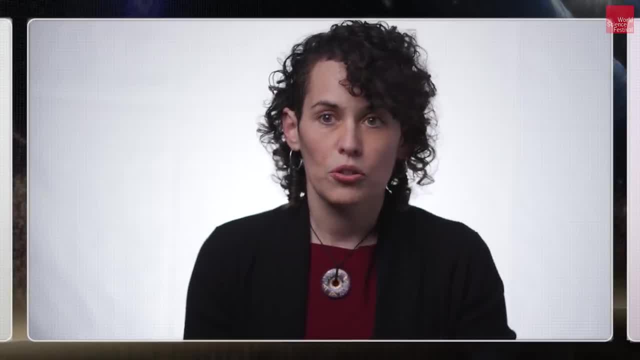 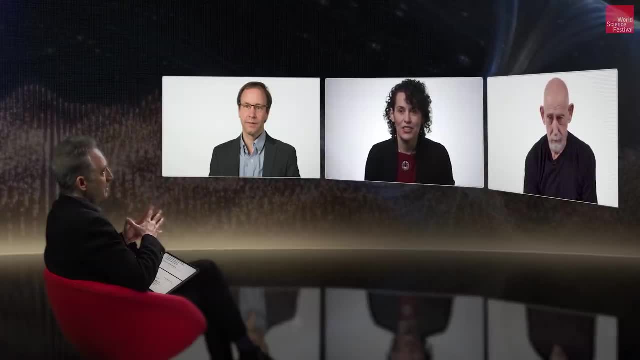 Because when you want to transmit things to the general audience, it's very difficult- The general audience. you tend to use metaphors or you know similarities with real life And, as I said before, this is not in our daily intuition. 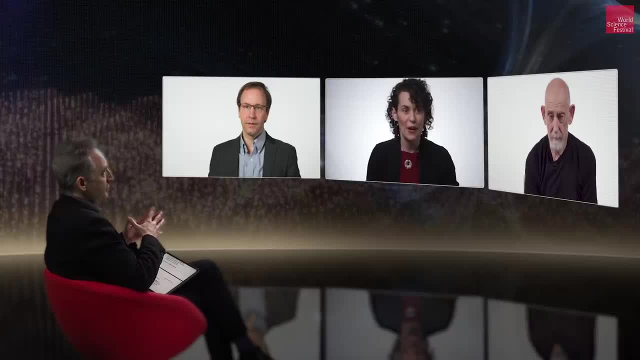 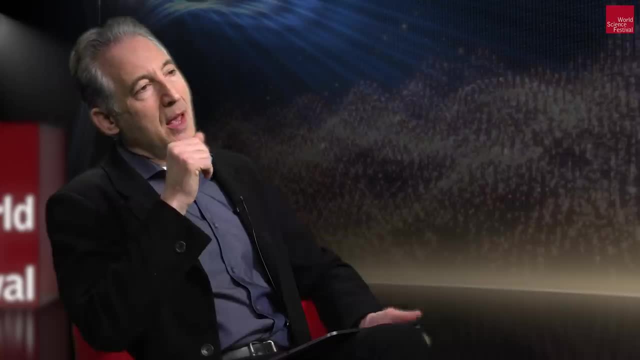 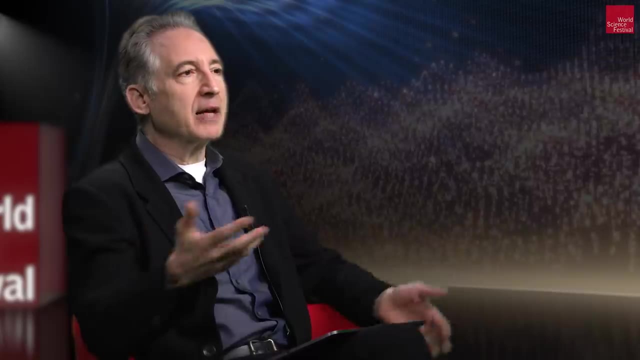 So then when it's problematic, like, oh, what is my understanding of this when I compare it with my daily life? And yeah, it's a tricky part- Now there is another tricky part of quantum mechanics, a kind of gap in our understanding. 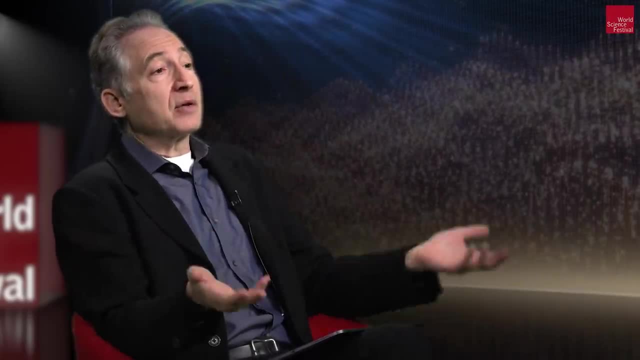 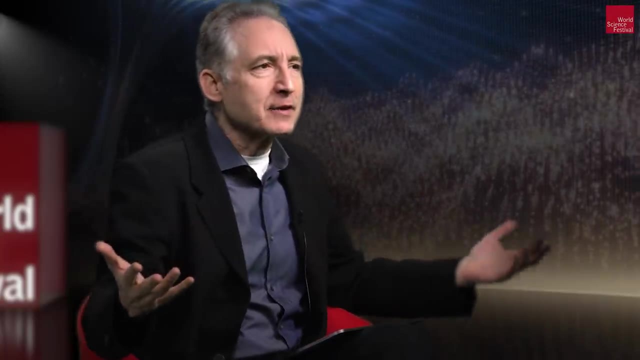 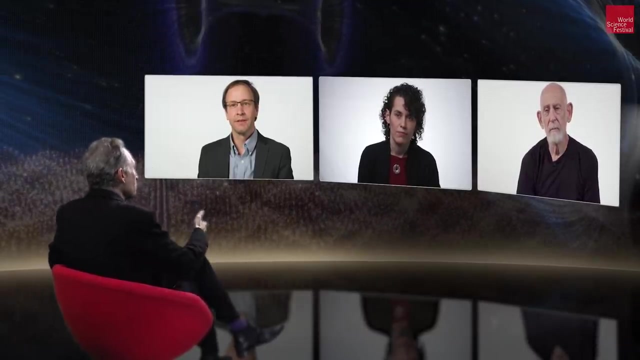 of quantum mechanics, And that's really just behind much of the territory we've been discussing, which is that quantum mechanics describes reality as a kind of fuzzy haze of possibilities that only resolves into the kind of definite reality we all experience when the world is observed. 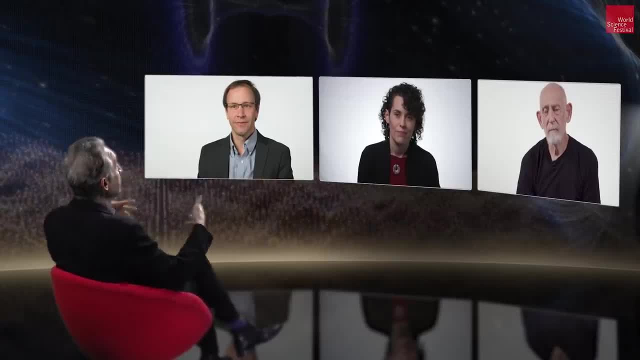 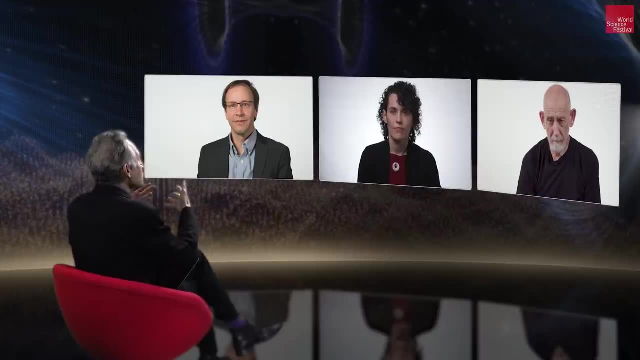 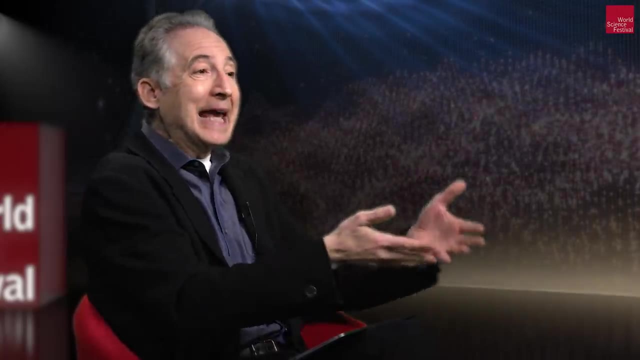 or measured or interacted with in the right way. And yet our quantum mechanical understanding has, at least so far, not articulated how that transition from fuzzy to definite How it actually happens, a transition that is, of course, essential to entanglement. 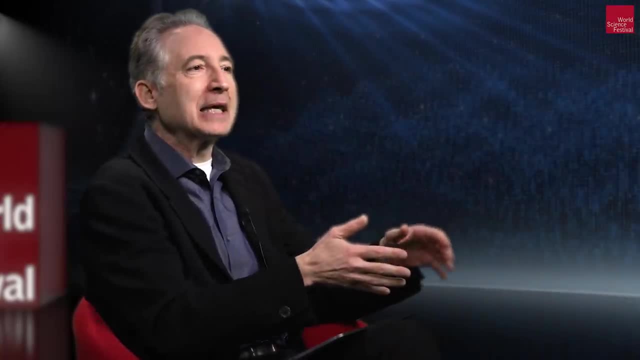 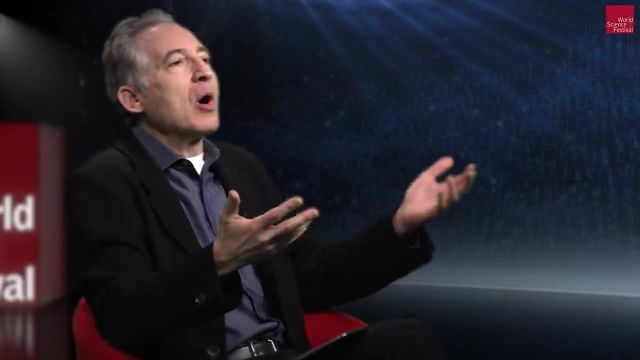 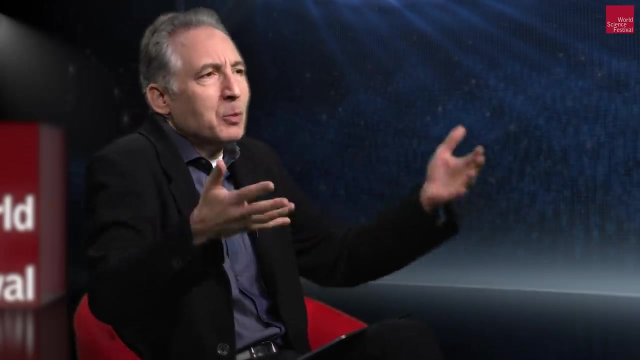 since we're talking about an observation here having a spooky connection to an observation over there. Now, Lenny, does this gap, this so-called quantum measurement problem, does it trouble you, or do you see it as more of a detail that we will one day resolve? 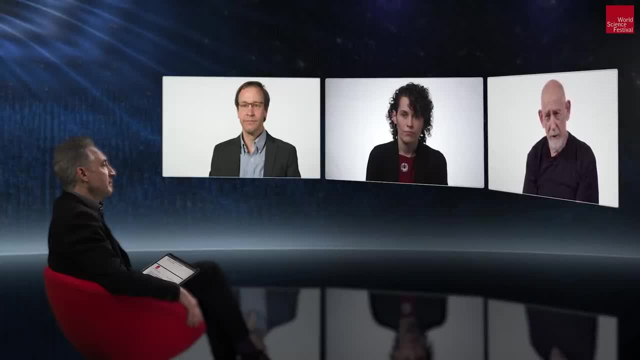 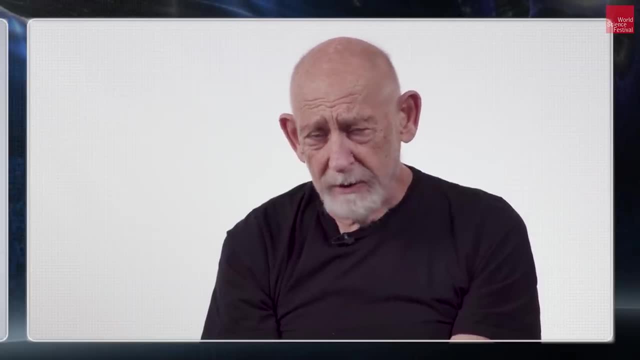 Oh, I don't think it's a detail by any means. I think it's at the. I think it's at the very center of all of the confusion about quantum mechanics, which I share. I mean, I don't feel I understand quantum mechanics at that level. 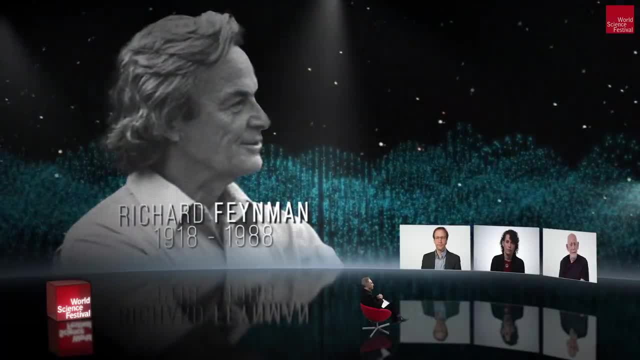 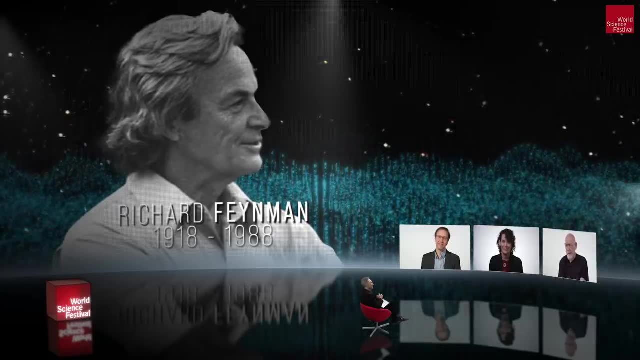 I think it was Feynman who said: I'm so confused by the whole thing that I can't even tell if there's a problem, And I think a lot of us feel that way. On the one hand, we have to use quantum mechanics. 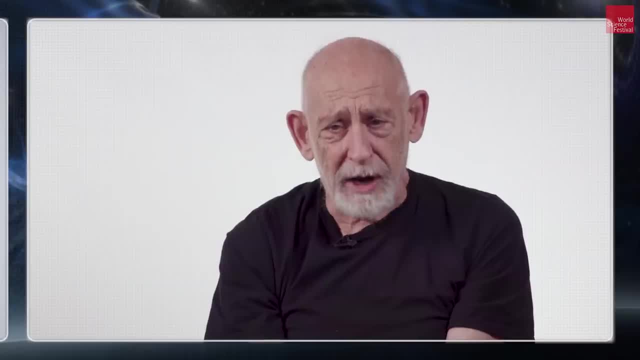 We know that quantum mechanics works. If we want to make a theory of the world, it's got to be quantum mechanical. On the other hand, we're stuck. We're so confused about what the basic conceptual framework of dividing the world into what's. 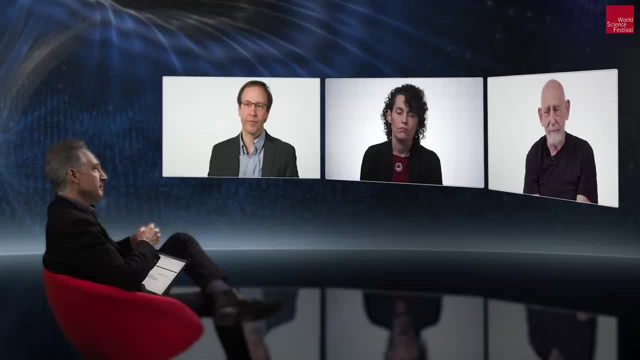 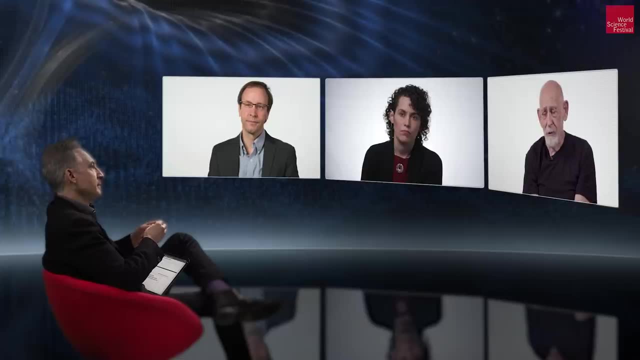 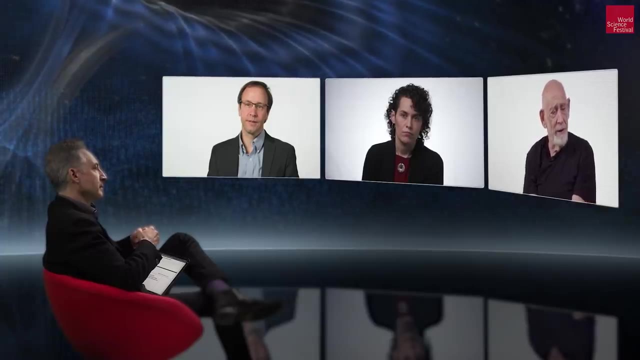 observed and what's not observed, that I personally think there is going to be another quantum revolution, That other quantum revolution is going to come to grips with this in a way that we can't conceive of yet. But I also have the. probably a lot of people think that. 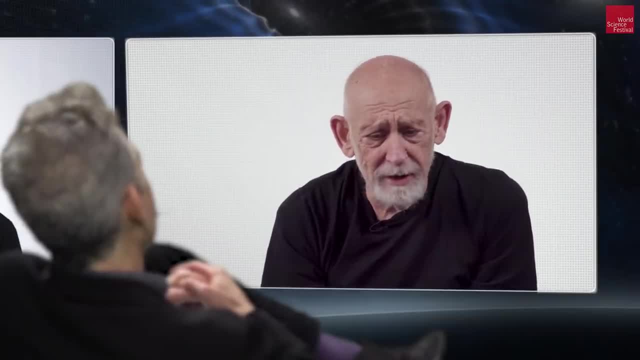 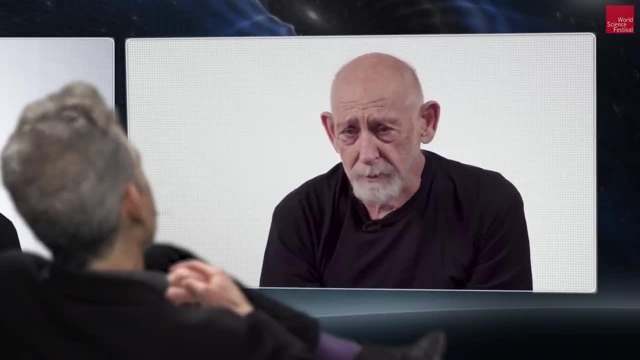 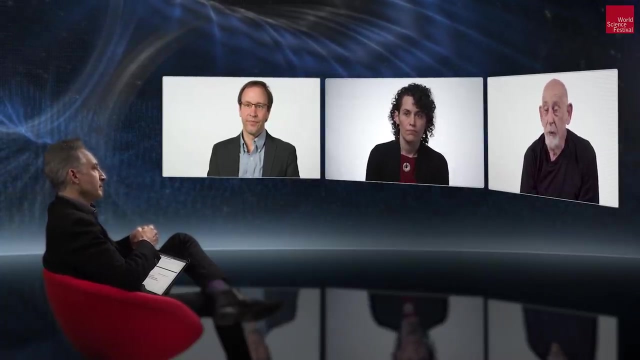 Okay, My guess- and I wouldn't be surprised if Mark shares it- is that we won't get that deeper understanding until we understand the relationship between quantum mechanics and gravity, quantum mechanics and the geometry of the world, And we don't fully understand that yet. 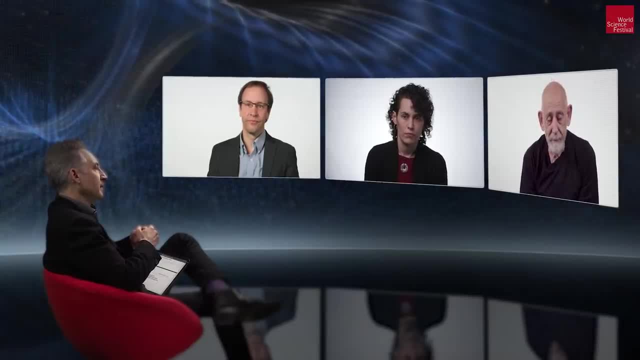 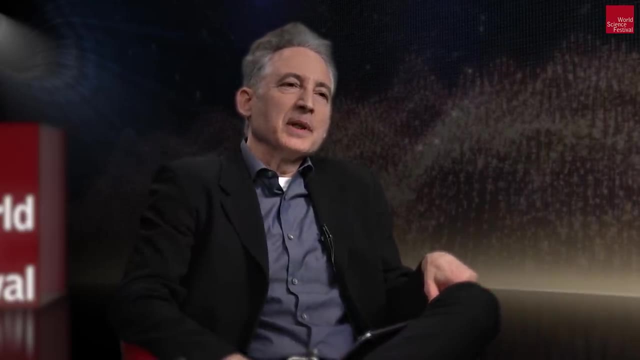 We're making a lot of progress, But I think it's not until then will we have a chance at understanding these deeper issues. That's a That's a great segue, So why don't we turn to gravity, general theory of relativity, where we're going to ultimately? 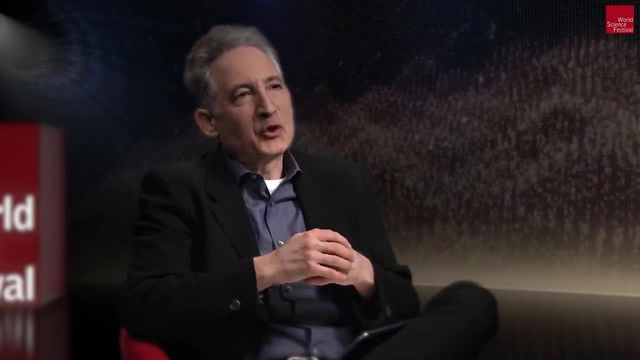 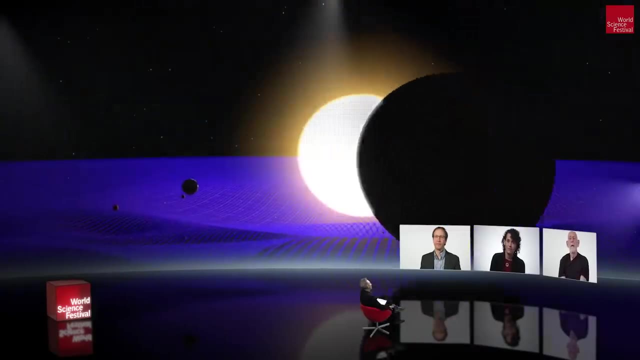 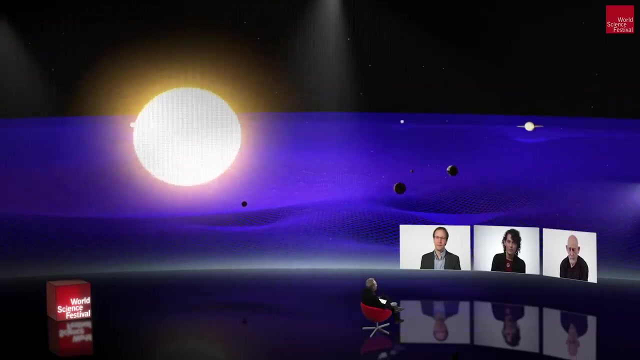 take up a second of Einstein's 1935 papers. So Mark Einstein gives the world this beautiful theory of gravity, the general theory of relativity, where now gravity is translated into geometry, warps and curves and space and time and so forth. 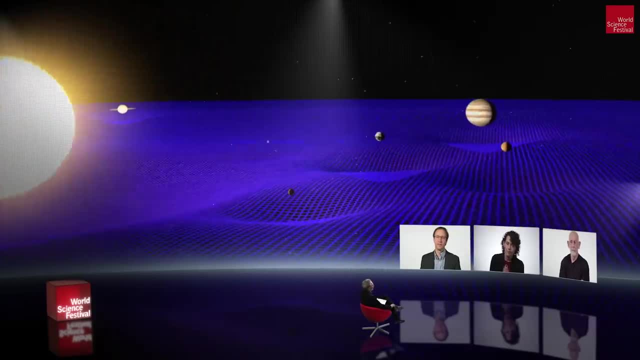 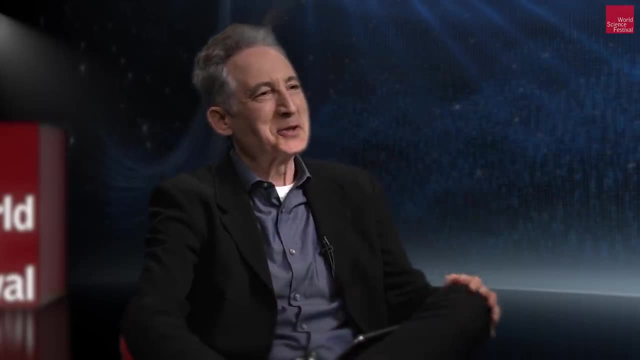 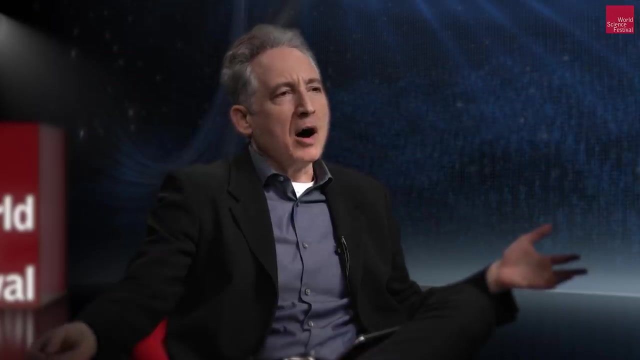 A sort of beautiful encapsulation of how the force of gravity actually works, 1919, it's confirmed, or sort of confirmed, depending on how you look at the history of it through the bending of starlight by the sun. But then interest in general relativity seems to taper off. I mean, why was that? Why wasn't that beginning? Why isn't that beginning of a sort of new era of gravitational study? Why did it sort of begin to die away? Yeah, that's a good question. I'm not sure I know the answer. 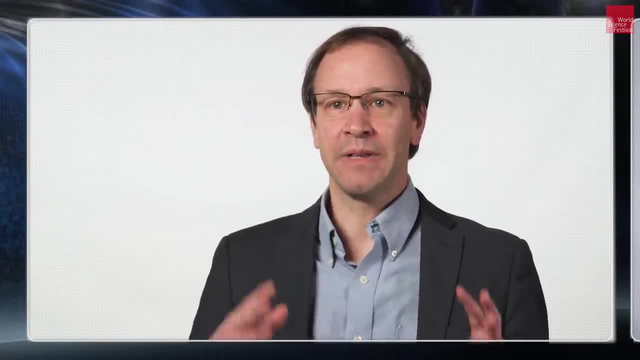 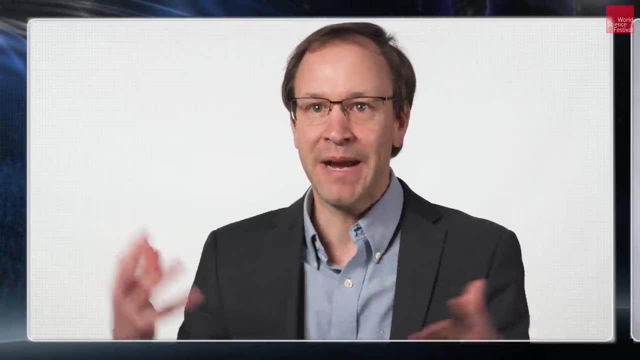 I mean I'm guessing that it was probably. I mean I'm guessing that it was probably the beginning of a new era of gravitational study. I mean it was probably seen as still maybe a little bit esoteric and mathematical and difficult to maybe compare with experiments that we could readily do in laboratories. 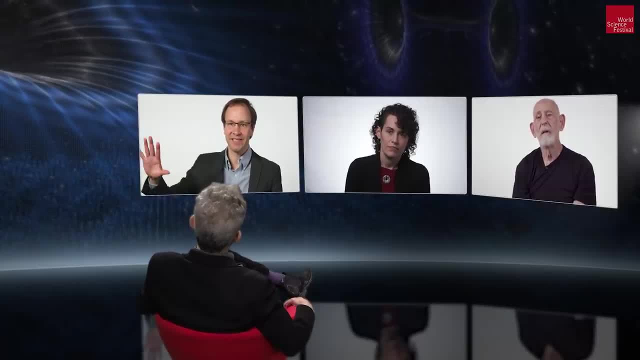 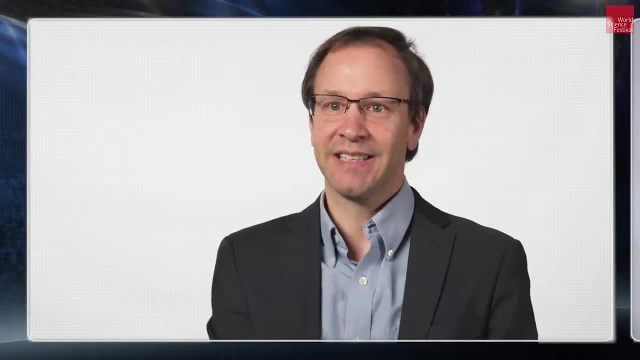 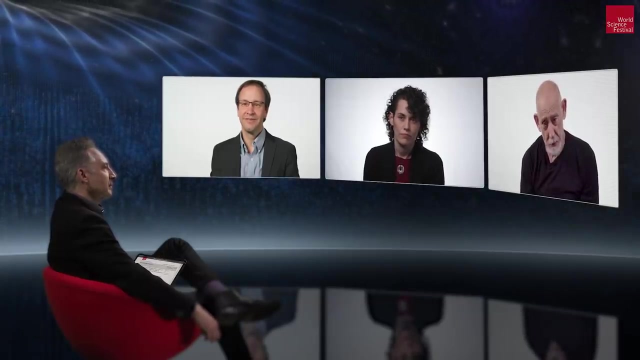 So it may have been that it was still seen as just not quite practical physics yet. But maybe Lenny wants to comment. I lived through that era. I'm old enough to have been part of that era When, grown up, physicists- Physicists- didn't think, grown up in quotes, physicists did not think about general relativity. 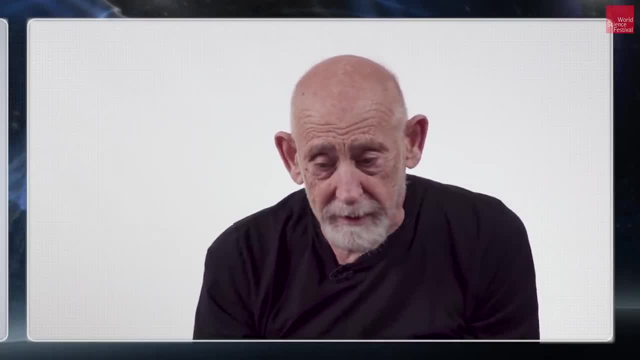 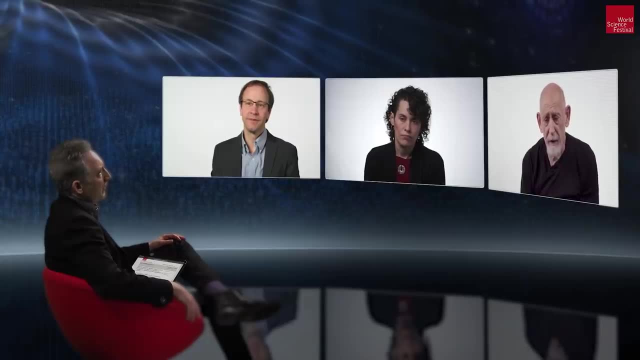 Part of the reason. Mark said part of it well, that it was very, very hard to get experimental data about it. But the other side of the coin is that it was very easy to get lots and lots of experimental data about other things. 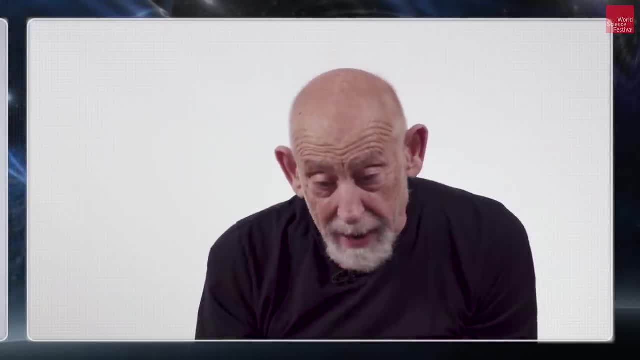 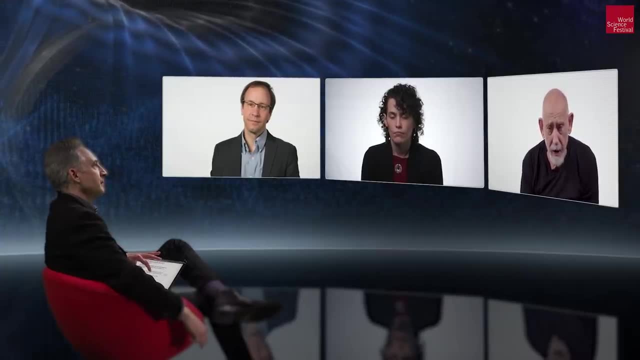 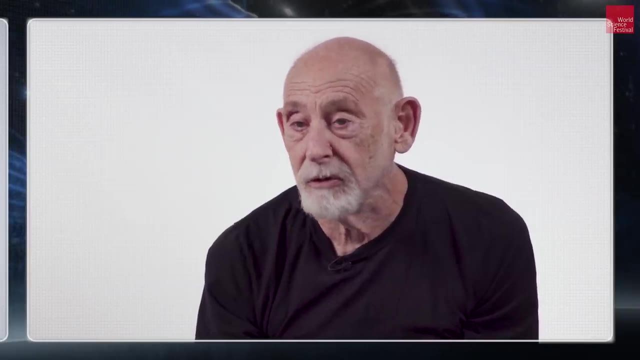 There were other fish to fry, There was condensed matter physics, There was elementary particle physics, And so I think a large amount of it was just physicists had other fish to fry, lots and lots of data, And so it was kind of natural that those who wanted to get ahead, who wanted to do things, 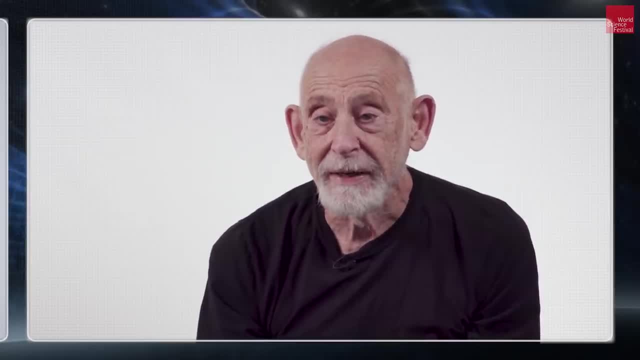 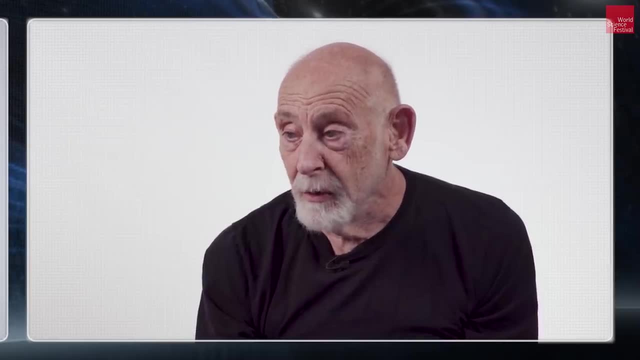 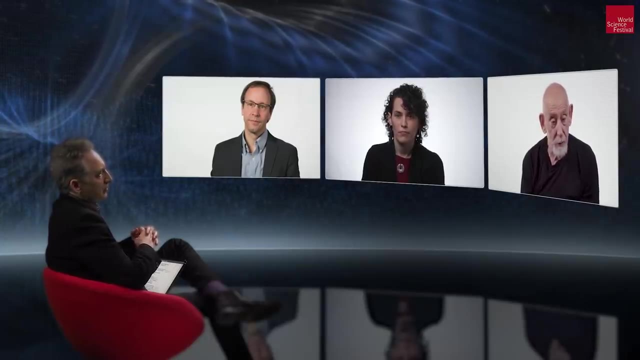 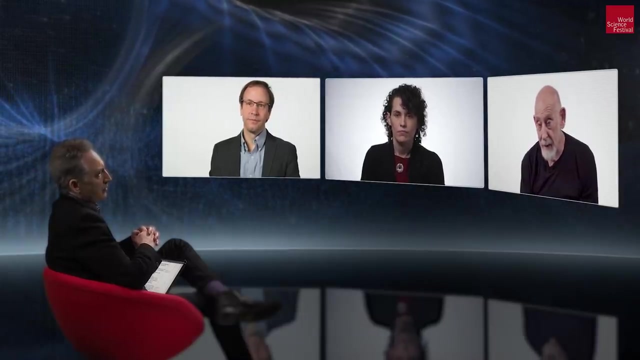 who wanted to get their hands on and maybe win Nobel prizes, would be going in the direction that seemed well. that seemed like it was going to yield to new theory, Whereas gravity was beautiful, It was pristine, It was special, But there wasn't too much you could do with it in the way of experimental data. 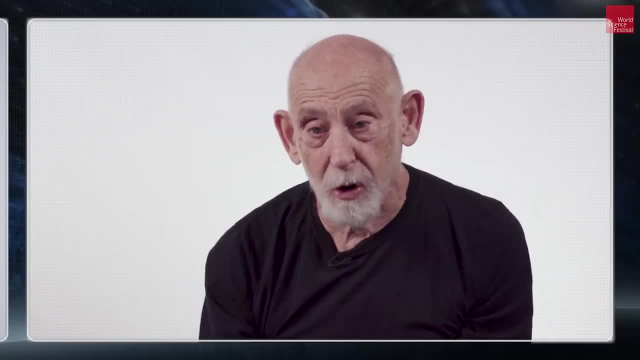 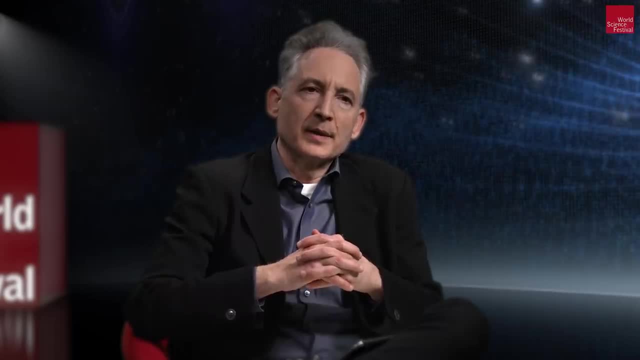 It was just laid out there by Einstein in all its beauty and all its glory, But what do you do with it? So that was my understanding of it at the time. Yeah, And so what about the 1935 paper? He was sort of 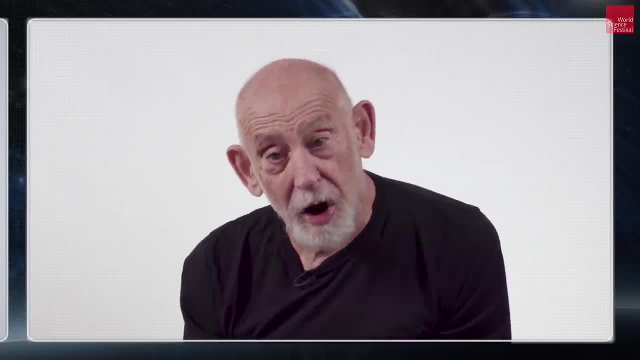 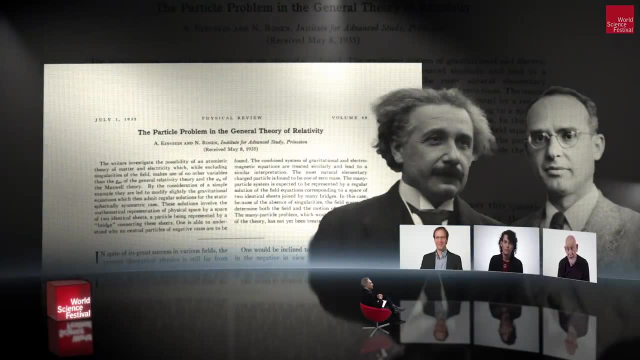 Okay, So then the other, that's the other 19.. You're talking about the other 1935 paper, The other 1935 paper, Exactly, The other 1935 paper. Yeah, I don't know what was on Einstein's mind, frankly. 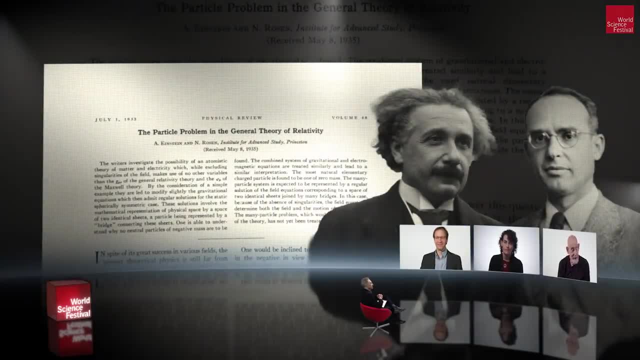 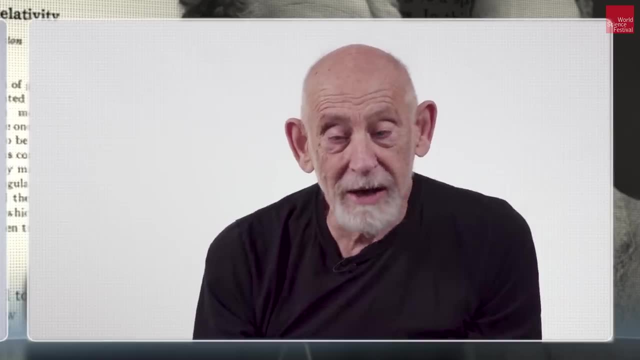 He didn't like black holes. I don't even know if he knew in that paper that he was talking about a pair of black holes. I'm not even sure that it was actually Einstein who cooked up the solution that we call Einstein-Rosen. 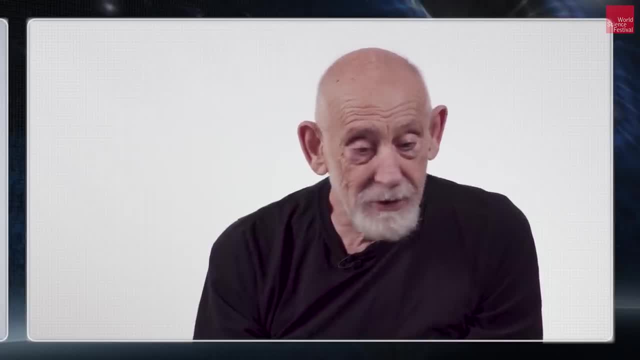 He, just as far as I can tell, he and Rosen- simply discovered a solution. He, just as far as I can tell, he and Rosen simply discovered a solution of the Einstein field equations, which contained this wormhole connecting different regions of space. 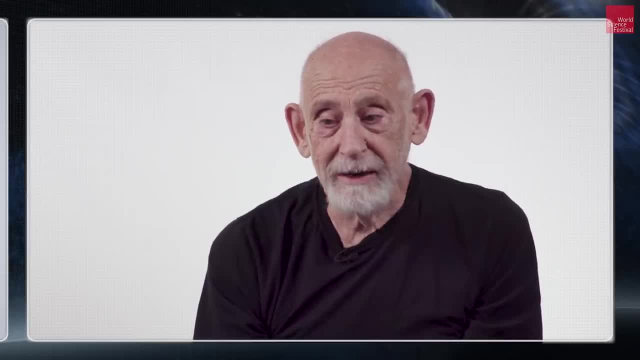 Yeah Yeah. It connects two distant points of space with a tunnel, with a short tunnel. It's as if you could Had a tunnel between New York and San Francisco or New York and Palo Alto, but if you go in the tunnel it's only a mile away. 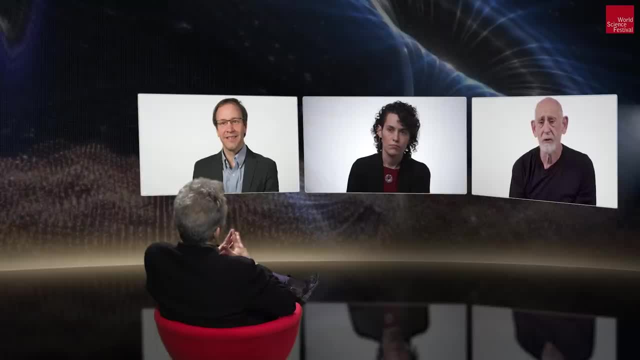 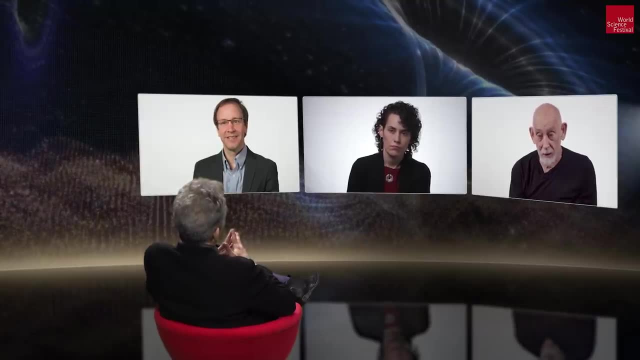 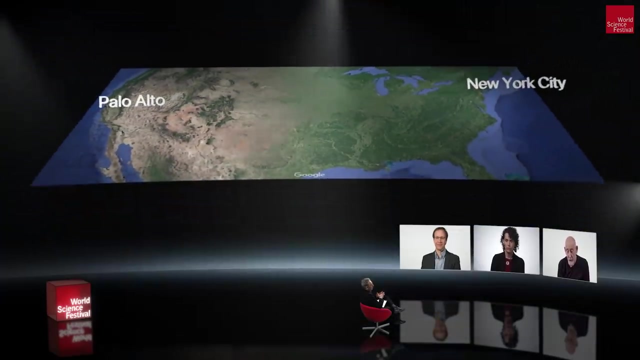 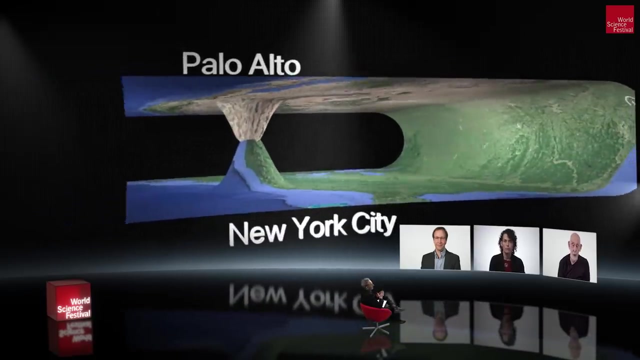 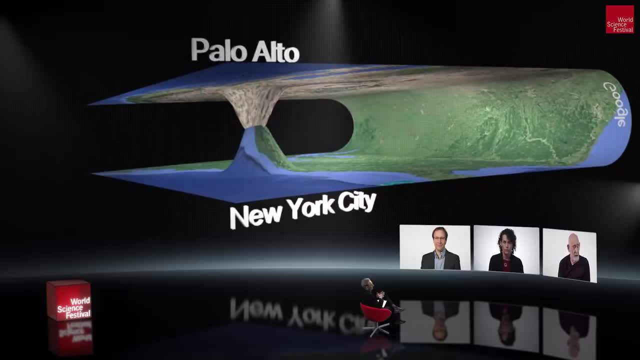 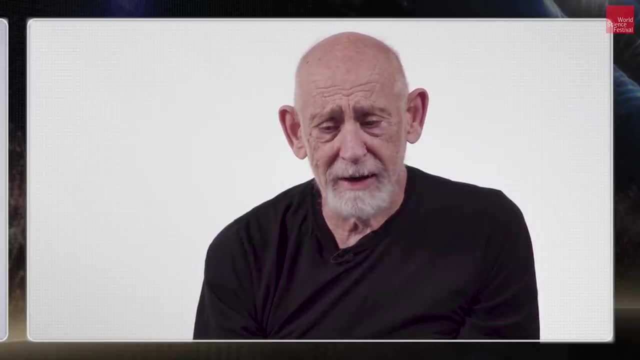 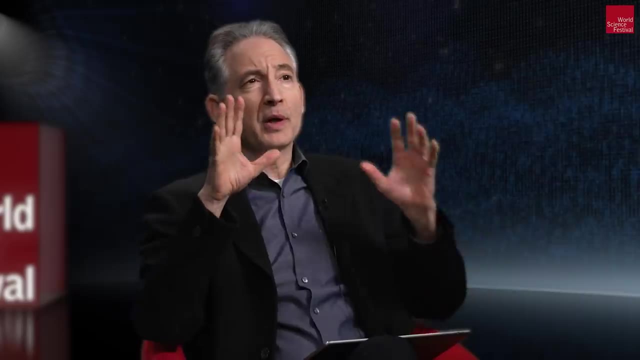 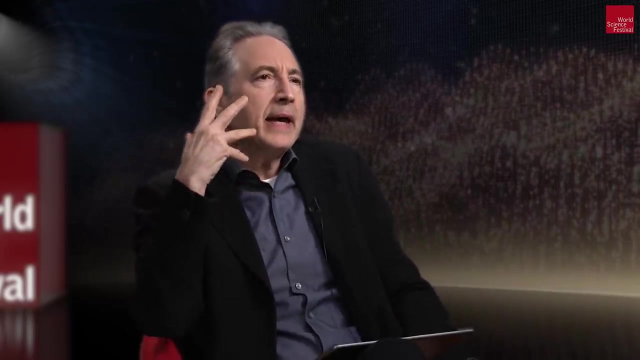 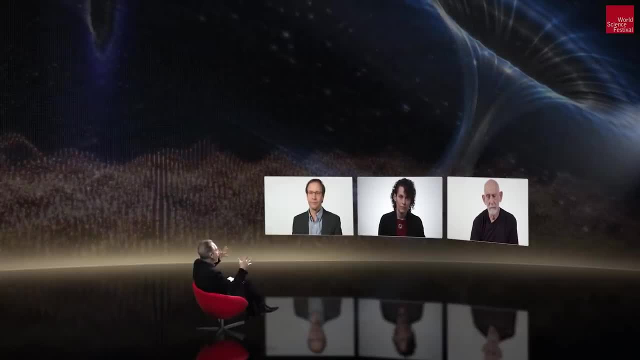 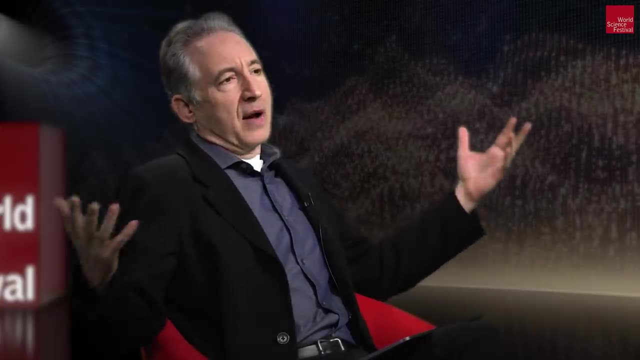 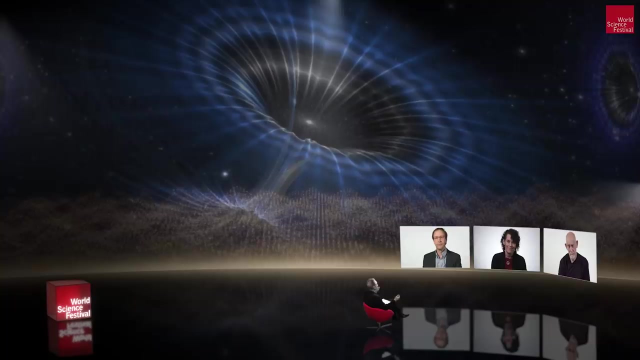 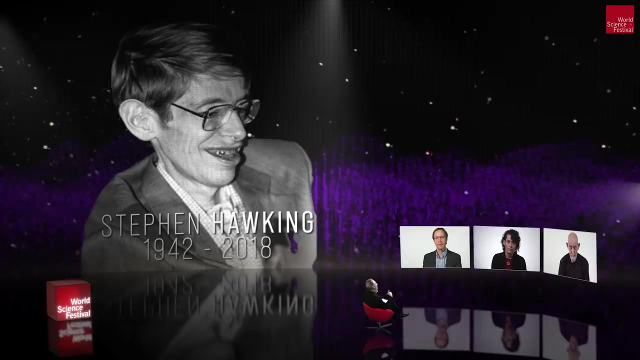 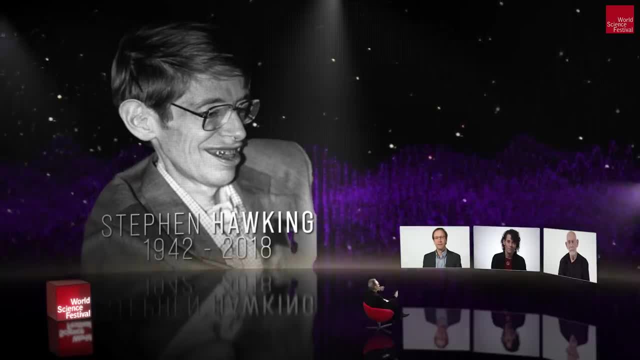 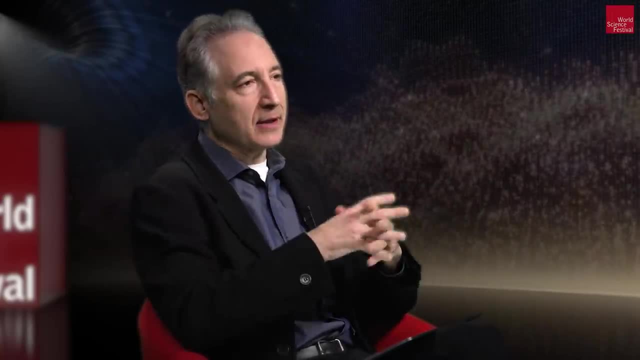 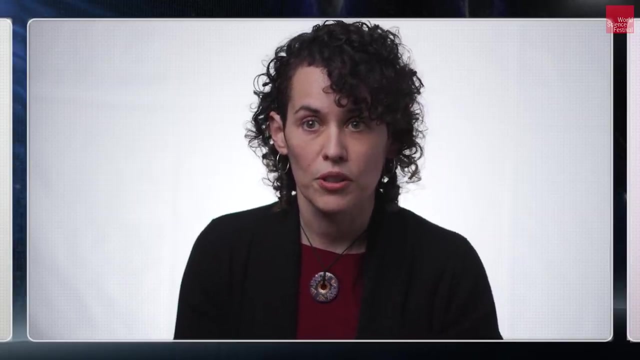 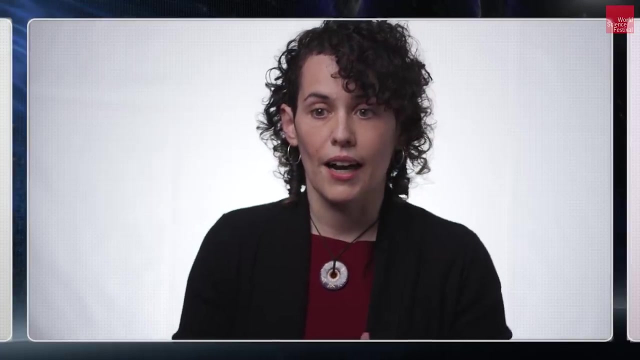 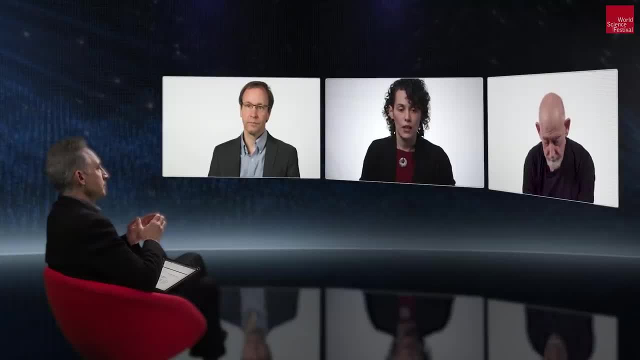 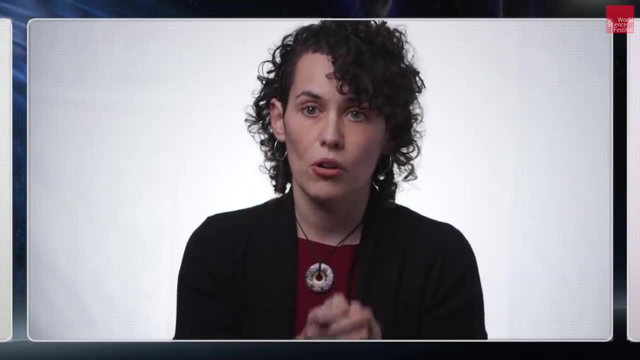 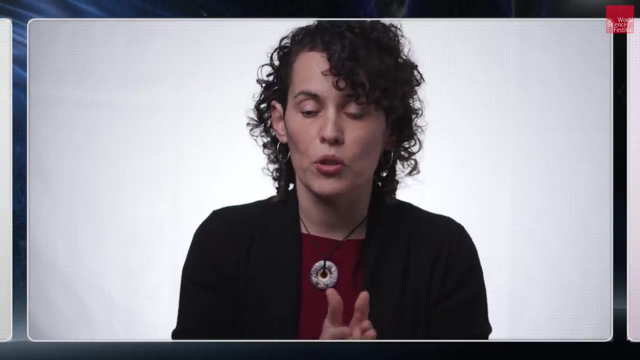 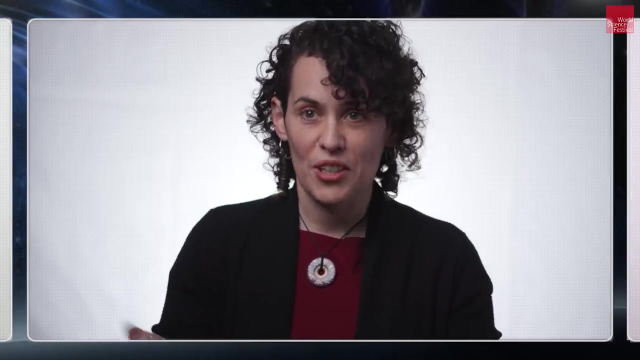 Yeah, Yeah, Yeah, Yeah. simplified version of thinking about it, that is that in this quantum field theory, we allow for the creation of particles- This is when we consider quantum mechanics applied to fields- and that you have a more complex theory. 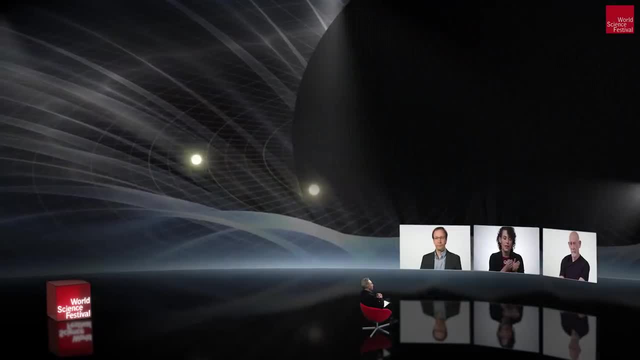 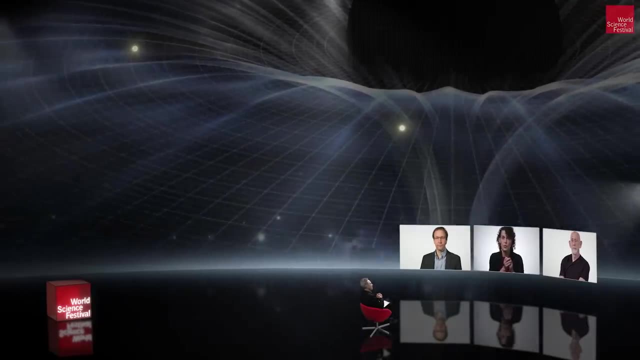 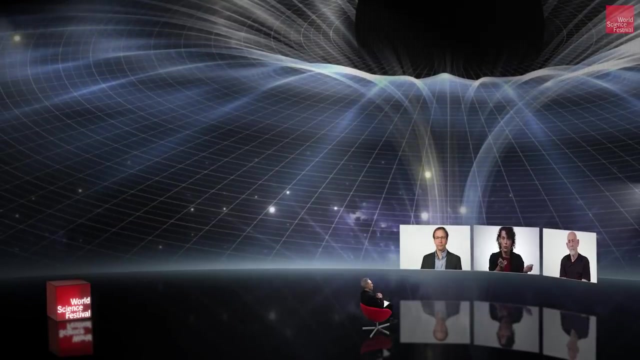 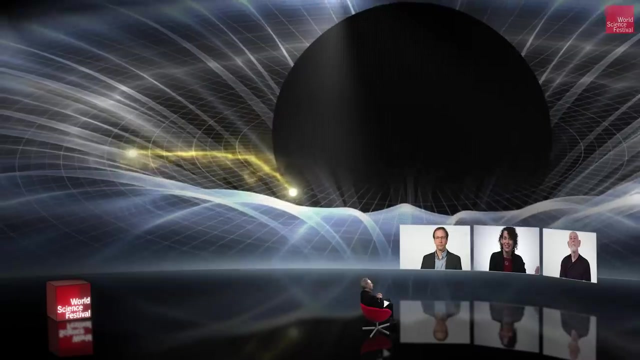 In this case you allow for this creation of particles. so it can be the point that this creation of particles takes place at the horizon of the black hole, So then one of the particles falls into the black hole and the other goes outside, the black hole, being these particles entangled, as we have been discussing before. 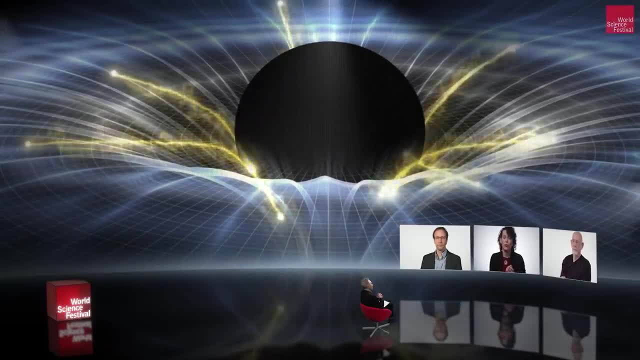 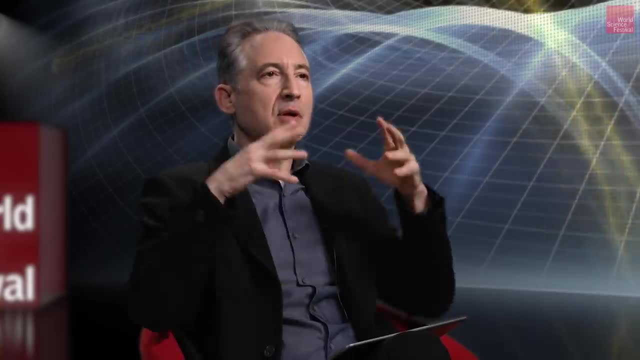 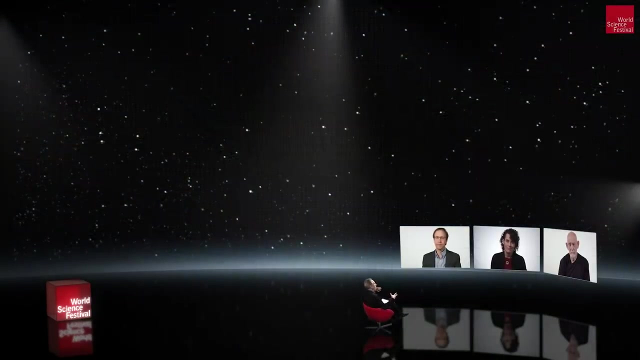 And in this case, what you have is like: in the end, what you find is that there is some radiation emitted by the black hole, Some quantum radiation, Right? so just to summarize those important points: according to quantum mechanics- pairs of particles- they can materialize in empty space and although in ordinary empty space, 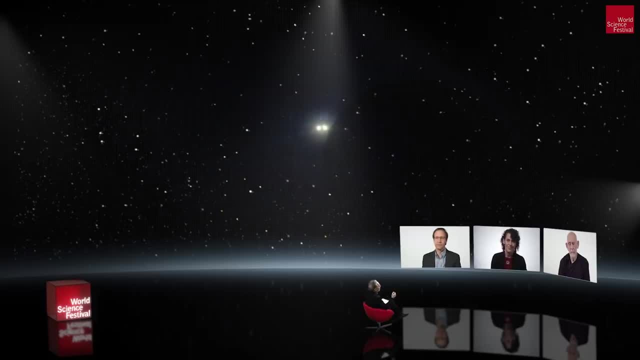 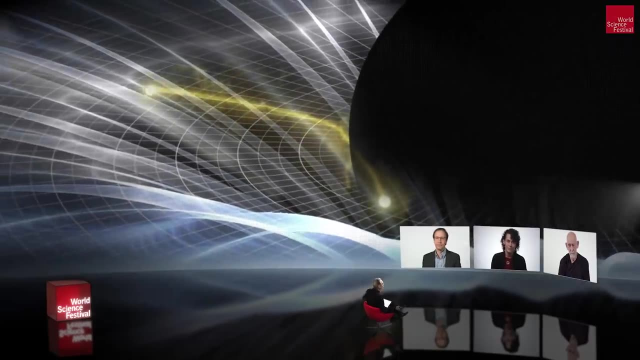 those particles would then quickly collide, annihilating one another. near the horizon of a black hole, one such particle can fall in, leaving its partner free to fly off, to radiate away into space And, as you also rightly pointed out, Anna, this radiation brings entanglement into the 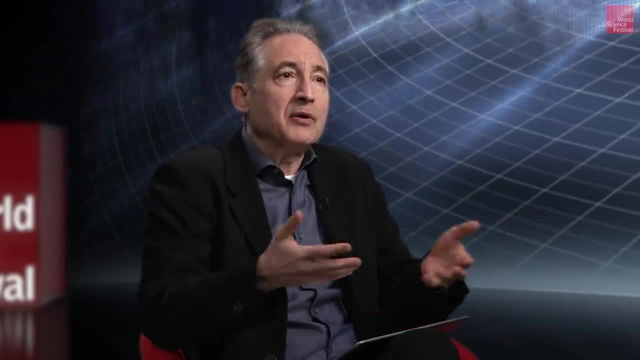 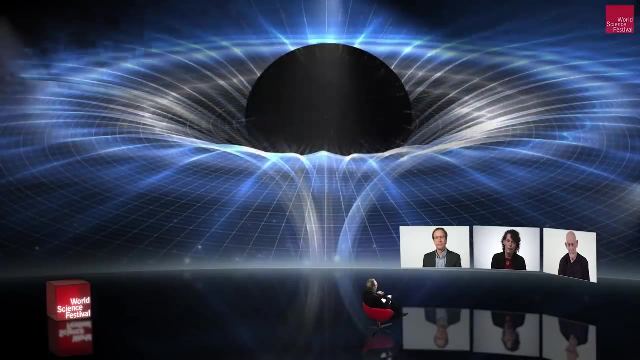 black hole story, because those pairs of erupting particles are entangled. that's a point we're going to come back to in just a moment. but first, Mark, once we learn that black holes radiate these particles that Anna is making reference to, that there's actually stuff. 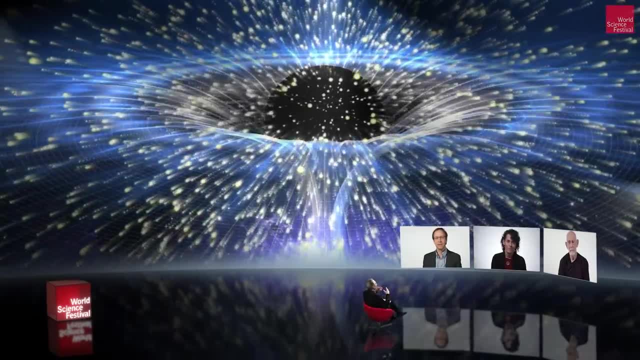 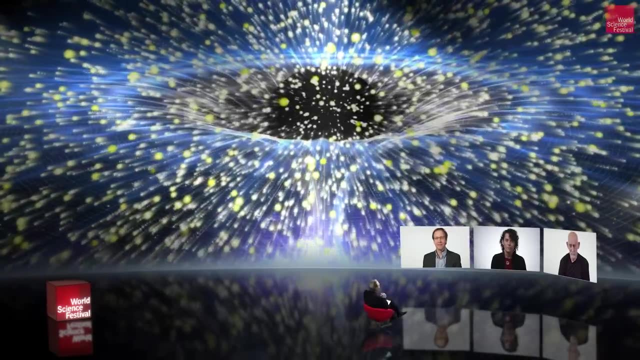 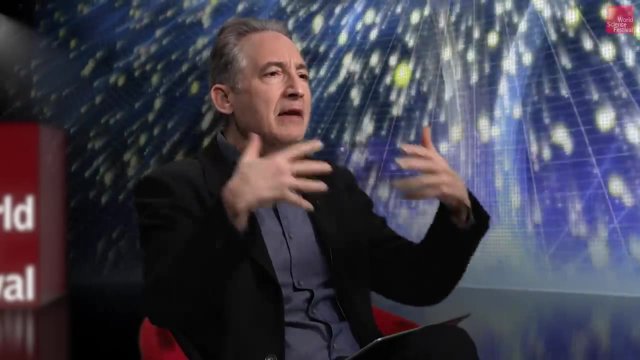 that in some sense is coming out from a black hole. well, that stuff, it takes away energy and so the black hole gets smaller in the process and will ultimately disappear. and this raises a deeper question. It raises a deep concern because a fundamental principle in physics is that information is. 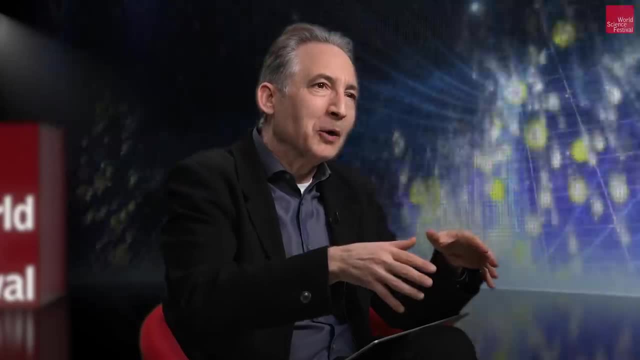 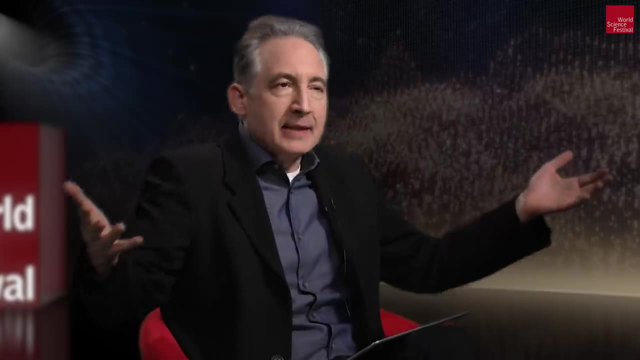 never lost. Now, when something falls into a black hole- right, if it's a book, an iPhone, whatever- you might have imagined that the information contained in the object is not lost. it's just inaccessible, since it's now inside the black hole itself. 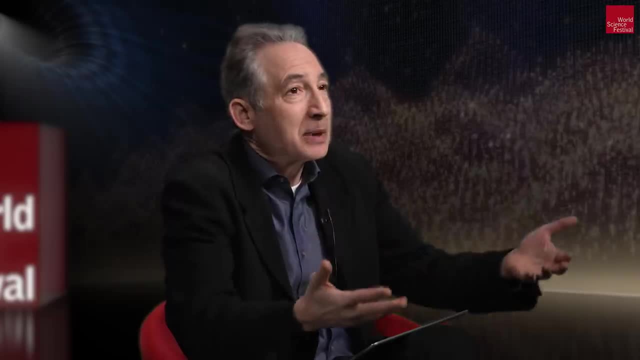 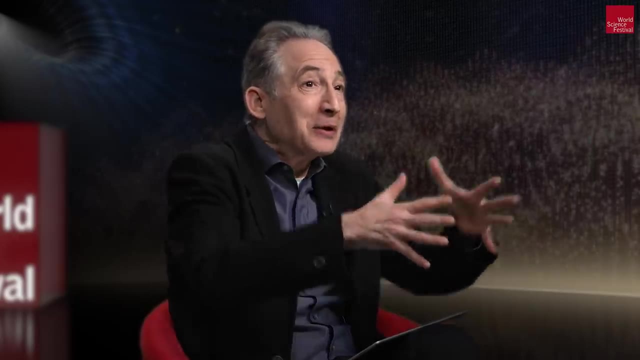 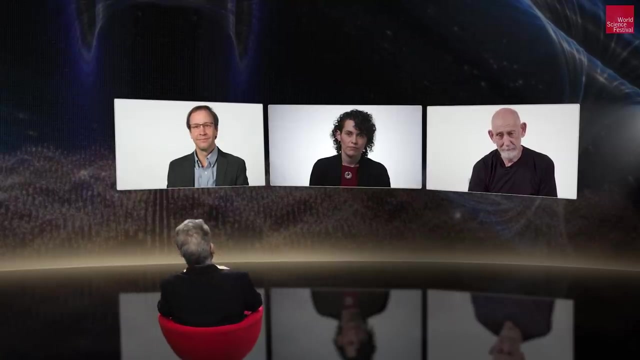 But when we learn that black holes radiate and ultimately disappear, that vision no longer works. We can't hide the information forever, so the radiation better carry that information back out with it. But at first blush it doesn't seem that the radiation does that, giving rise to the so-called 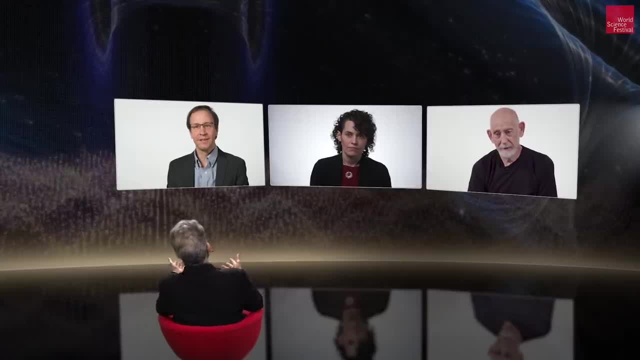 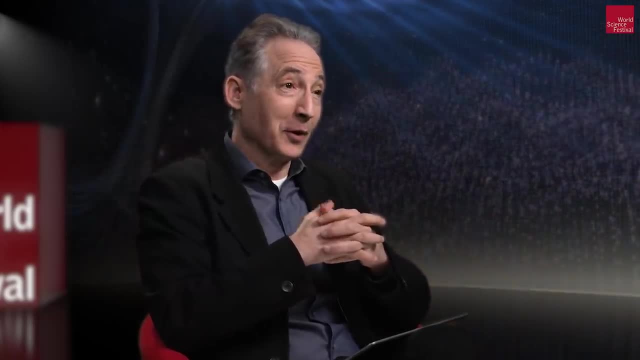 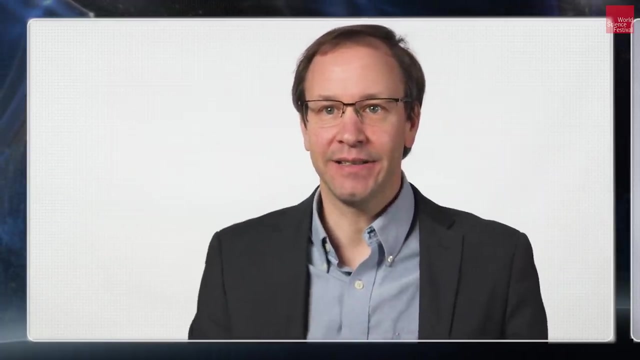 black hole information problem or black hole information paradox. So, Mark, can you tell us about that and then we can discuss how Lenny's going to solve it for us? Yeah, So with this black hole radiation? Yeah, So this is something that Anna described. so you've got your black hole. 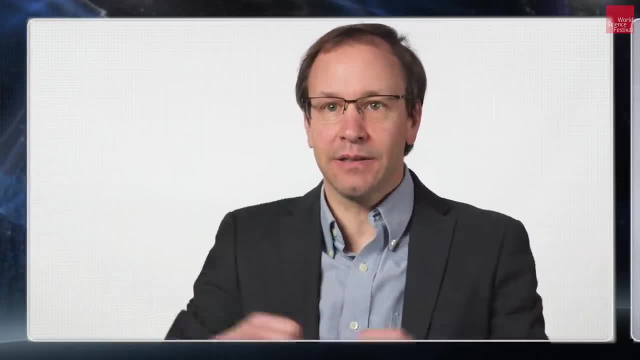 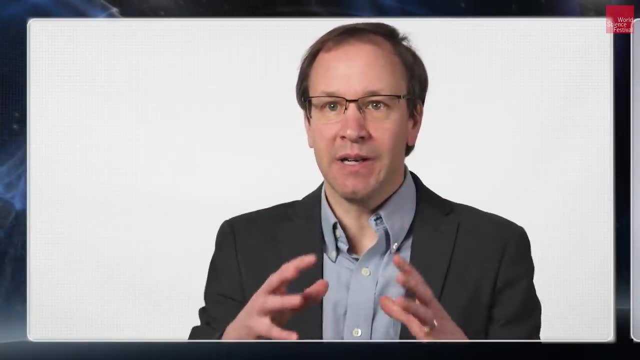 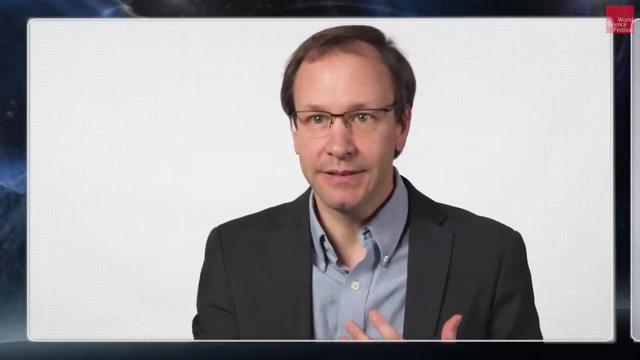 What it looks like if you were to measure what's coming out of the black hole. it looks just like, say, an object with some temperature emitting the thermal radiation corresponding to that temperature. And one of the interesting things about the detailed calculation that Hawking does is: 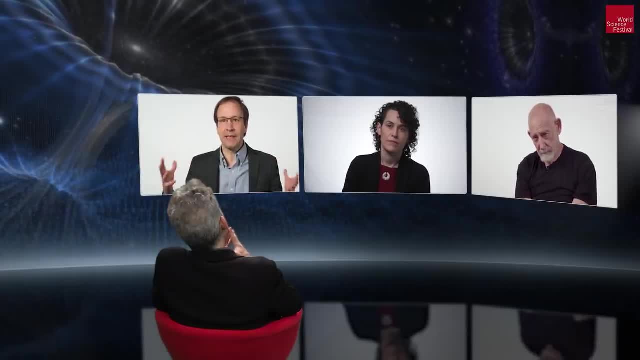 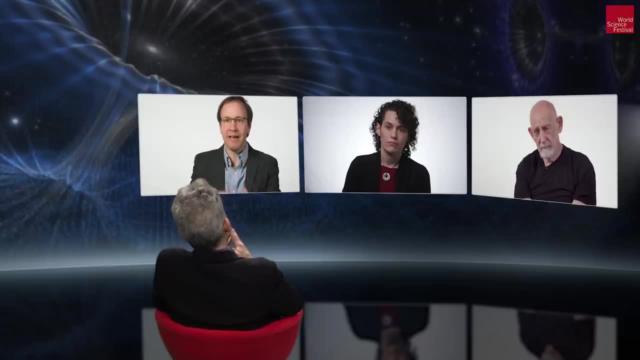 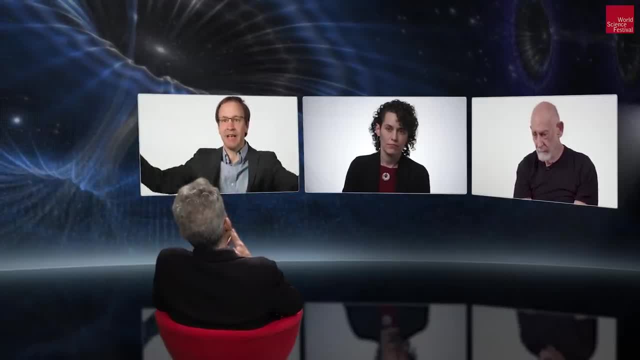 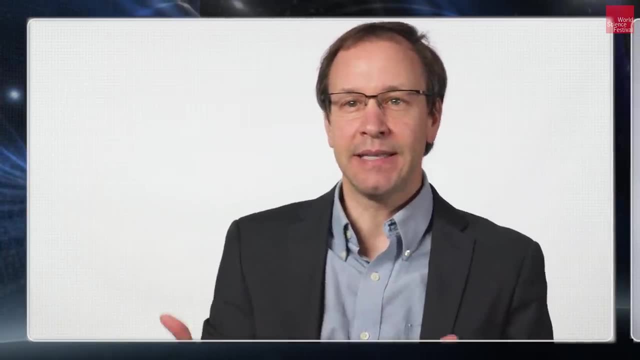 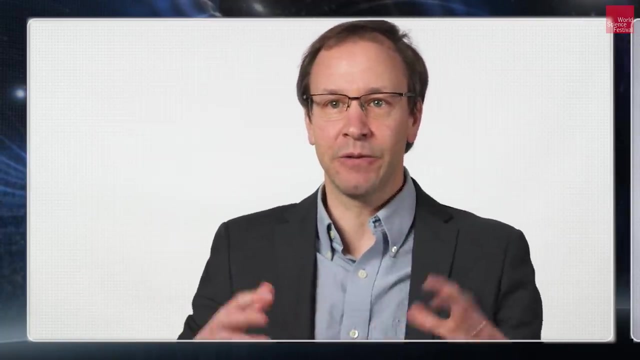 black hole in the first place, It just is the same kind of purely random thermal radiation coming out, And so it seems that you lose information about what formed the black hole, And that's kind of in conflict with a basic assumption or a basic property of quantum. 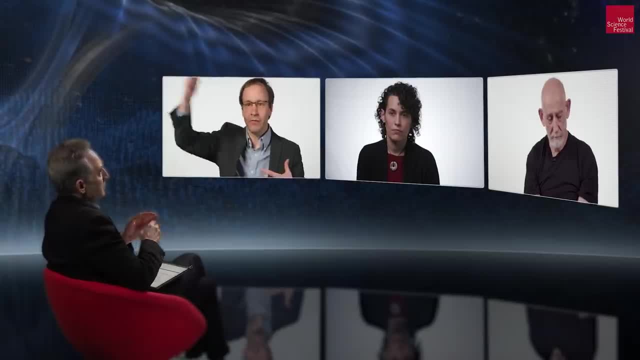 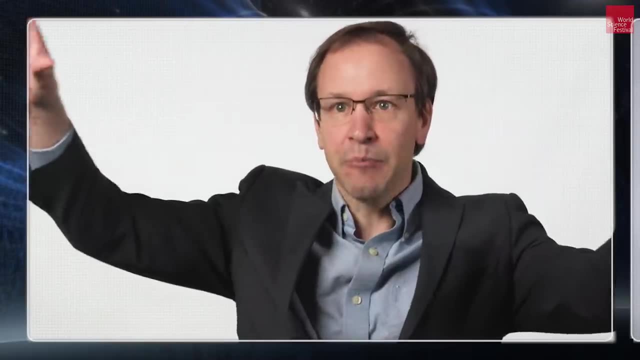 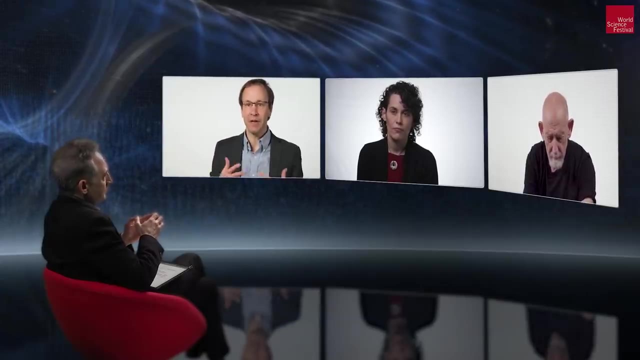 mechanics. In quantum mechanics you could always sort of run the clock backwards. You could recover what it was, that was the initial state given if you had complete knowledge of the state later on. And so there was a tension there that if you completely accepted Hawking's calculation, 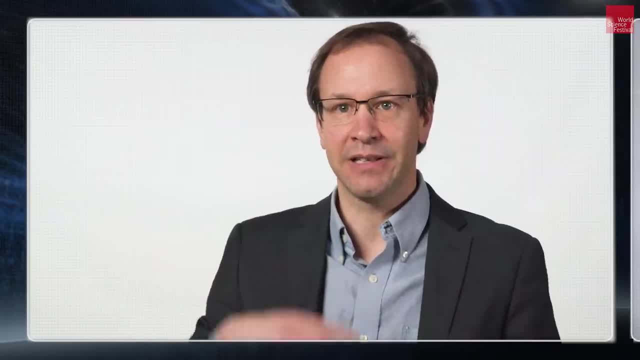 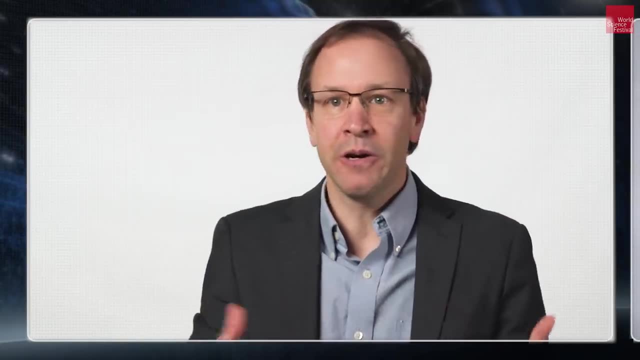 then there seems to be a tension with quantum mechanics, And so you could decide: OK, well, you need to modify quantum mechanics if gravity is going to be a part of it, or you have to come up with some more creative And brilliant idea. 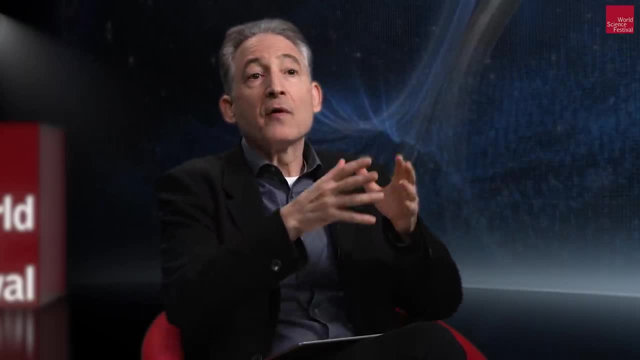 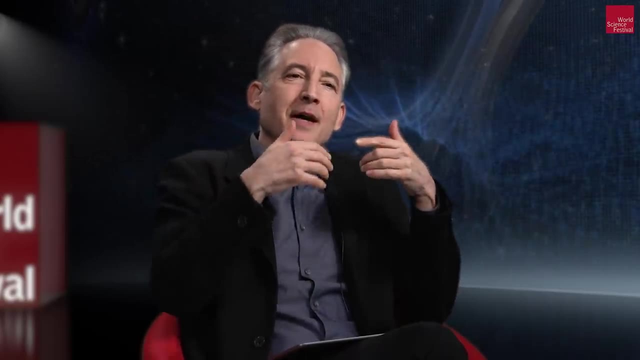 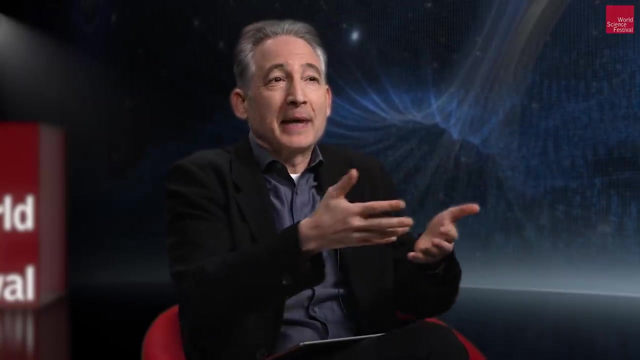 So, Lenny, this loss of information regarding what falls into a black hole was a potential blow against all the hard-won understanding, because, according to quantum mechanics, no information is ever lost. According to quantum mechanics, a detailed form of radiation coming out of a black hole 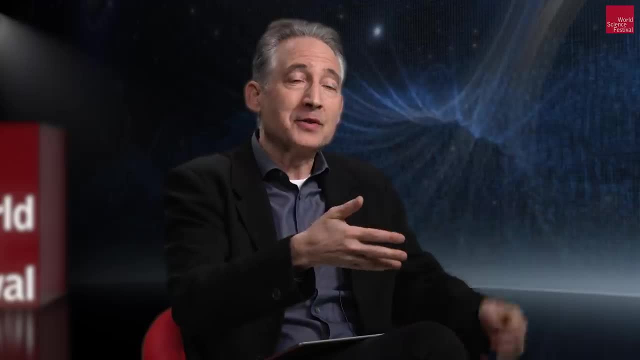 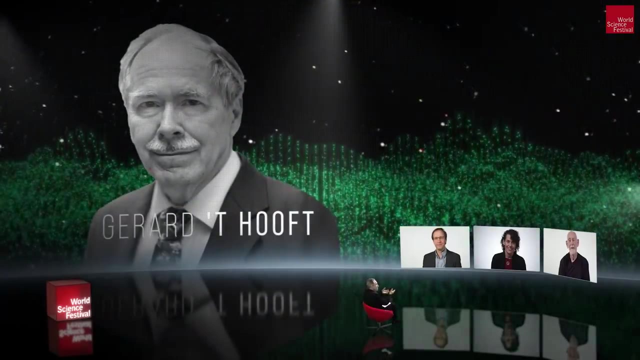 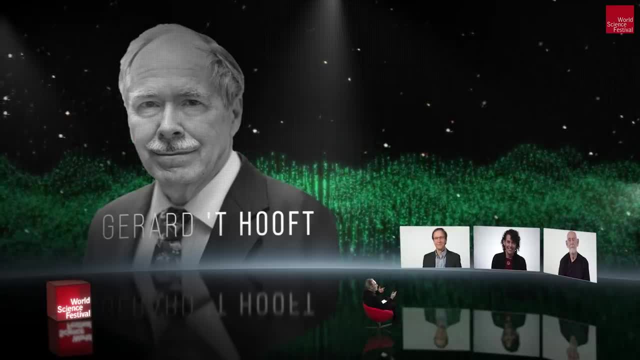 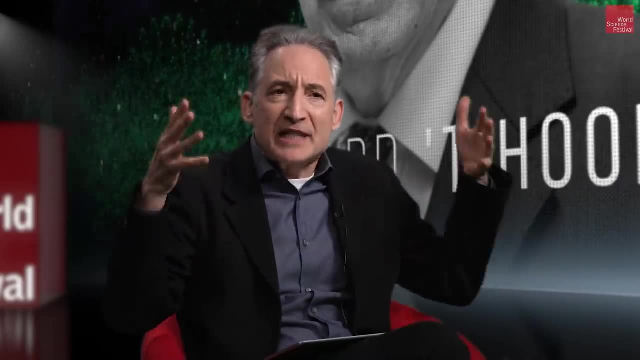 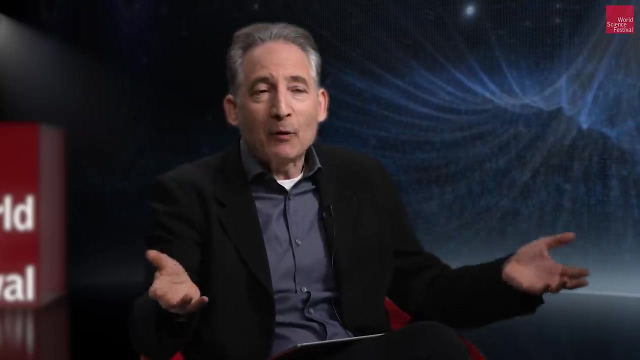 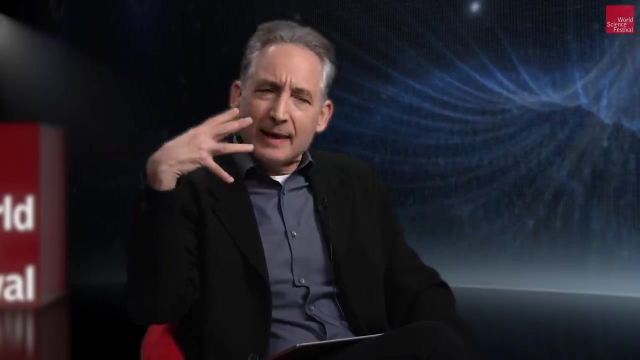 You both were having none of it, And over the course of many years, you both developed your own versions of similar arguments, claiming that information is not lost, making use of incredibly strange but wonderfully powerful idea known as the holographic principle. So tell us how that goes, and I gather that string theory was an important 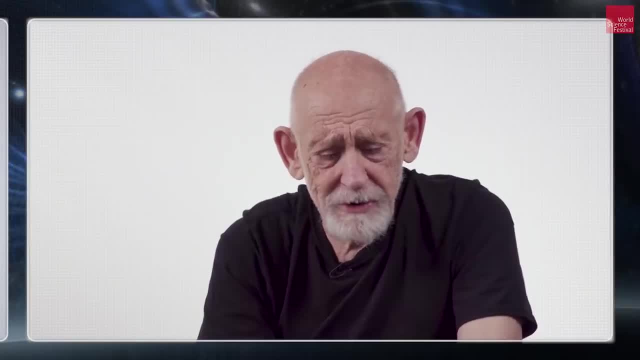 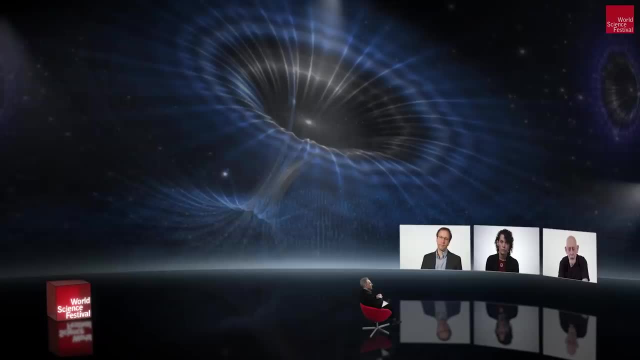 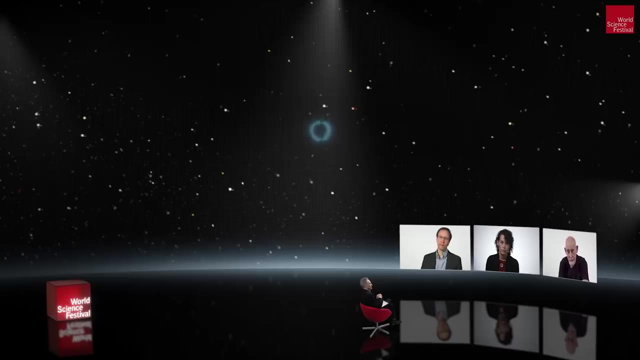 inspiration in your thinking here. Okay, I had had some experience in the field of string theory and there was one thing that had always puzzled me about string theory: The more carefully you look at a quantum string, the more precision that you bring to bear on the measurement of the 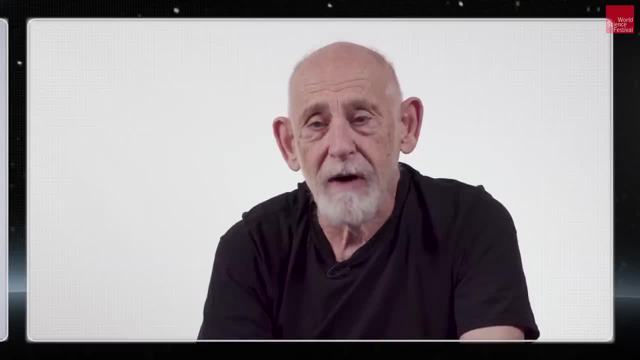 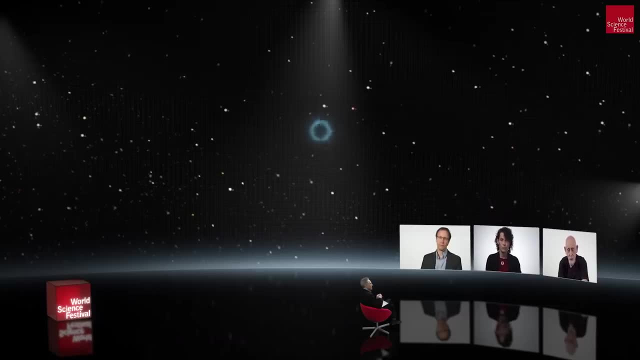 quantum string, the more you will find that it's spread out over all of space. If you look at it casually, with not too great a resolving power, you'll find the string localized. a little string, a little particle, you'll find it localized in some localized place. If you look at it more, 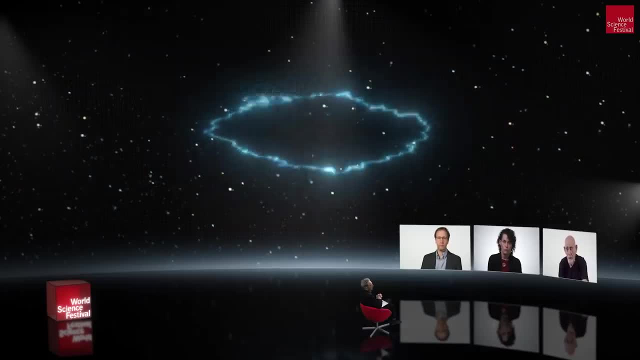 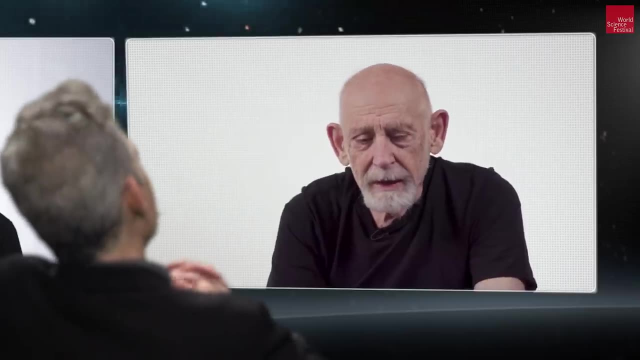 carefully, with more precision, you will find out that it's spread over a bigger distance. If you look at it really carefully, you'll find out that it's spread out over a larger distance. It occurred to me that when a particle falls into a black hole, somebody watching it from the 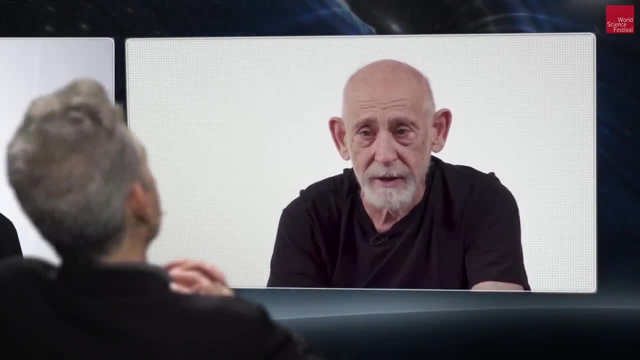 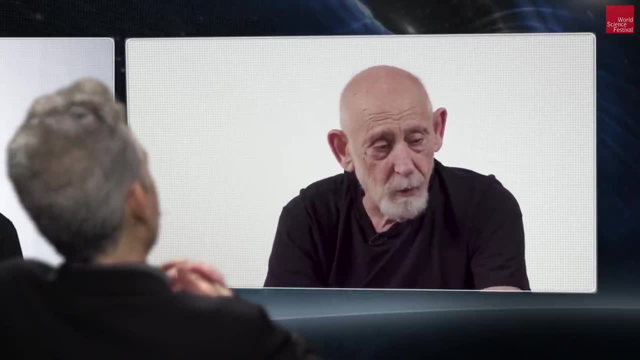 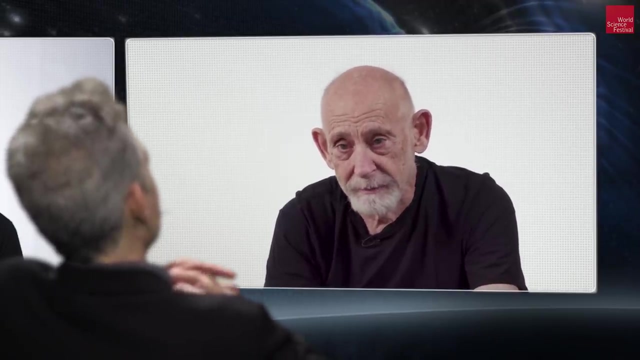 outside. because, Because everything slows down As a thing falls towards a black hole, its internal motions slow down. Somebody watching it from the outside gets to see it with more and more precision. because it slows down, It's like looking at an airplane propeller If it's going too fast. 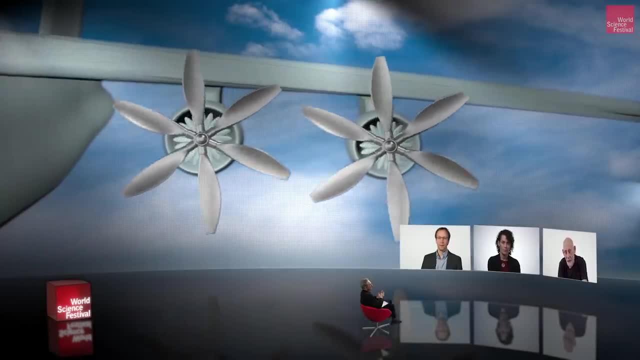 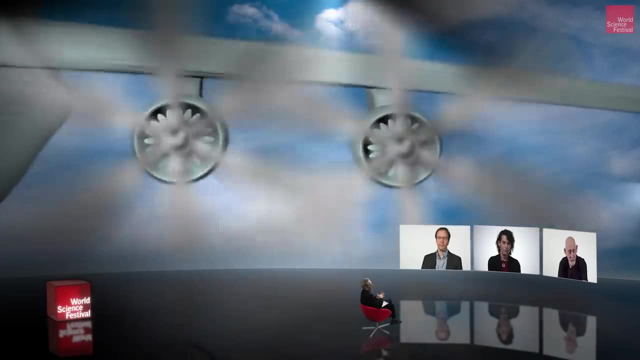 you can't see what it is If it's slowed down. you can get a look at it and see what it is and see it in more detail. Same thing with this vibrating string: As it falls into a black hole. somebody watching it would get to see it with better and better. 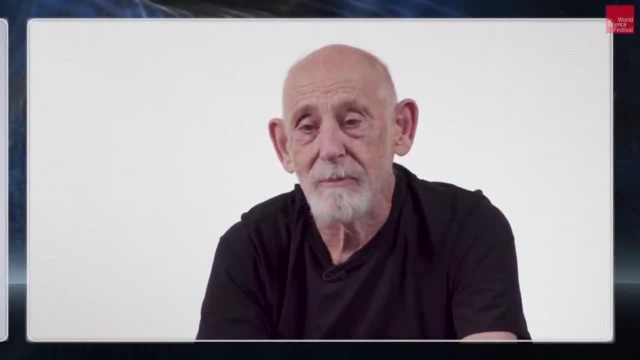 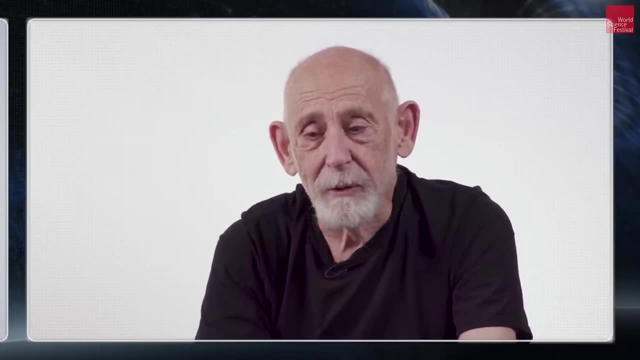 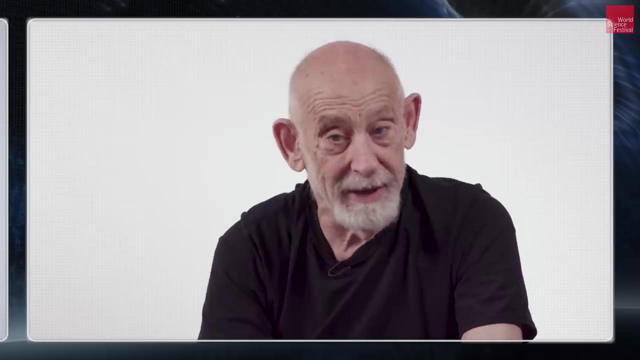 resolution, And therefore we get to see it spread out more and more in just such a way that, instead of falling into the black hole, it would get spread out not only over the horizon, but spread out way out to infinity. And so this preyed on my mind. I got to thinking about it. 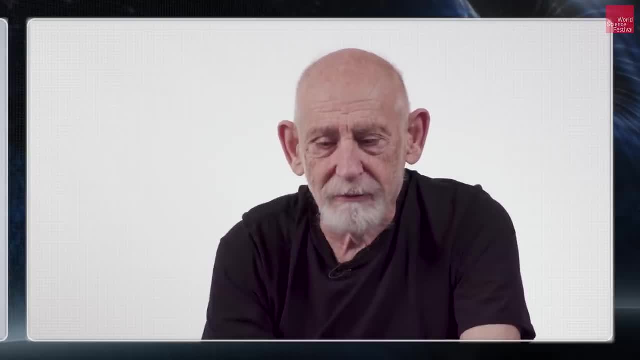 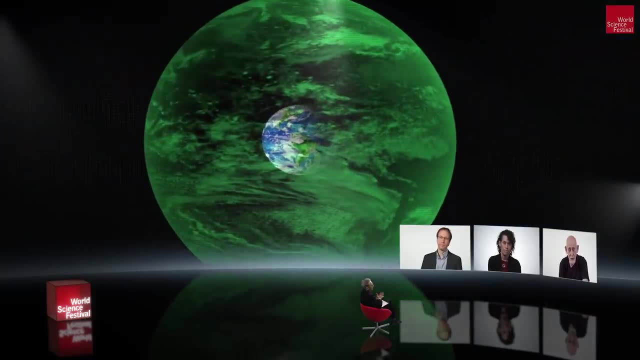 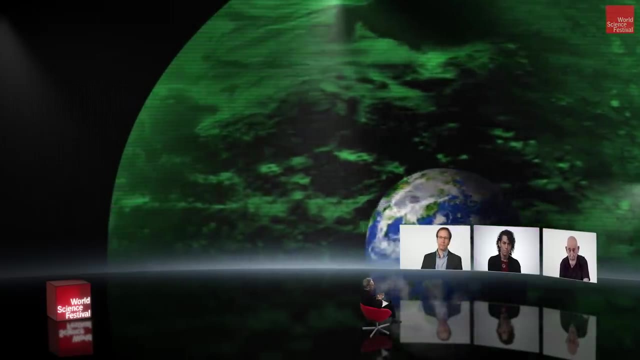 And I had the idea that somehow the fundamental degrees of freedom in string theory are stored very far away And that the relationship between the actual things that you see and the actual storage of information was very much like a hologram At about the same time, maybe even a 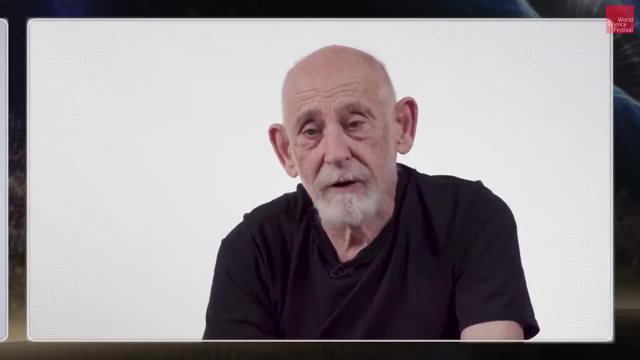 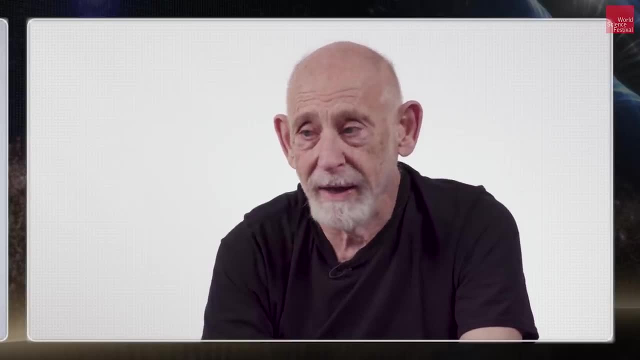 little bit earlier, my good friend at Tuft had a very similar idea Again, that the information in a system, any system, is stored very far away. And so I got to thinking about it, And so it was stored far away, at the boundaries of the world. A very weird idea, an extremely weird idea. 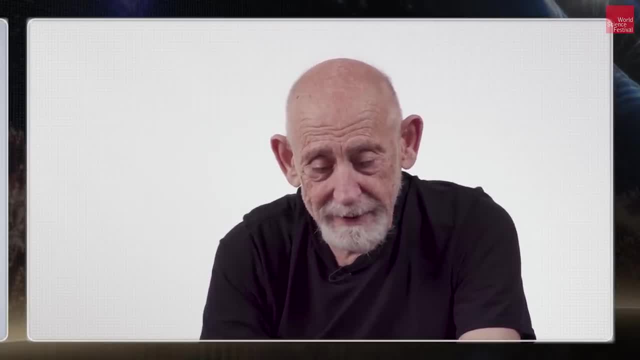 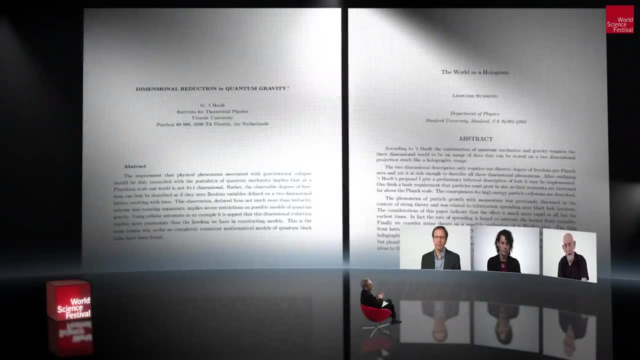 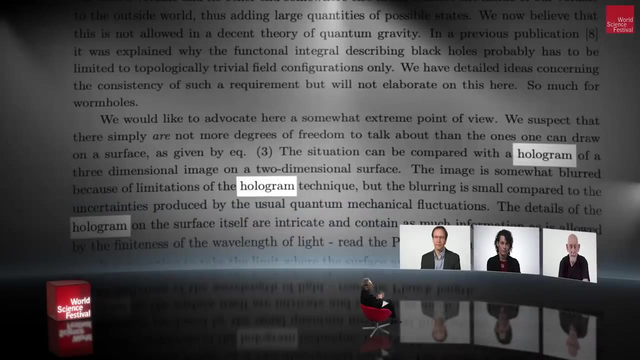 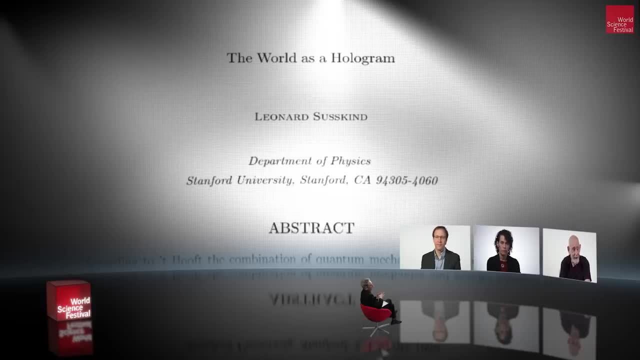 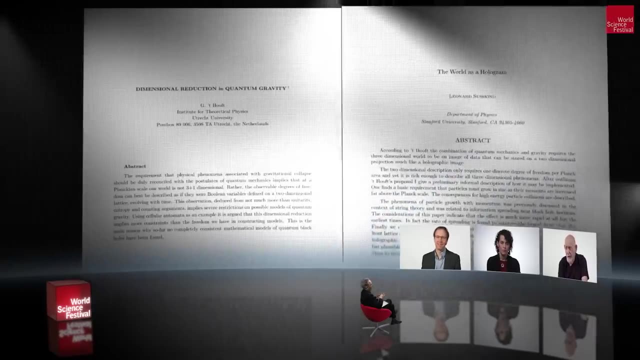 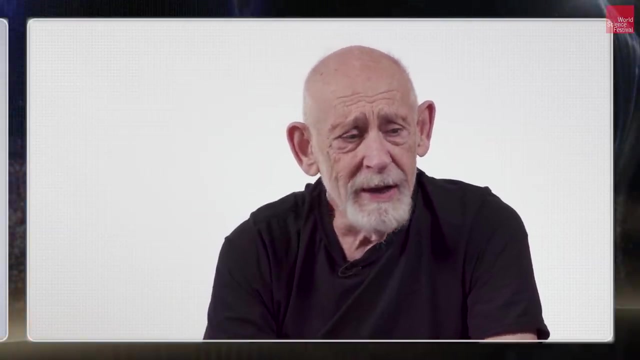 I got lost. People didn't notice it for some reason. The bold title The World as a Hologram, I think, caught a few people's attention at the time. So the idea was that information never really falls into the black hole. It's always stored far away, But it's only the kind of 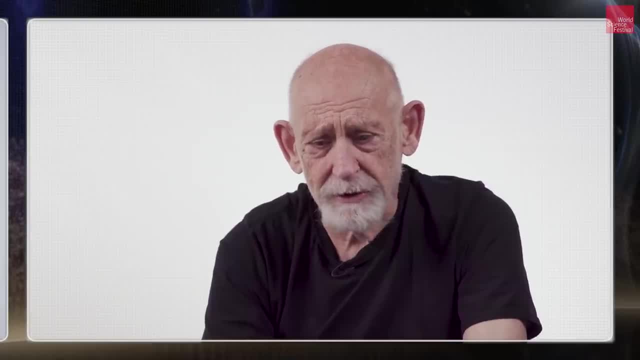 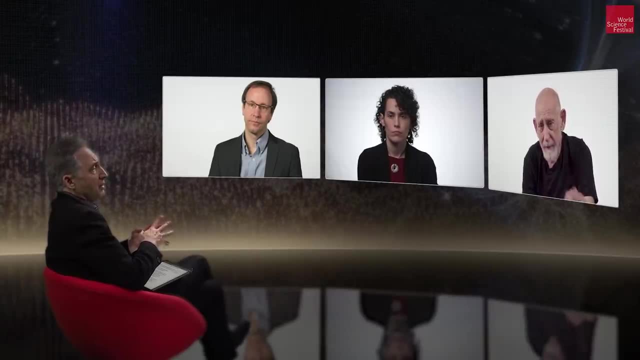 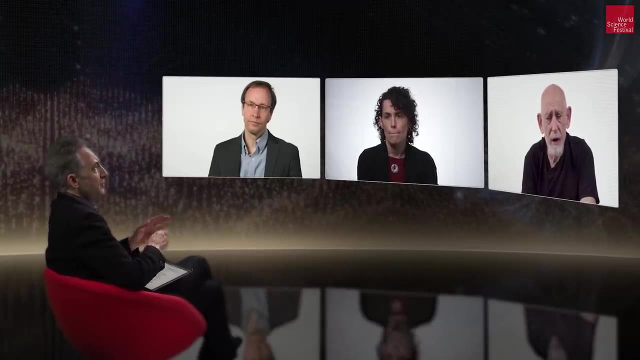 image of this information that falls into the black hole. And can we think of the information as being on the black hole, The horizon echoing with? I think that's one way of thinking about it. But you can even go further than that. You can say: if you get enough resolution power, you will find that as you get better and better. 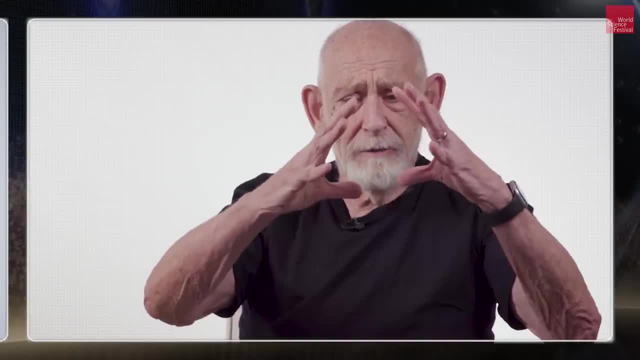 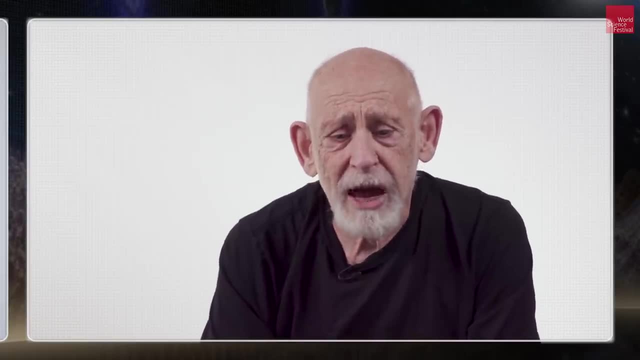 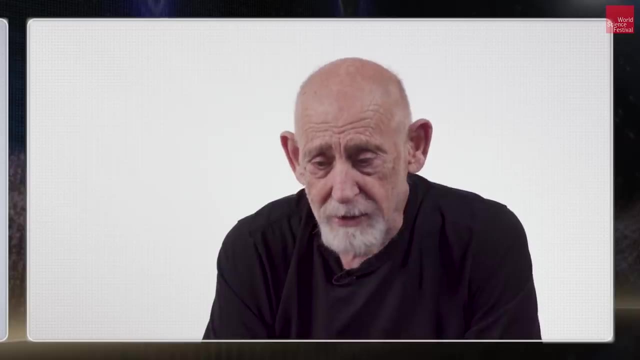 resolution power. it sort of hovers above the black hole to larger and larger distances away from the black hole. Where exactly is the horizon? That depends on how much detail you look at it. Where is the information? It again depends on what detail. 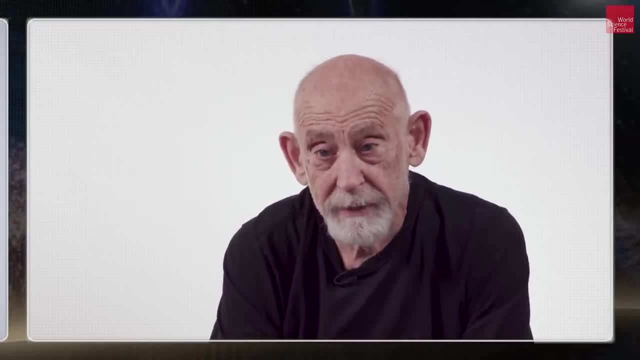 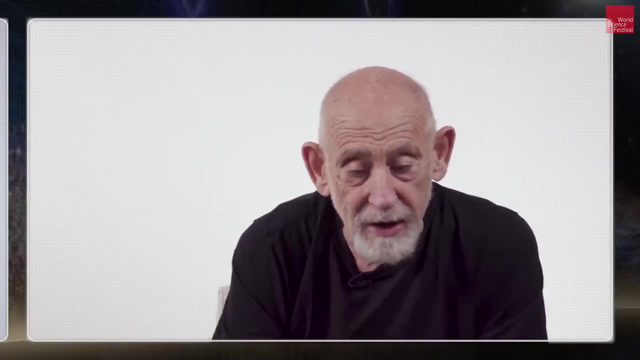 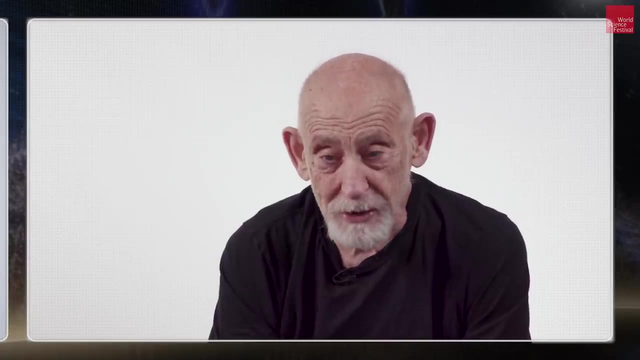 you look at it with your resolving power of your camera, the speed of your camera, if you like, It's not in the black hole. It's not on the black hole. Ultimately, it's out at the boundaries of space, wherever the boundaries of space are. 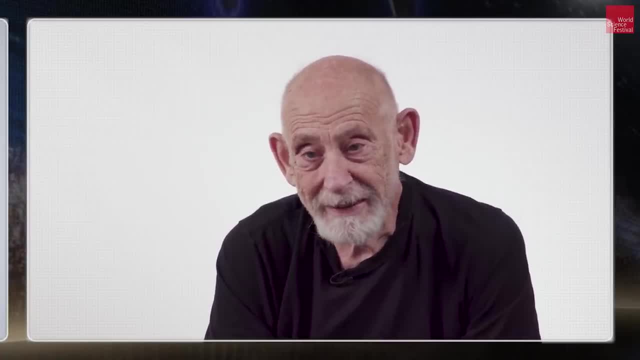 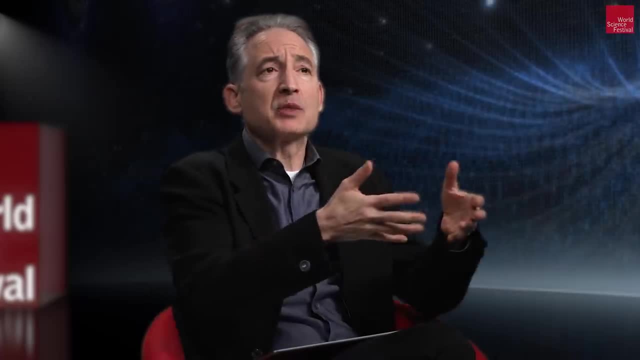 Now, does space have a boundary, Who knows? And so we come to a pretty wild state of affairs, which seems to solve the problem right. Yes, yes, The information regarding whatever object falls into a black hole is not lost because that. 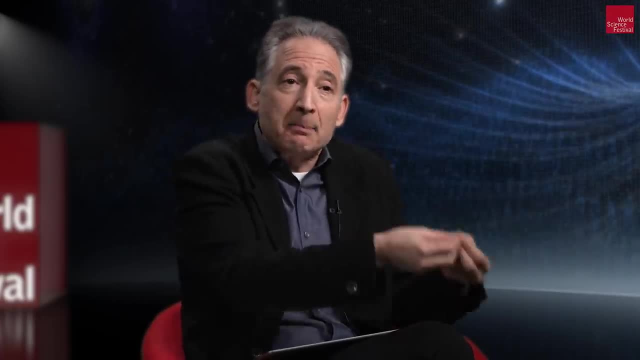 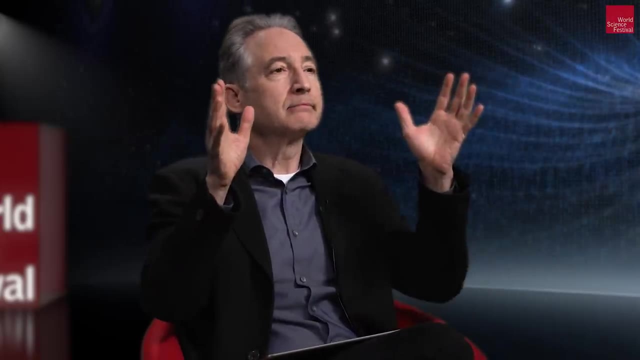 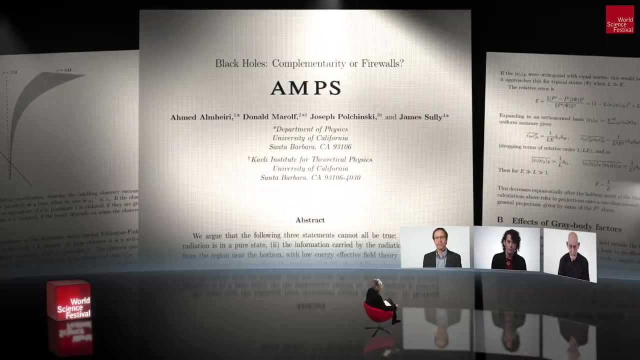 information gets stored holographically outside the black hole itself, which in principle means that the information is recoverable. Good, But then comes a paper in 2012 by four physicists- Almieri, Marl, Polchinski and Sully- a paper referred to in the field as AMPS. 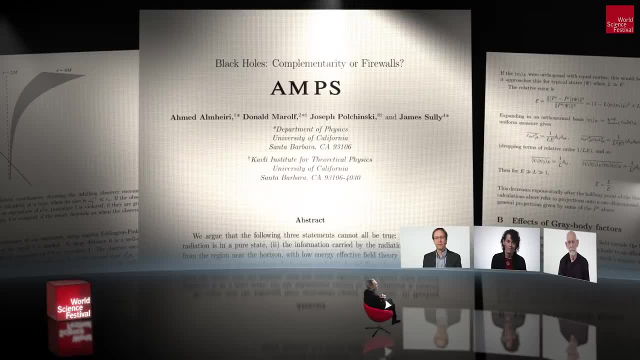 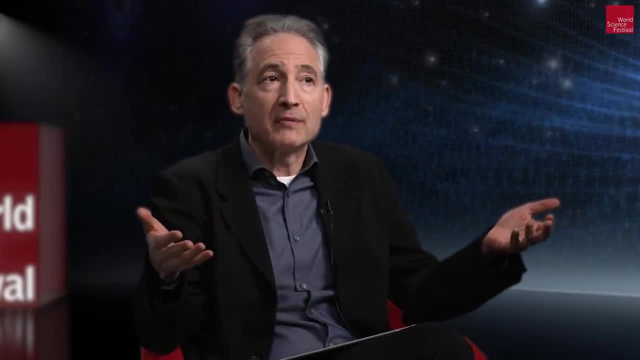 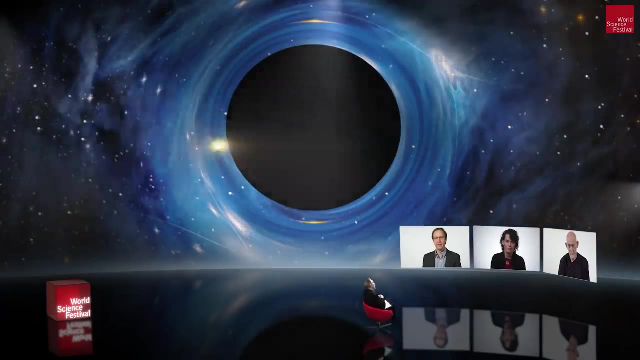 which, shall we say, shocked the community, And it has to do with the entangled nature of the Hawking radiation that comes out of a black hole, which, Anna, you alluded to earlier, Namely the erupting particles near the black hole's horizon. 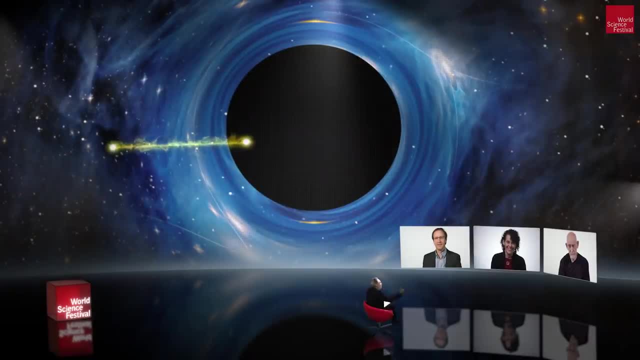 are entangled. But for the outgoing radiation to embody information about whatever fell in, that radiation can't be fully random. Instead, there also has to be entanglement between the early radiation, which is the black hole, and the black hole's horizon, And so 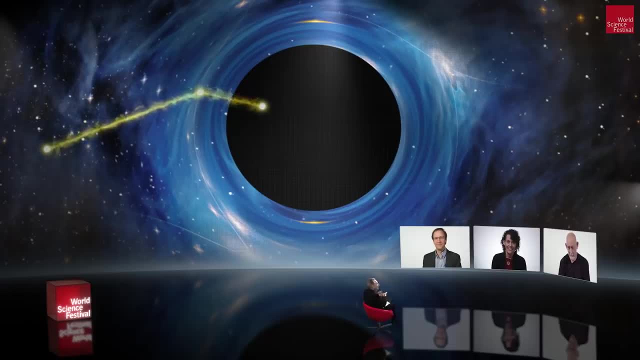 this is now traveled far from the black hole, and later radiation, which is still near the black hole itself, because only with such entanglement can there be information storage. Now for the problem that AMPS pointed out: quantum mechanics doesn't allow such three-way entanglement cheekily. 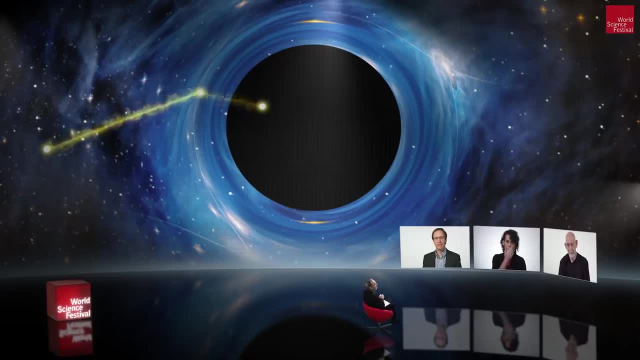 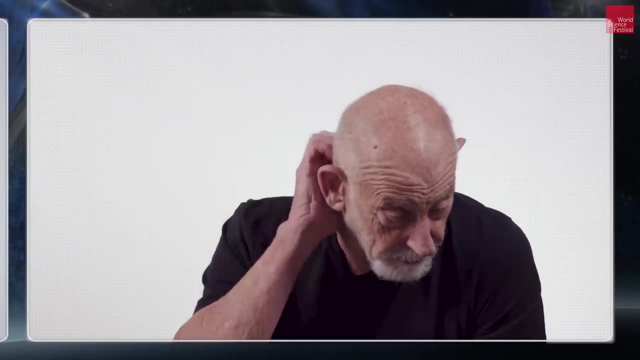 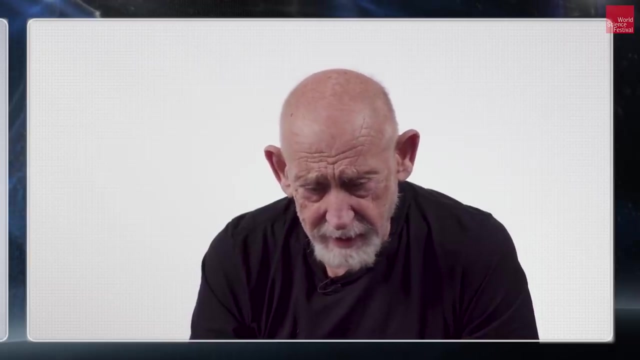 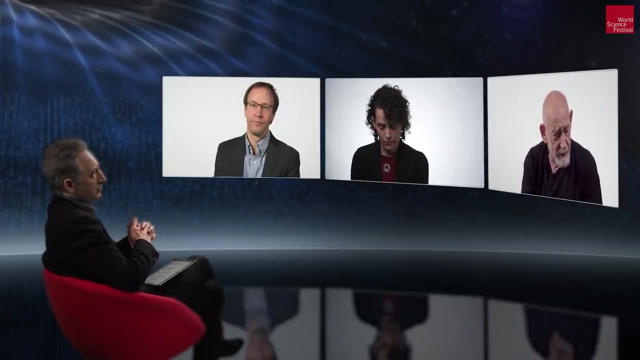 referred to in the field as the monogamy of entanglement. So, Lenny, what to do? So Mark's work was very, very instrumental in this. Now, before yes, again, I have to bring up another person on this paper that I wrote that had to do with the two 1935 papers. For once in my 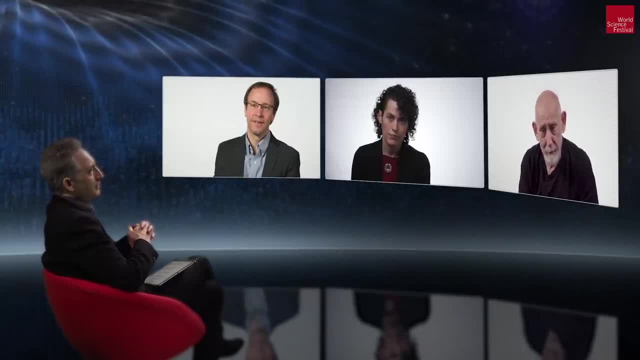 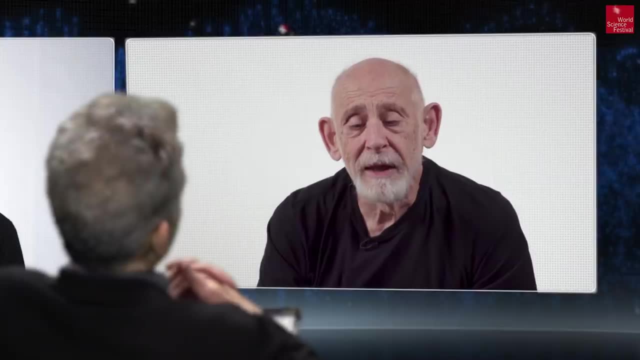 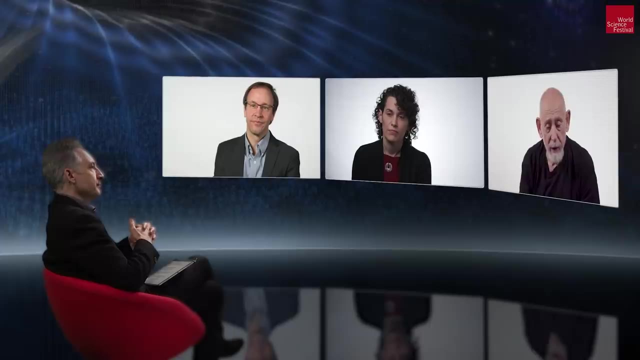 life. I was very definitely the second author on a paper. The first author was Juan Maldacena, who had been thinking about very related things a long period of time, And I should mention that before we go any further. Okay, So what was I? 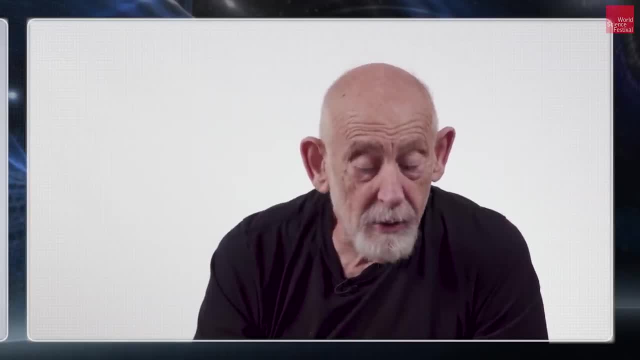 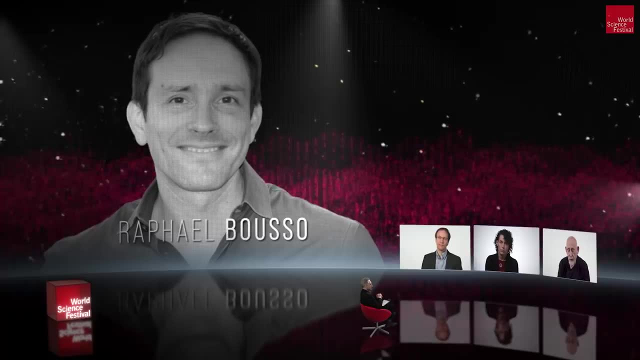 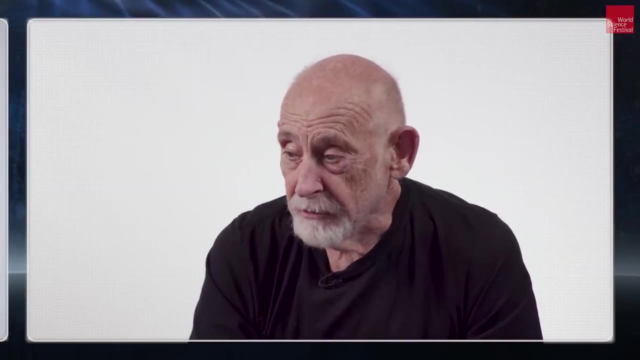 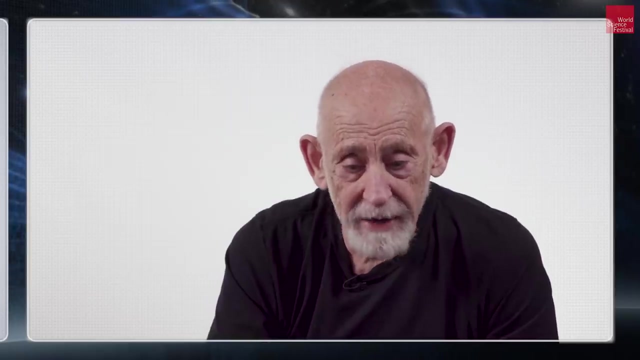 thinking I had. I, and also, I think, Rafael Busso, had the following idea: The information right behind the black hole, right behind the horizon of the black hole- let's see how to say this- right, the exterior of the black hole cannot both be entangled with what's just behind the horizon. 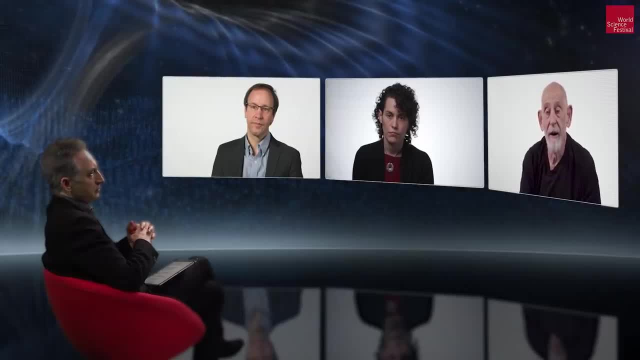 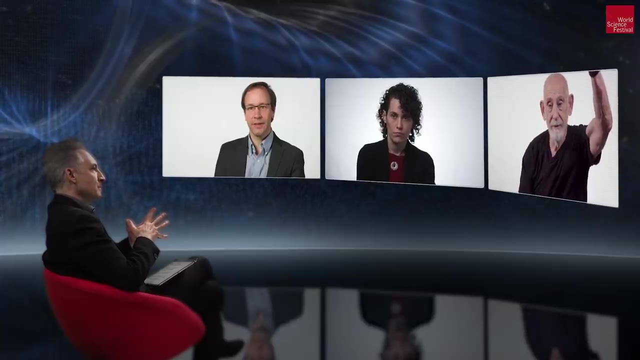 and the Hawking radiation unless the information right behind the black hole and in the Hawking radiation are the same thing. Now that sounds again crazy. How can? what's right behind the black hole? here's my black hole over here. Okay, The Hawking radiation is miles and miles, and miles. 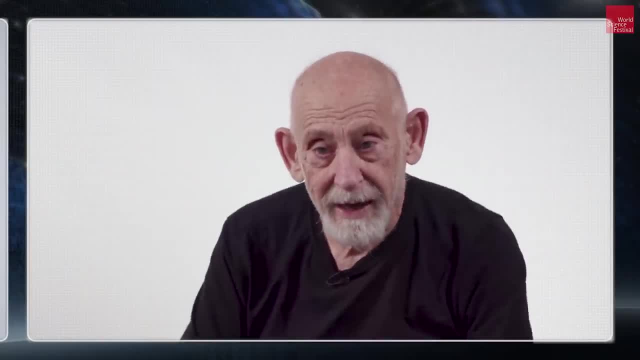 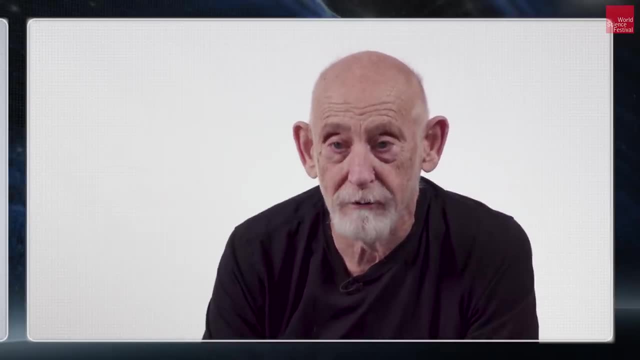 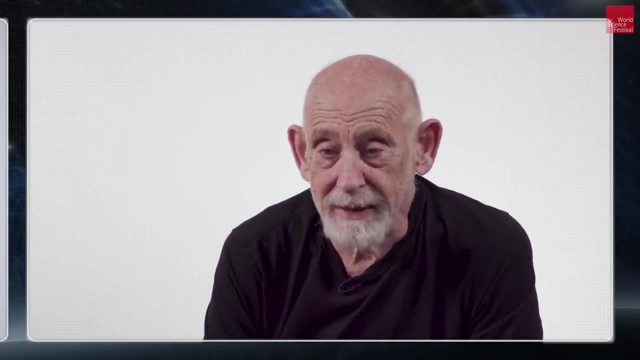 No, Many, many, many light years away. How can the information of what's right behind the horizon of the black hole be the same thing as the information in the Hawking radiation very, very far away? Nevertheless, I said it must be true. It must be true that the entanglement 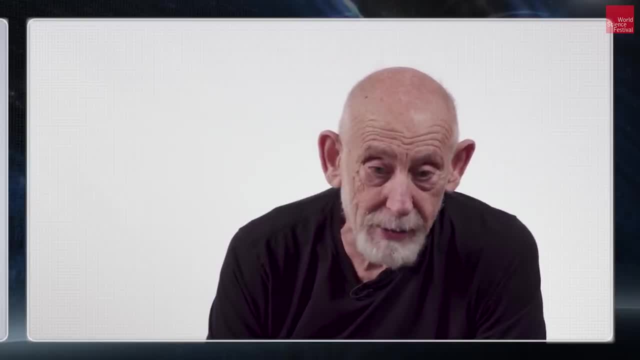 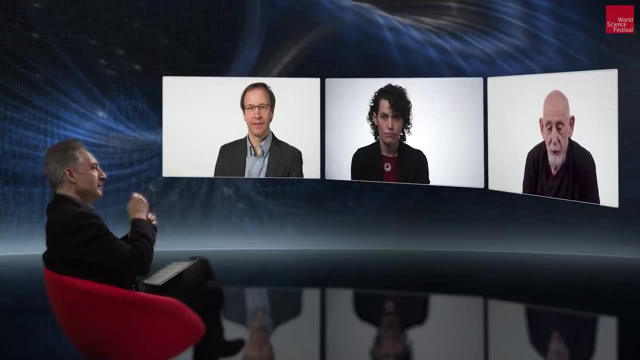 is not broken. It's just that the information right behind the black hole is the same as in the Hawking radiation. And that was my opinion: that somehow, in some mysterious way, the interior of the black hole just behind the horizon was really the same thing as the Hawking radiation. 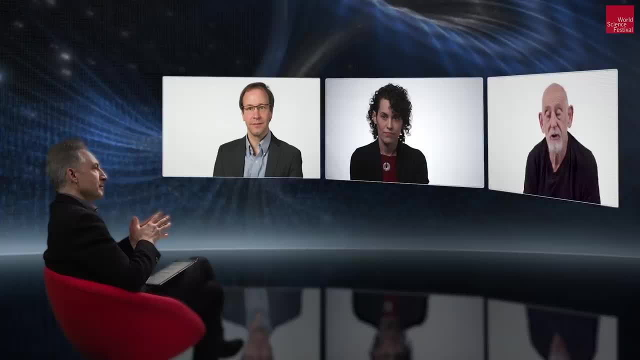 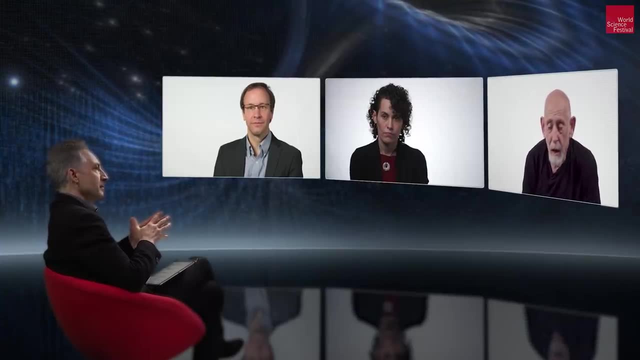 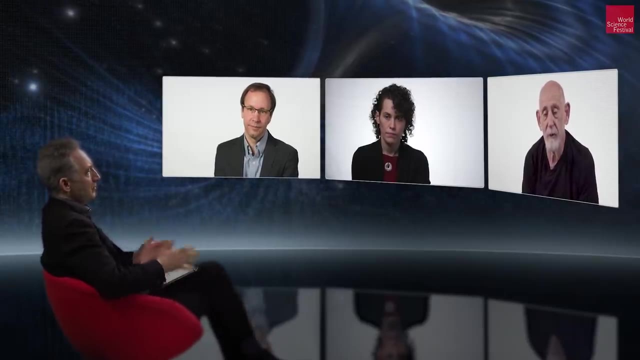 very far away. Another nutty idea that sounds somewhat similar to the holographic idea: information that you thought was nearby, really very far away. Juan Maldacena and I got to talking over the internet. We started collaborating and trying to figure out what was going on with the Amps Paradox. At some point, Juan sent me a very cryptic 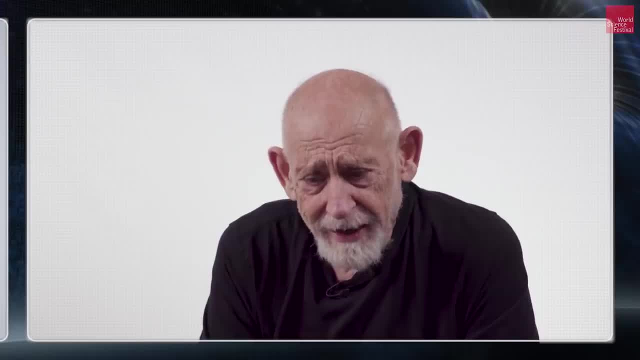 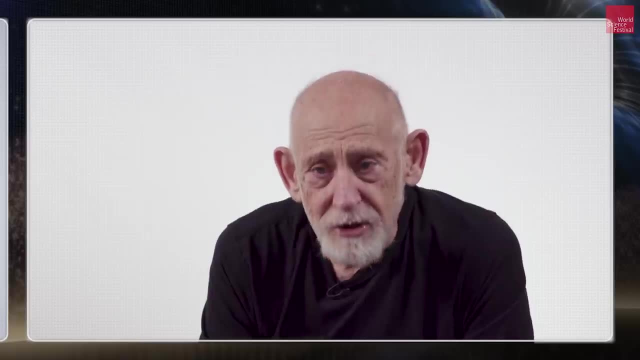 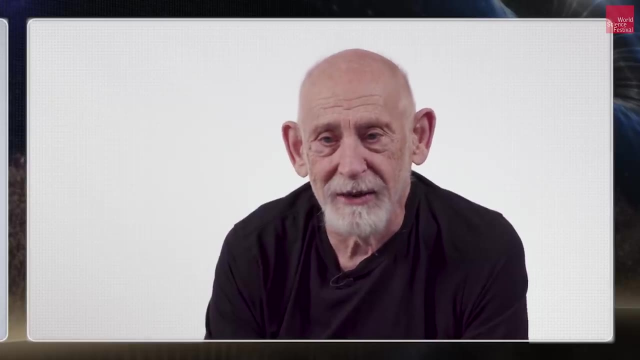 message, And in the cryptic message he simply wrote down: ER equals EPR. I knew instantly what he was talking about. That just was an explosion in my brain when he said it. I knew exactly what he was talking about, but he said it in such a clear way. Now what did it mean? 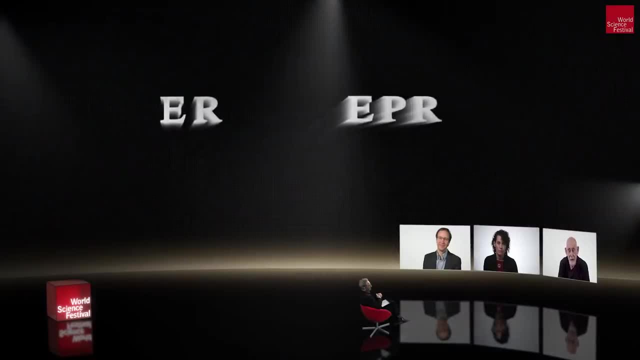 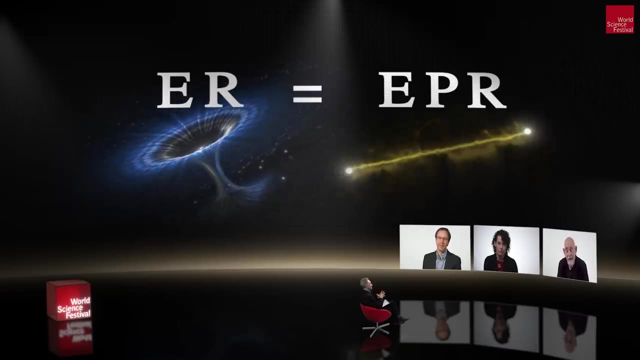 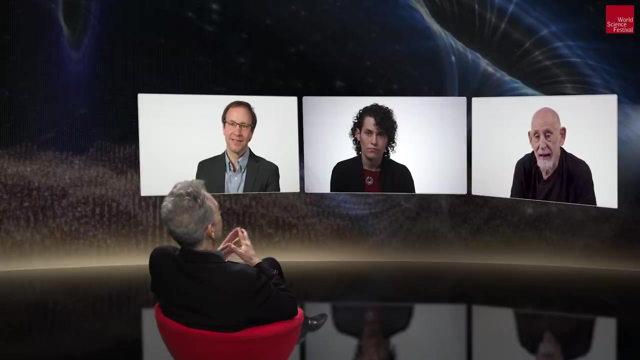 ER stood for Einstein-Rosen, EPR stood for Einstein-Podolsky-Rosen. Remember what that took. I knew exactly where they are: Einstein-Rosen wormholes, EPR entanglement. What he was saying was that if there's entanglement, then there must be wormholes connecting. 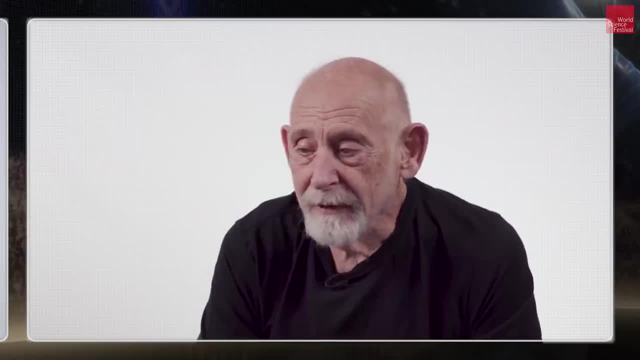 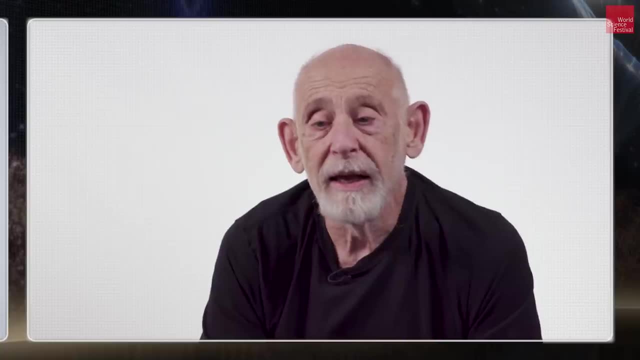 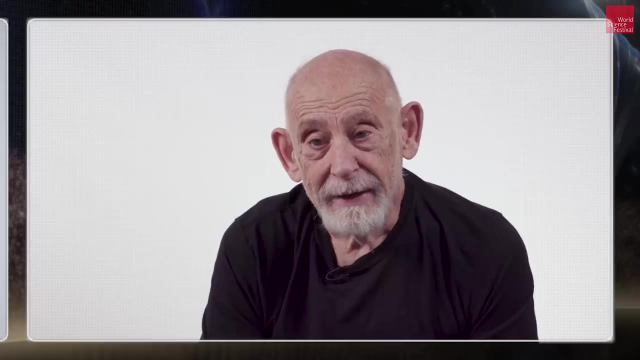 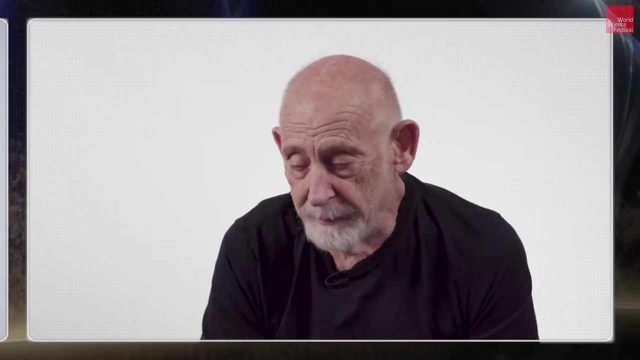 the regions that are entangled. If you took the whole thing together, what it seemed to say was that there must be wormholes or a wormhole connecting the distant radiation to the interior of the black hole. As measured through the wormhole, they're really not very far away, so that what we see as radiation very, very far from the black 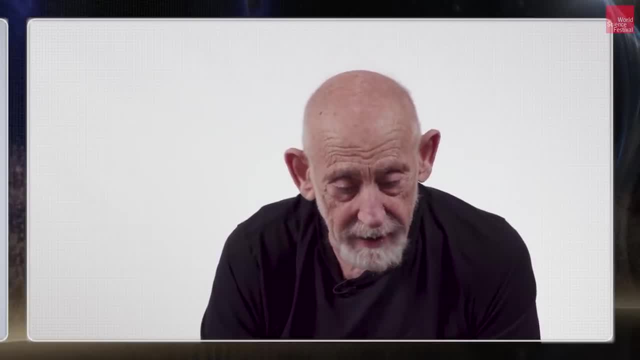 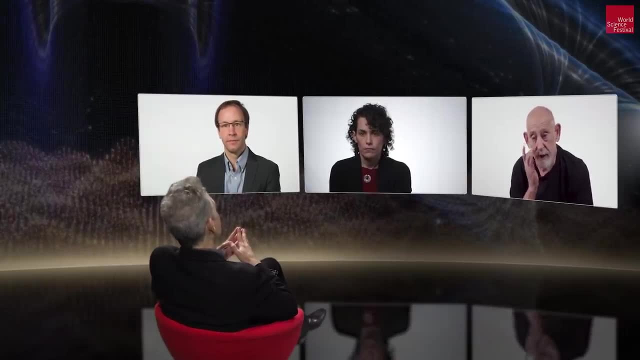 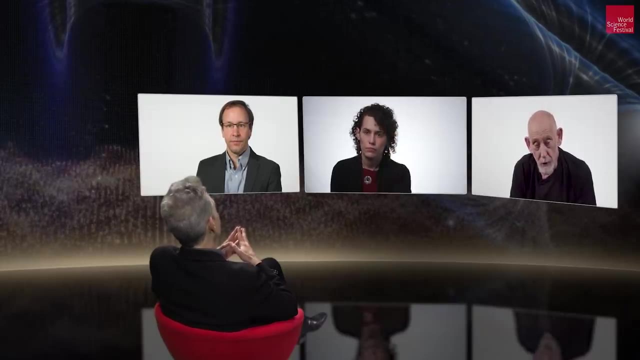 hole is connected through a hidden wormhole to things just behind the horizon of the black hole. That's what Juan meant when he wrote down: ER equals EPR, that that if there's entanglement, there must be wormholes, there must be spatial connectivity. That, in fact. 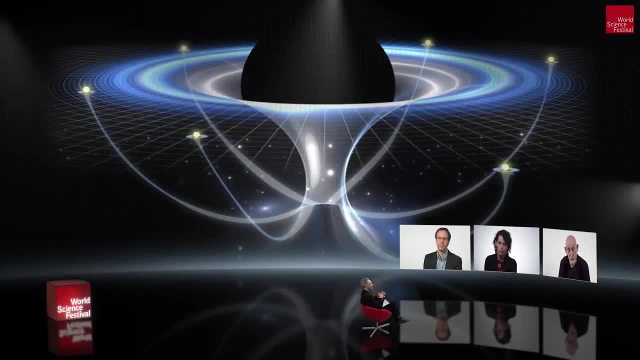 did turn out to be the solution. We believe that is the solution of the Amp's paradox, that the entanglement between the exterior and the interior is not broken. it just reappears as the entanglement between the exterior of the black hole and the Hawking radiation. 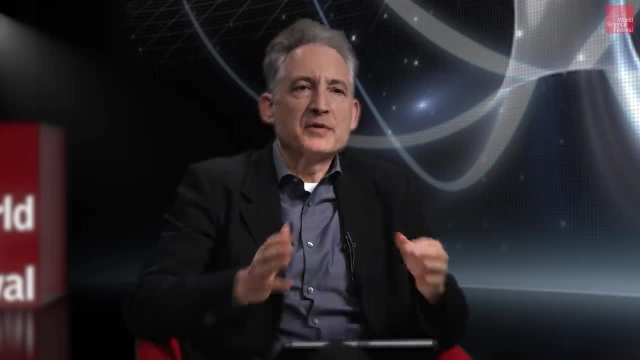 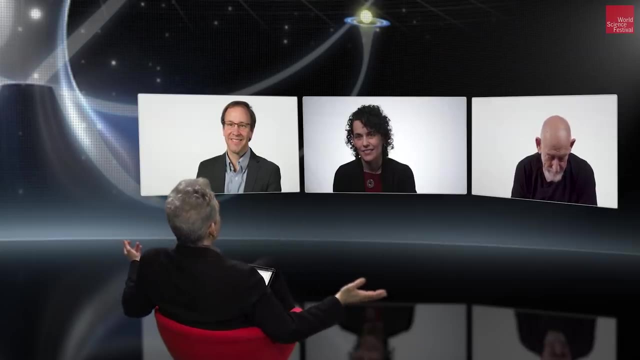 Now, Einstein wrote those two papers like two months apart. That's incredible. Do you think that he had any inkling that there is any connection between them? No, I don't think so. There's no evidence whatever and no, I do not think so. 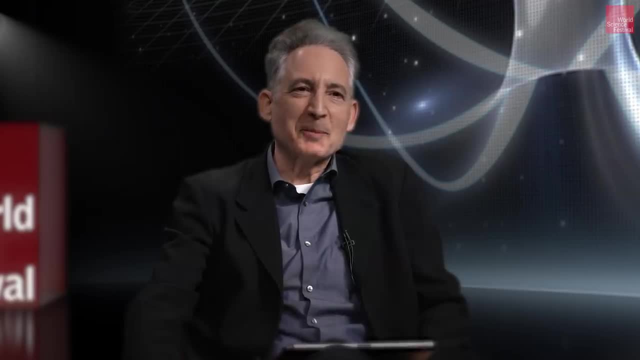 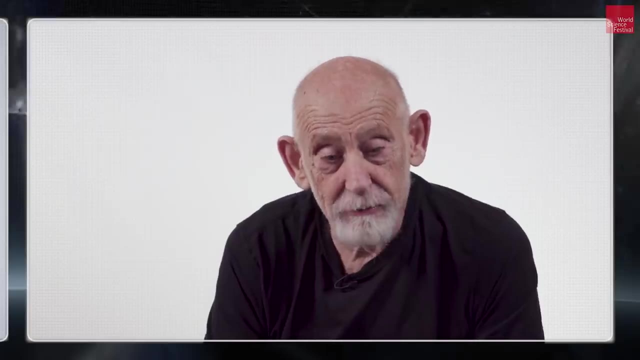 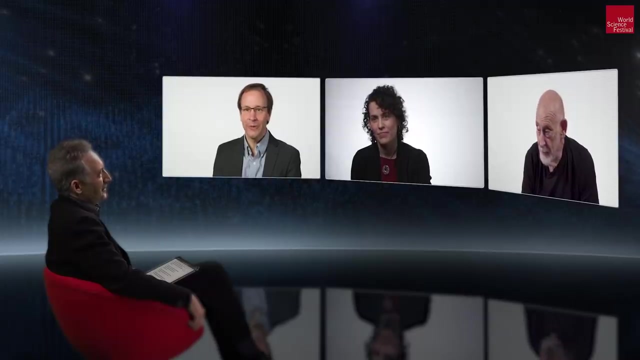 So it's another one of those crazy examples where Einstein is just somehow able to put his finger on things that last and matter. I really think this is just accidental. but who can say Einstein was extraordinarily unusual, but he wasn't supernatural and I don't think 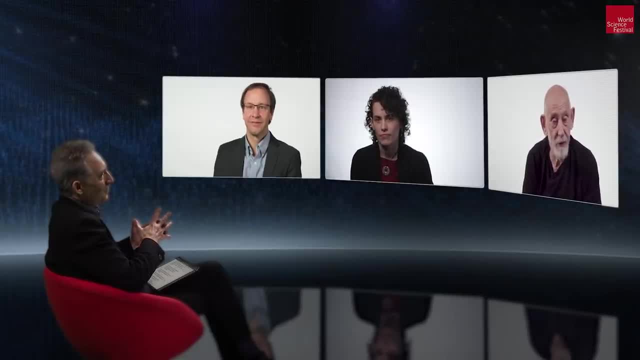 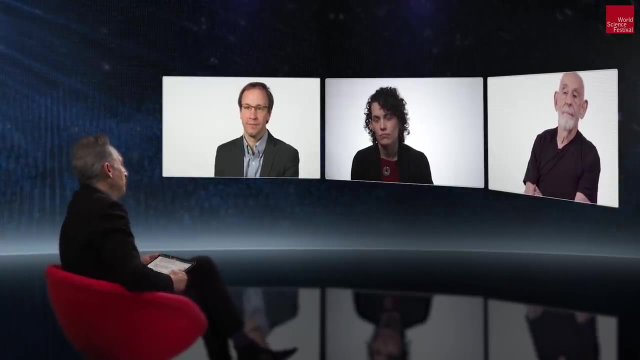 he could have. he didn't have the things which were necessary to formulate a reason for connecting those two ideas. Yeah, yeah, absolutely So. Mark Lenny made reference to your work that played an important role in the remarkable results that he was just recounting. 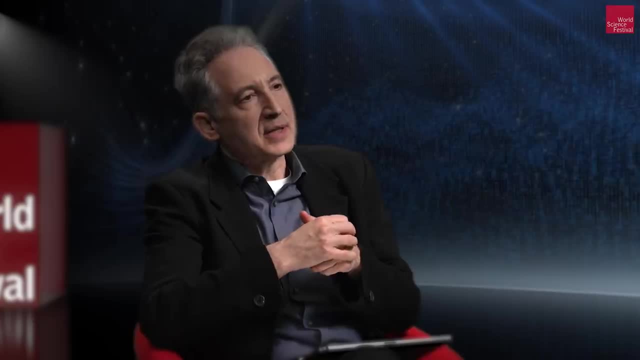 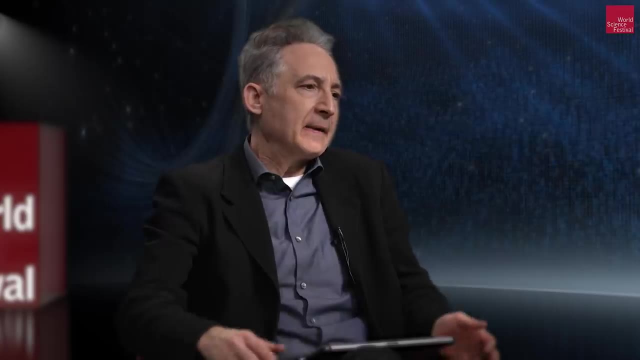 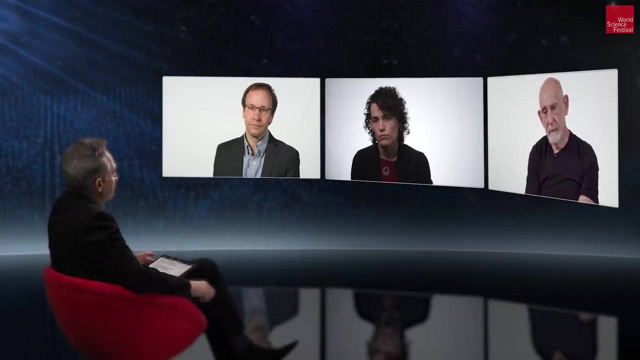 I want to finish up with our final scientific subject, to explore that insight of yours a little bit, and maybe we can do it in two pieces, because part of it makes use of an insight of Juan Maldacena, the physicist that Lenny made reference to, this generalized version, if you will, of holography. 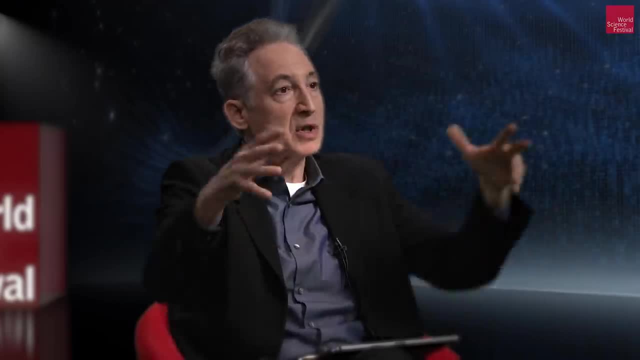 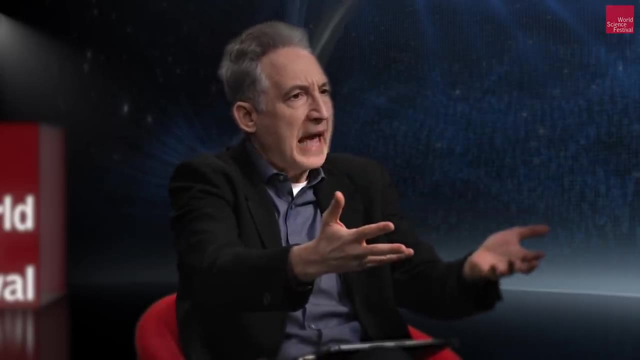 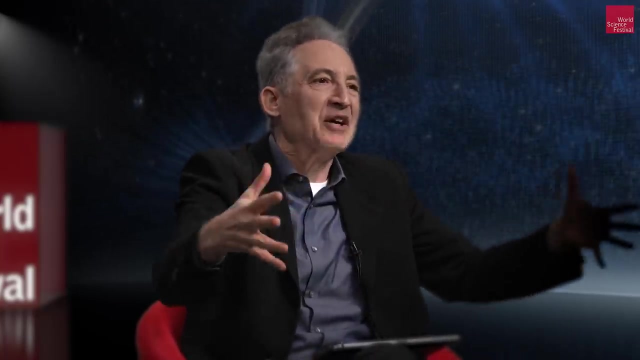 you know describing some region of space by degrees of freedom in physics that lives on a boundary. If you can give us just an intuitive sense of that first, and then we can go on to how that insight is then leveraged into this result about how space is held together by quantum entanglement. 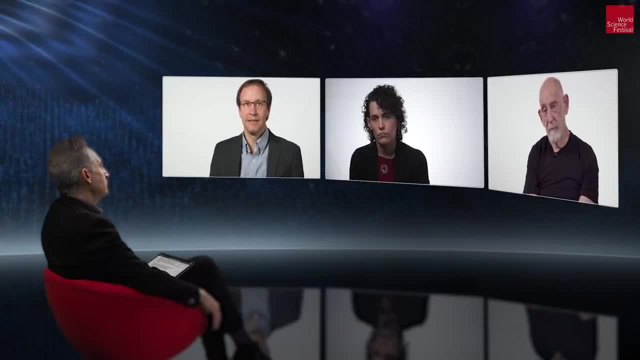 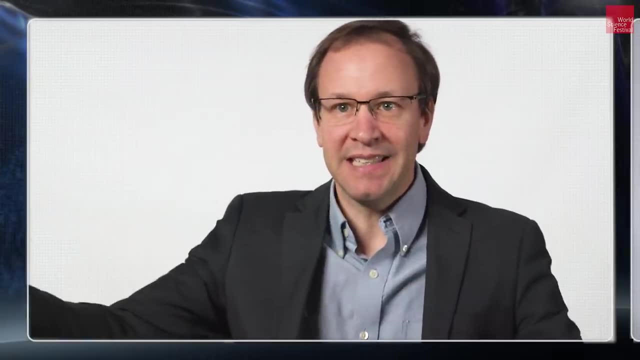 Yeah, So I think that the way I would describe holography is the idea that what you see in a gravitational universe is really not. it's somehow encoded in a way that you know. 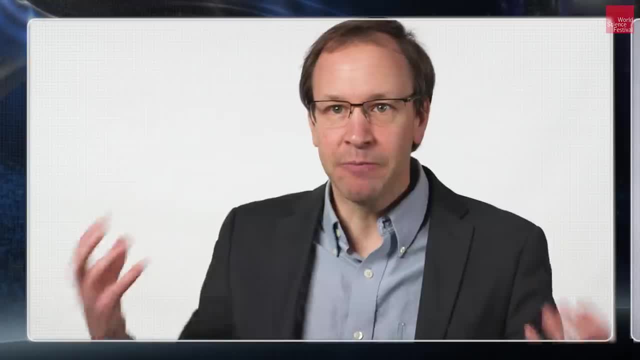 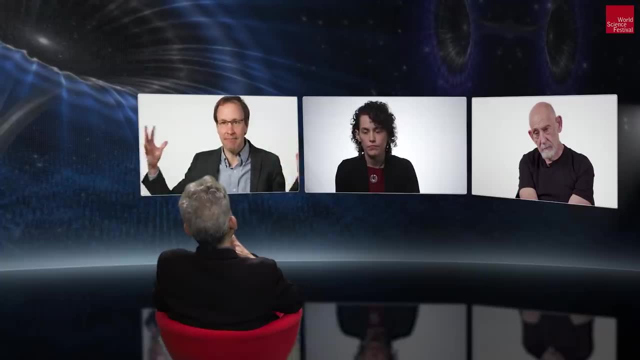 So it does happen to have the same geometry as the boundary of space in some examples. 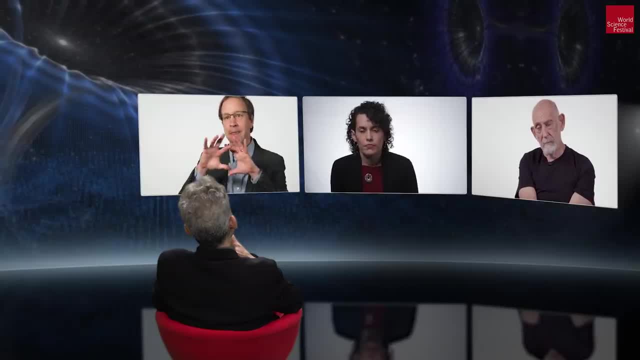 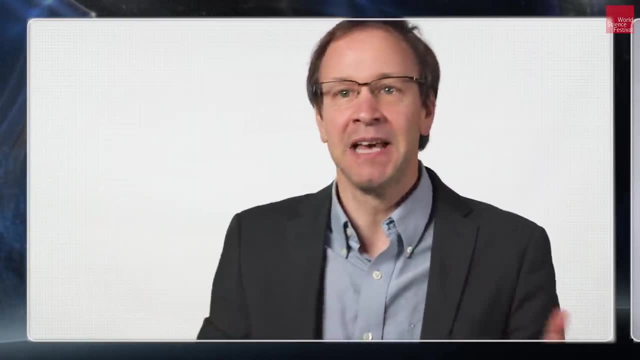 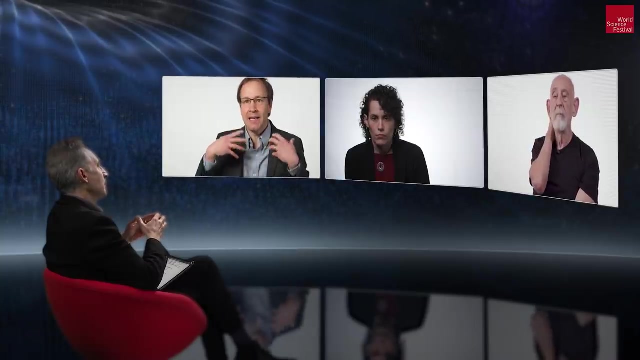 but I think maybe the more general idea is that you got some kind of more or less ordinary quantum system that doesn't have gravity And some of the examples. it's basically, you could imagine, a spherical shell of some exotic material, material- and that thing is able to encode the physics of a gravitational 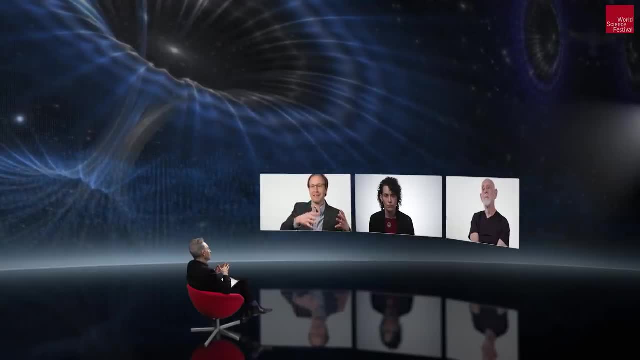 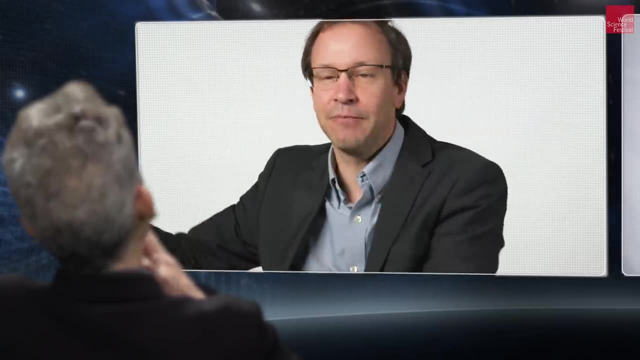 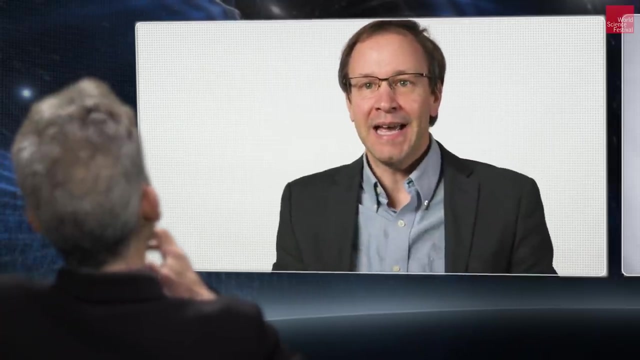 universe. and then there's a basic question: well, how does it do that? how does how do you store the information about geometry of space and the presence of black holes and radiation? all this, how does that stored in this much simpler kind of quantum system? and we've eventually come to an understanding that 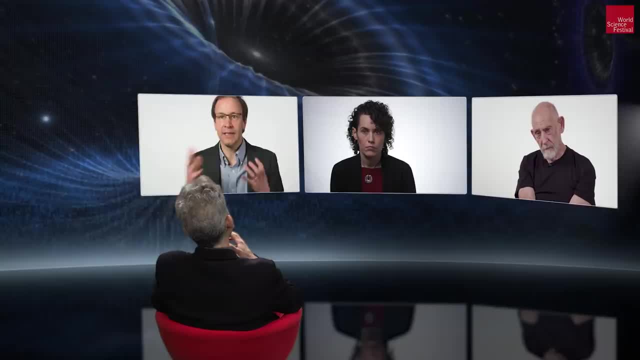 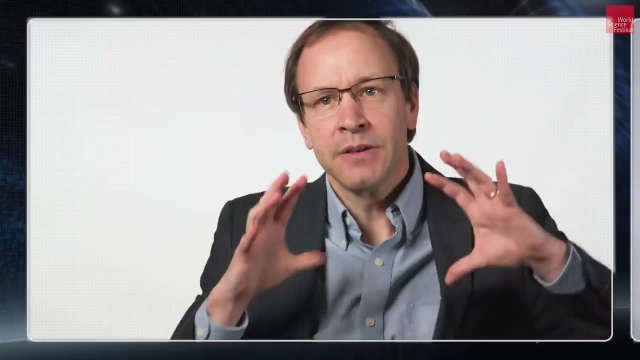 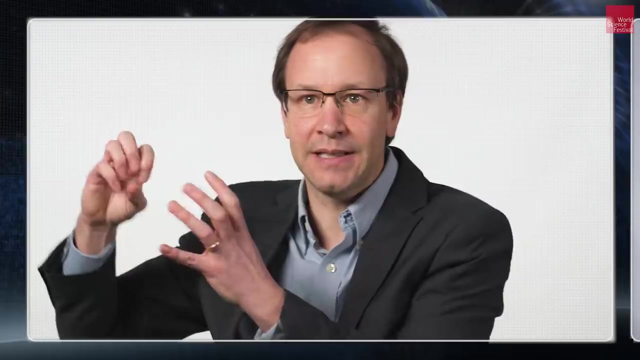 actually thinking about this story of entanglement is really important for understanding. how does that information about gravity encoded in this, in this more ordinary system? so Maldacena gave a really interesting example where he wanted to describe not just a single ordinary black hole but a kind of more. 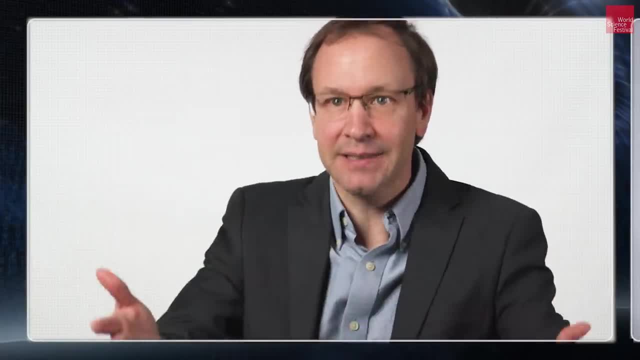 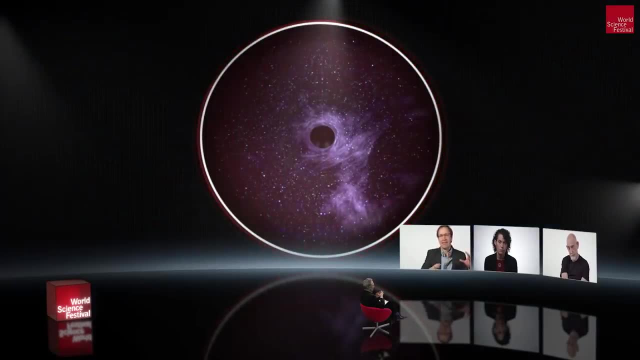 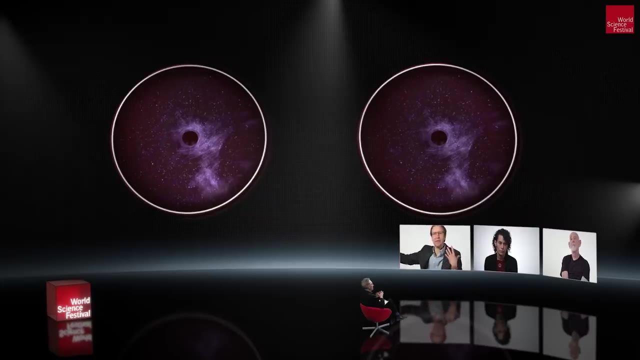 exotic system. that is basically the one that Einstein and Rosen thought about. so you one way to describe that is you have a black hole in one universe, or one part of a universe, and another black hole- and Maldacena was thinking about the case where that was in an entirely disconnected, separate universe, and so 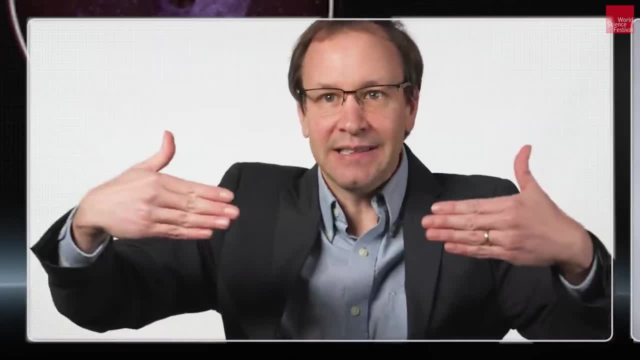 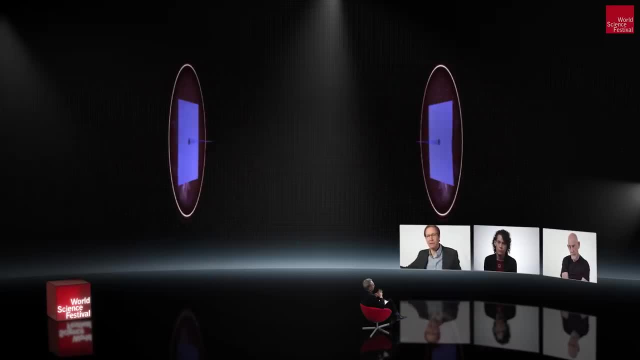 there's this configuration where geometrically those two things are connected such that if one person went into the horizon of one black hole and another person from the other universe went into the horizon of another black hole, they could- they could meet in the middle. so there's a spatial 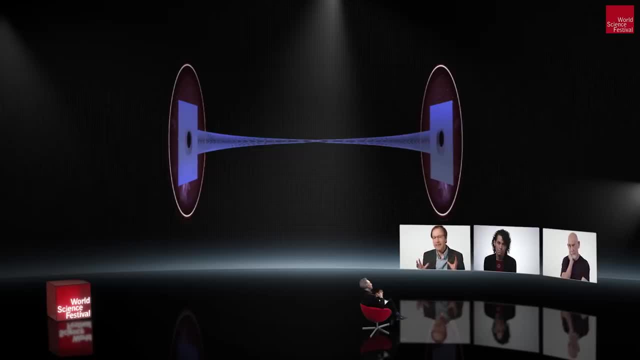 connection between these things. and so Maldacena said: how do we describe this thing using this holographic approach? and he says: because there's two universes that you know otherwise, apart from this wormhole, they're just separate universes. well, this should involve two copies, two sets of two copies of this. 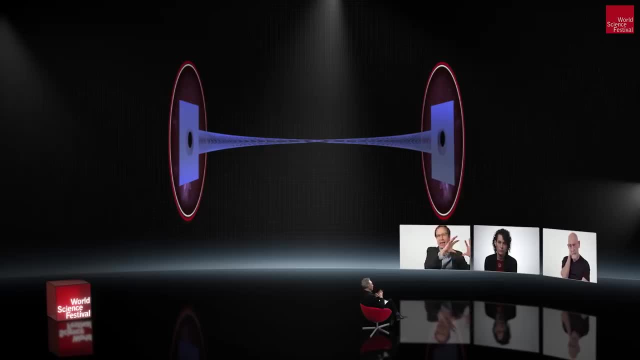 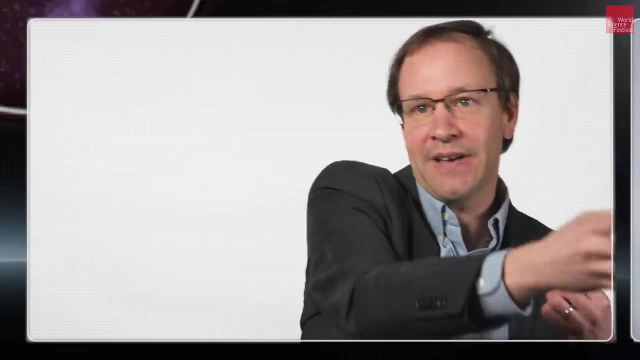 quantum system that we were talking about before. so you can imagine having two of these spherical shells. and he says that if you want to build one of the wormholes, well, you put a lot of energy in one. to get a black hole, you put a lot of energy in. 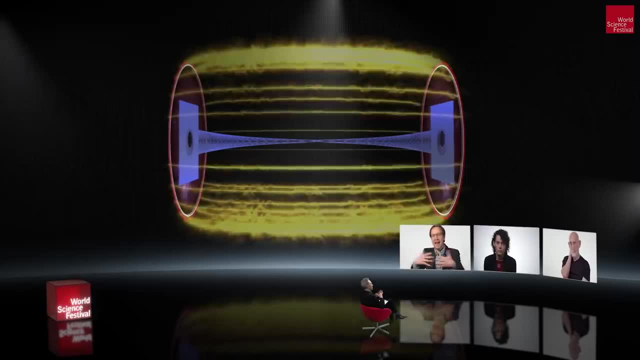 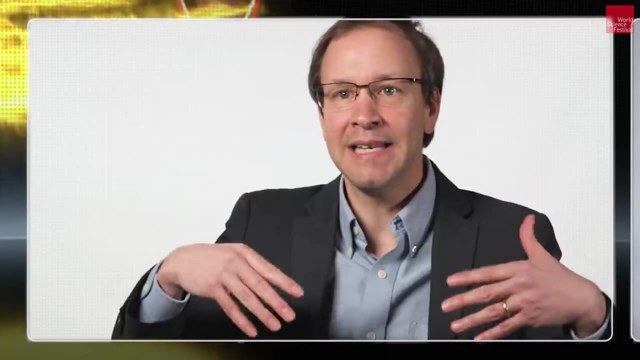 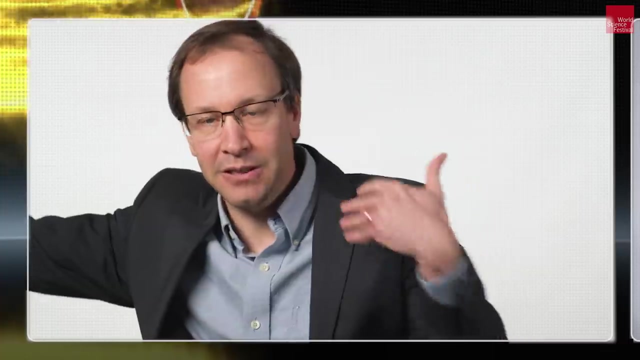 the other to get a black hole in the other space-time. but then you entangle them in this very special way and that's the only thing that connects them. and he says: well, this is the natural description in quantum mechanics of that space-time where you have the two parts of the two universes connected by a. 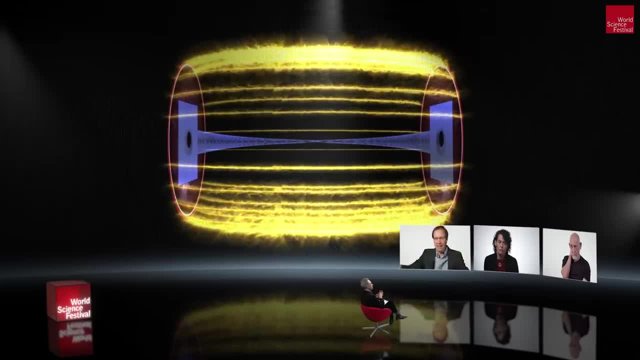 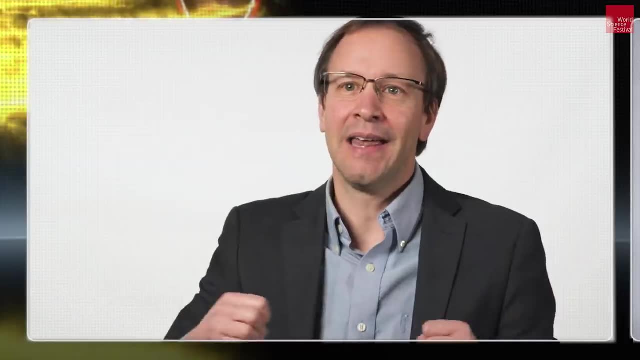 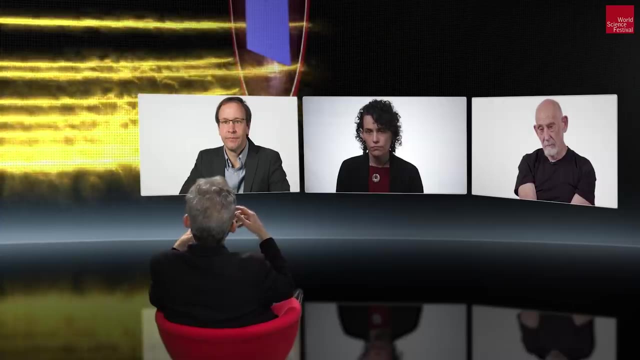 wormhole and it just struck me that, really, because this entanglement is the only thing that makes these two systems have anything to do with one another, then maybe that's the thing that is just directly responsible for creating this wormhole. as I said, you did a study, theoretical study, of course, where you 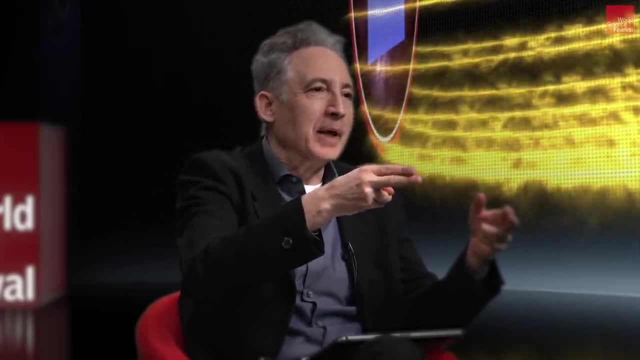 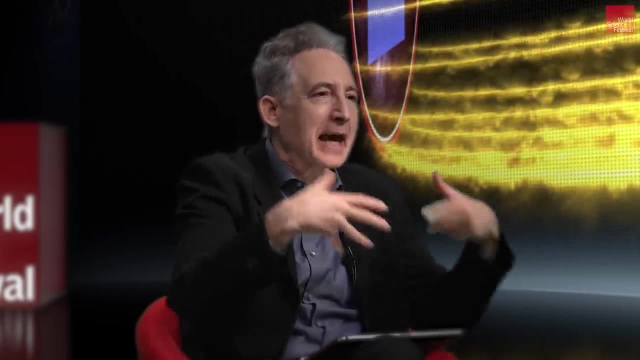 were kind of snipping the threads of quantum entanglement and recognizing its impact on the connectivity of the quantum entanglement and recognizing its impact on the connectivity of the of space, and that to me really brings it home. so you can describe how that goes. 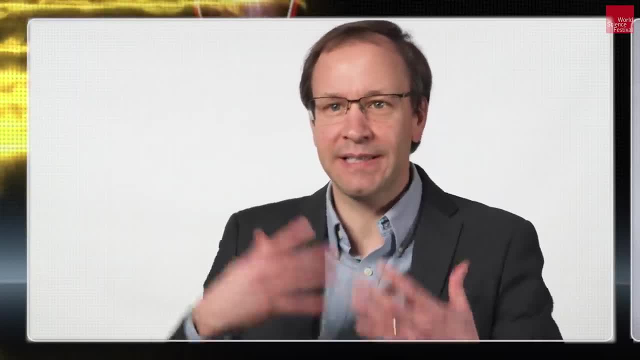 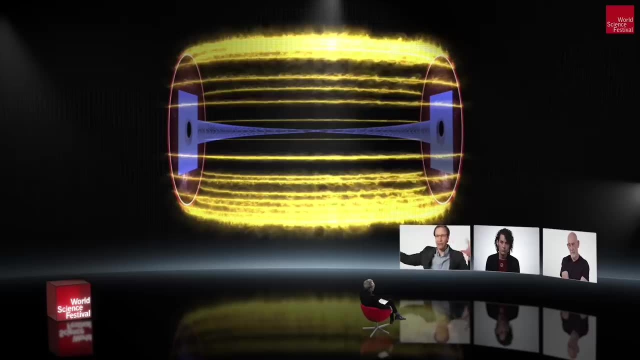 yeah, yeah. so I was wondering, you know, is this something that is specific to this black hole? space-time? that's kind of an exotic thing having two universes connected by a wormhole. so is that, is it that entanglement makes these exotic wormholes, or is it just the more basic thing, that entanglement is the thing? 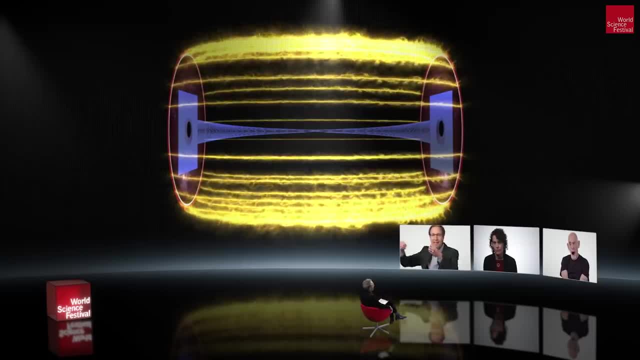 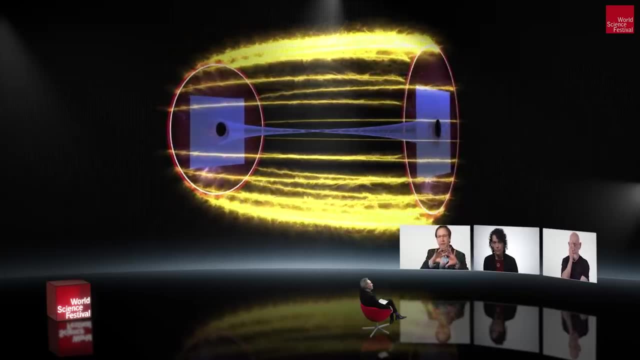 that is responsible for any space-time entanglement, yeah, yeah. so I was wondering, you know, is this something that is specific to this being connected with any other space? and so what I thought to do was just look at a simpler example where you go to the case where you just have one of these. 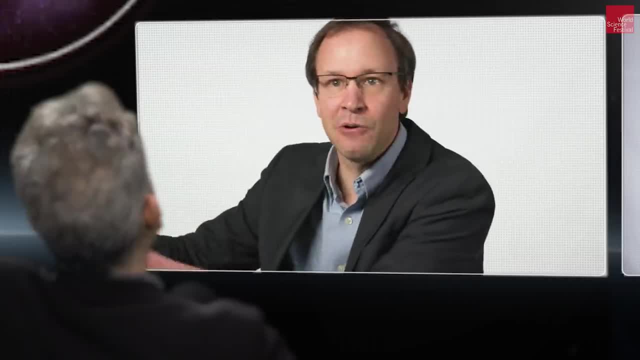 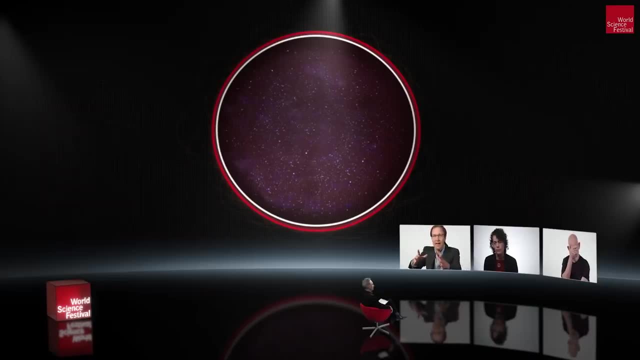 quantum mechanical systems describing a completely boring empty space-time. so, just like we were talking about with the near the black hole horizon, you have an ordinary kind of empty patch of space. there's lots of entanglement between the fields here and the fields here, so that's the same in these holographic. 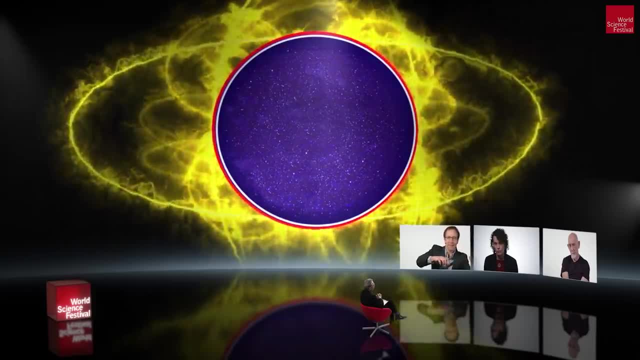 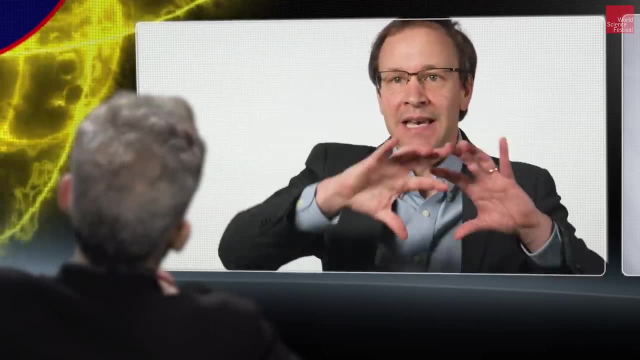 quantum mechanical systems, and so I was wondering if you could talk a little bit about what happens when you have two different systems. they have lots of entanglement between the left side of this ball and the right side of the ball, and so I wondered: well, what would happen if you envisioned altering the state? 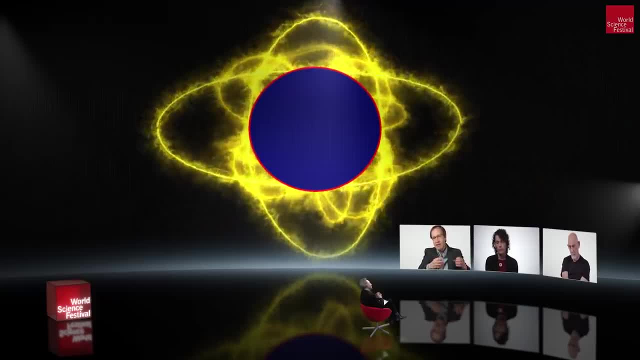 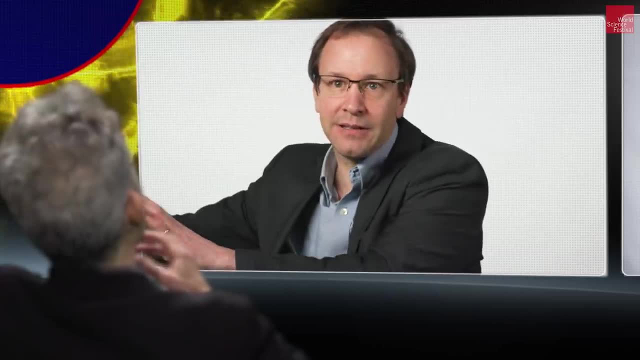 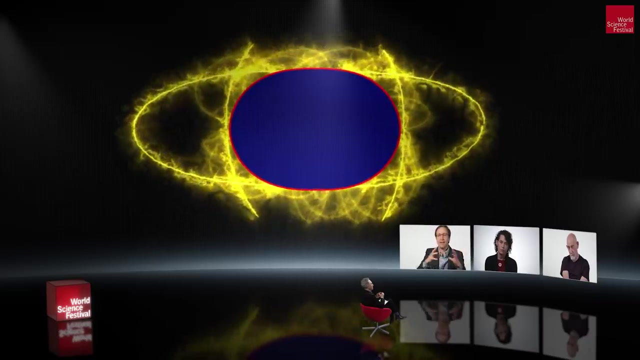 altering this state. you have to add energy, but to you add energy in such a way that it removes entanglement between two sides. you could kind of follow it through and ask what happens to the space-time, and it seemed that as you removed entanglement between one side and the other, then what happens? 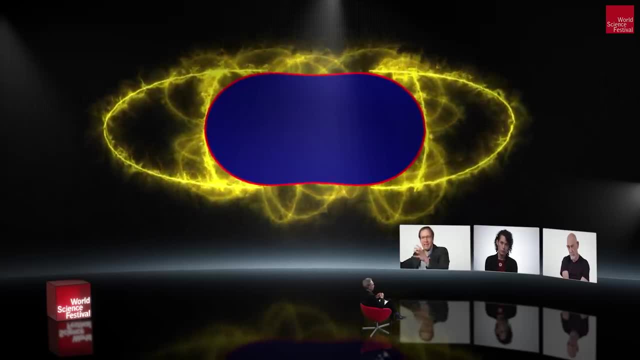 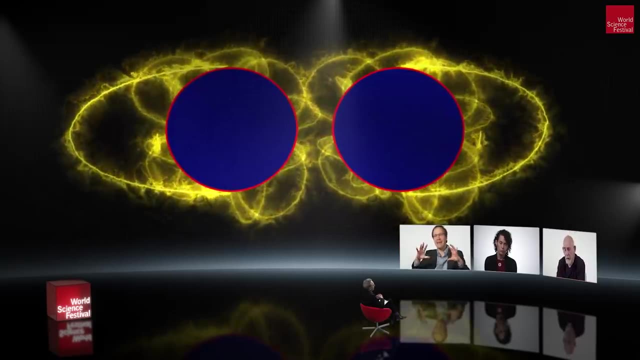 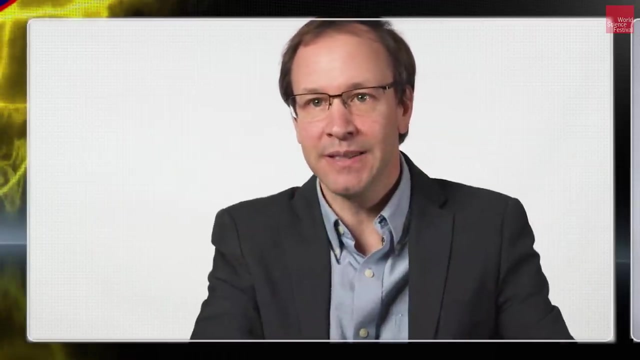 to the space-time is. it kind of pulls itself apart like like pulling a piece of gum apart. it gets, you know, thinner the connection and eventually would snap and be basically just two disconnected pieces once you've removed the entanglement from the underlying quantum system, and then you can just keep doing. 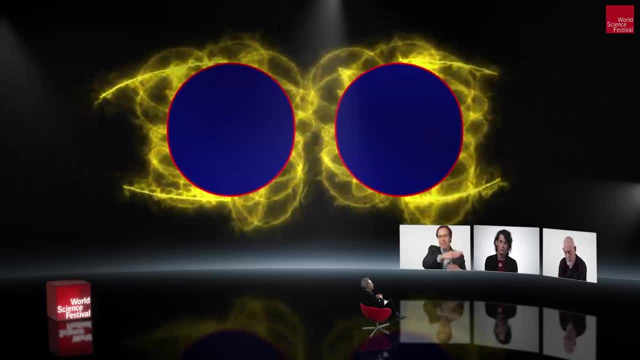 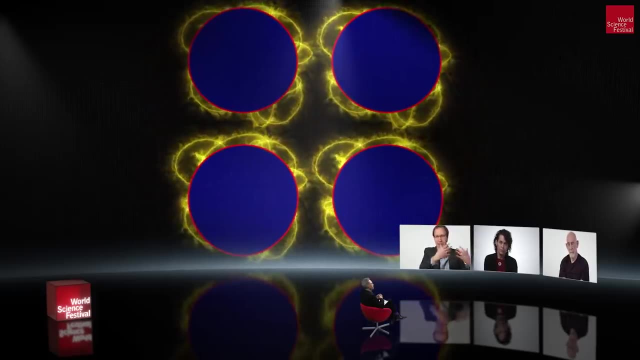 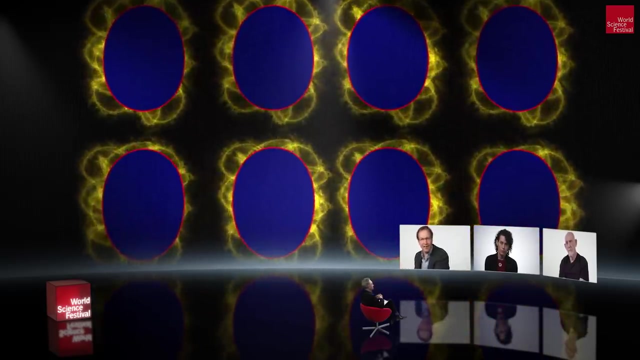 that you know you'd have two pieces now. you could divide up this ball into more pieces, remove the entanglement between those further pieces, and if you just kept going and going, it seems that on the gravity side you really have nothing left at all. and so when you say there's no, when you say there's nothing there at, 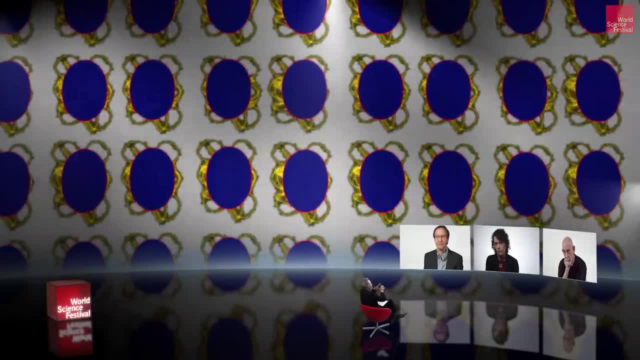 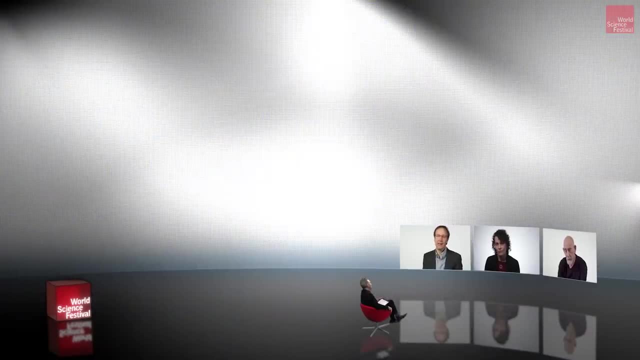 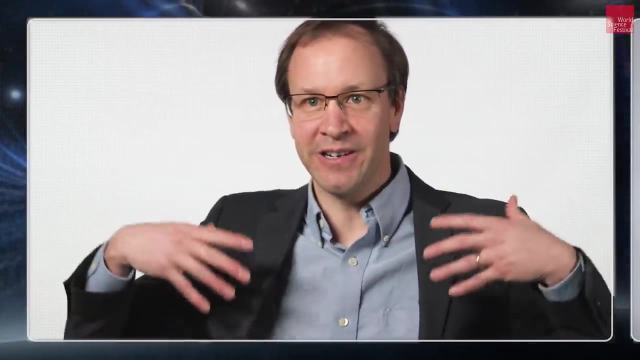 all. I gather you mean that in some sense spacers keeps cutting up into smaller and smaller kind of pixelates, to the point where no connectivity is left and it's just gone. yeah, that's, that's right. so you just have you know. we think of maybe space as being the background for everything else, but with 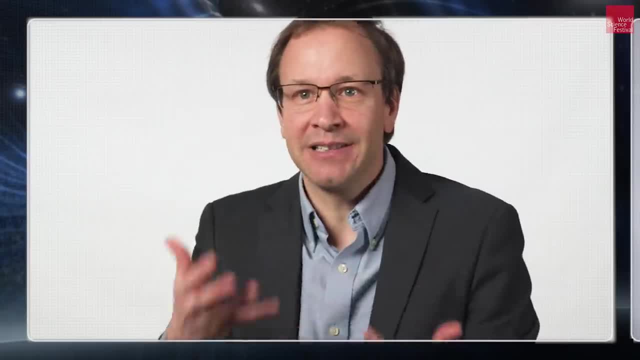 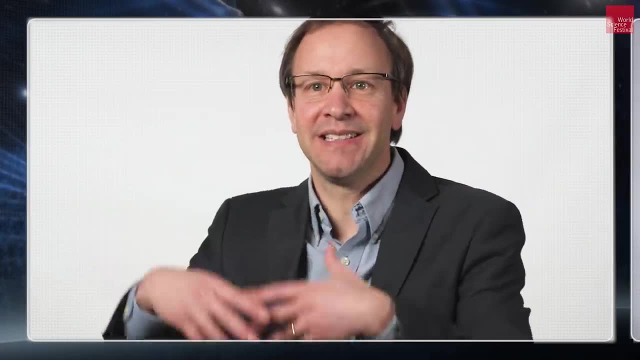 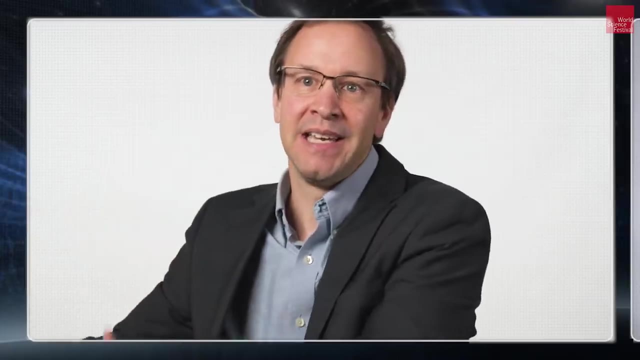 Einstein, space became a dynamical entity and then you could start to ask the question: maybe where does it come from? is is it always there? and this picture said. this holographic picture suggests that even space, in order to exist, you need quantum entanglement between these underlying physical 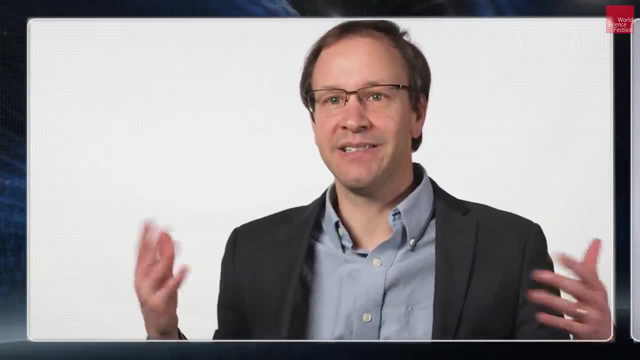 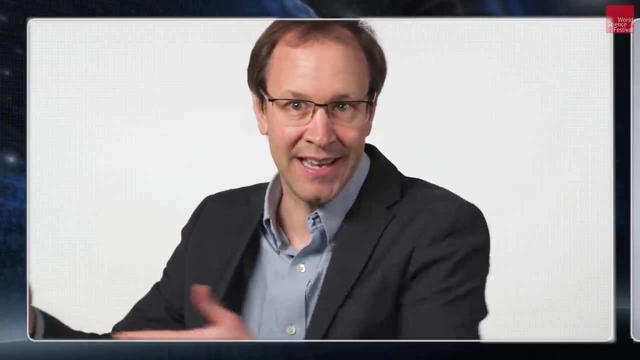 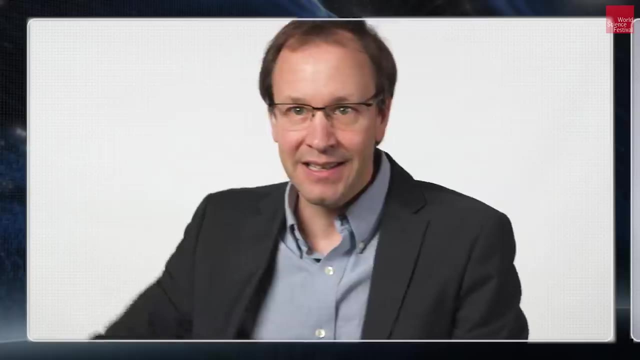 entities. so it's- it's kind of bizarre like we went into studying string theory and holography to really to understand quantum gravity and then, when you get to this kind of observation, it suggests that even if you're trying to understand classical gravity, then there's quantum mechanics behind that. 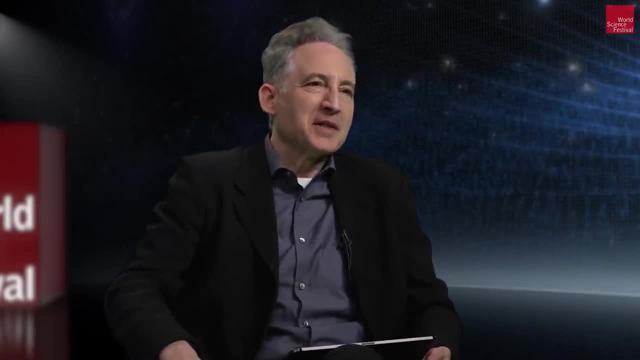 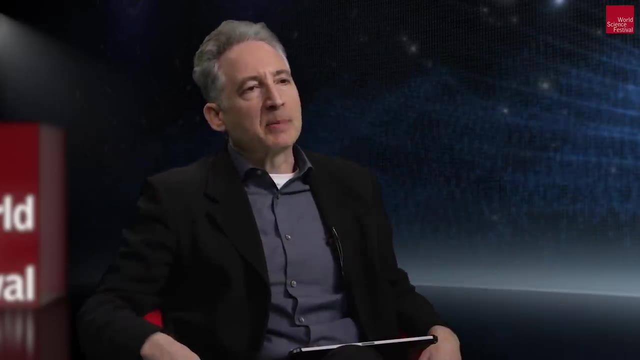 yeah, that takes us to our, to the final question I wanted to ask. that's a perfect segue in so, so on a final question that I'd like everyone to weigh in on. in traditional approaches to quantum mechanics, the way we often teach you to our students is: we have a 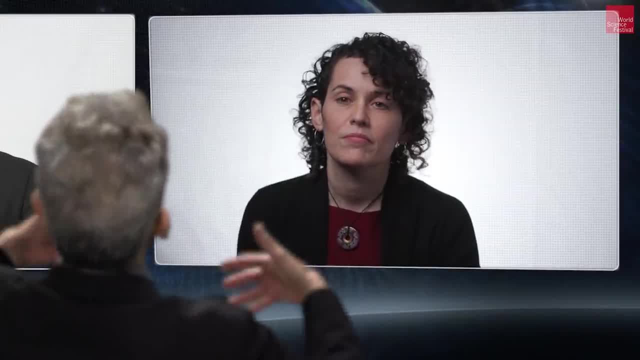 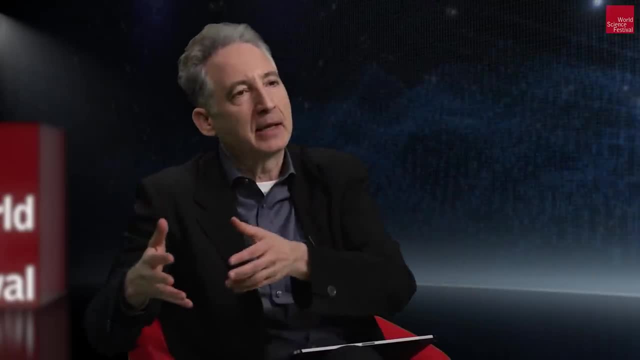 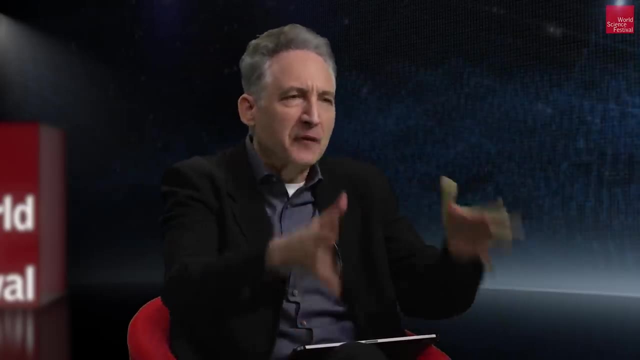 and then we quantize it. We employ certain rules of quantum mechanics to take whatever system that we might be studying using Newton's equations and translate it into a system using Schrodinger's equation, the quantum degrees of freedom. Now, when we've tried to do that straightforwardly, 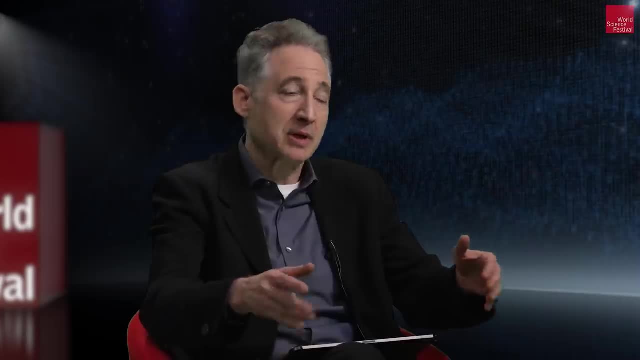 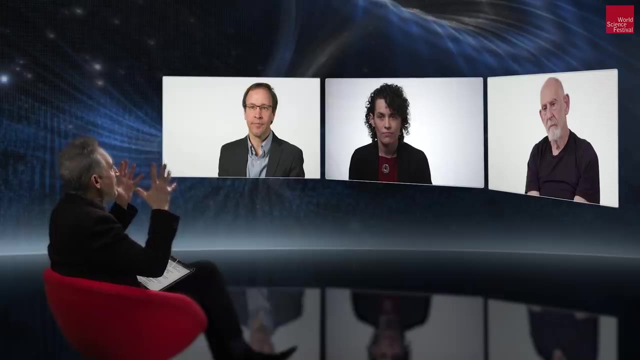 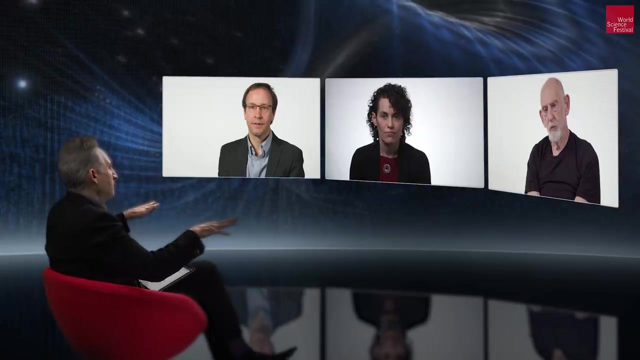 with gravity, we've always run into headaches, which is what has motivated approaches that many people follow, from loop quantum gravity to string theory and so forth. Now we're learning that in some sense, quantum mechanics knows about space. Space, according to Einstein, is the arena It's. 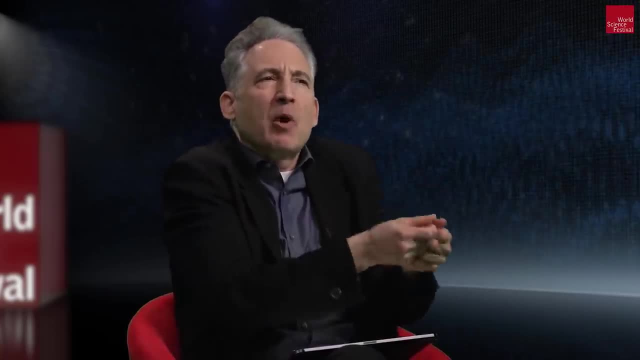 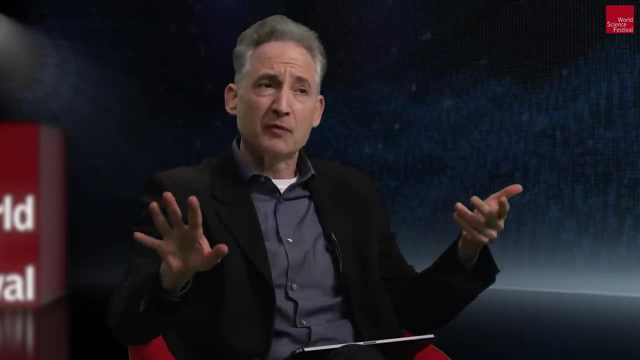 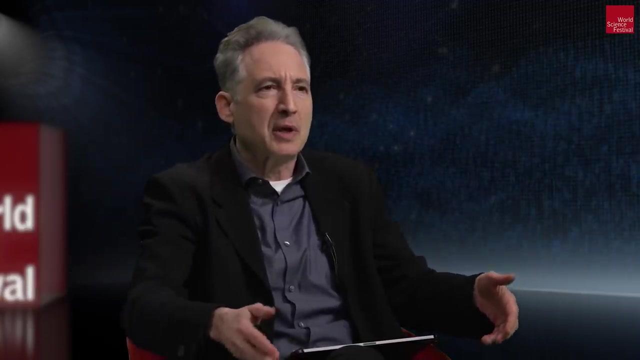 warps and curves of space that give rise to gravity. So in some sense quantum mechanics seems to know about gravity. So is that quality of quantum mechanics that was overlooked for a long time. do you think that might have been the reason Why we had such trouble using the standard quantization rules and trying to apply them to? 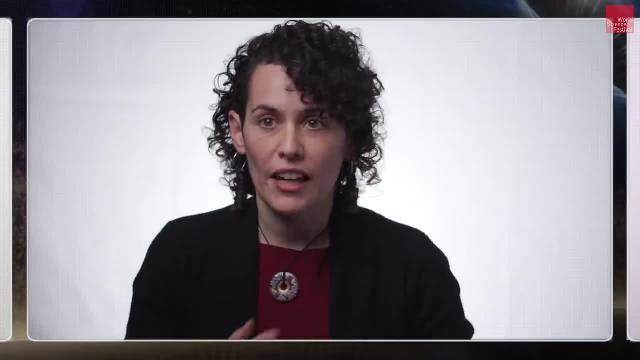 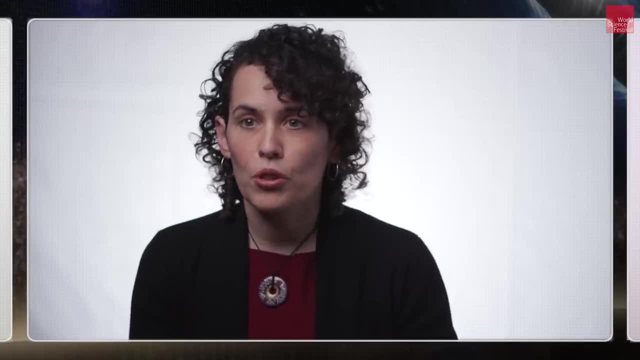 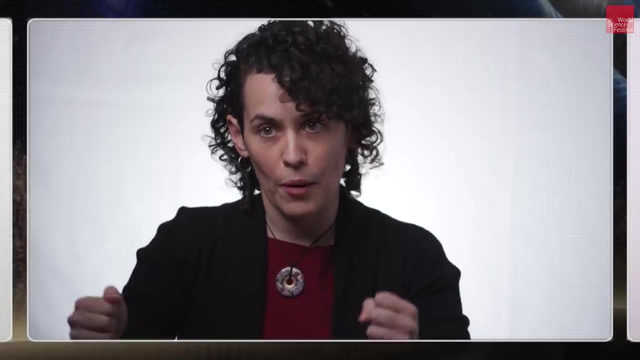 gravity itself. What happened, at least to me in the last years, and inspiring all the proposals that they have mentioned, is that I'm not sure if it's coming from quantum mechanics as a basic setup that has a control over what happens there, But what is nowadays clear is that quantum 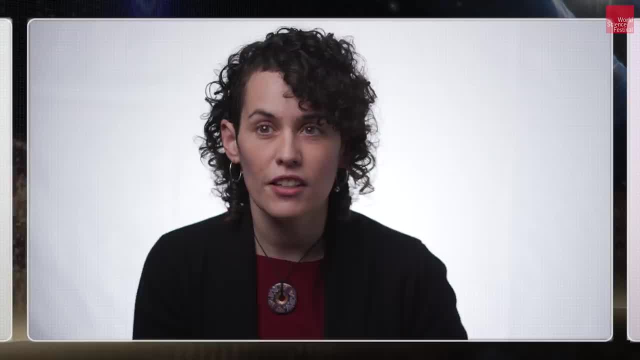 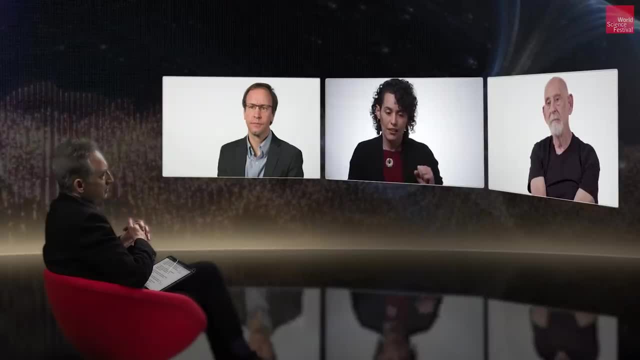 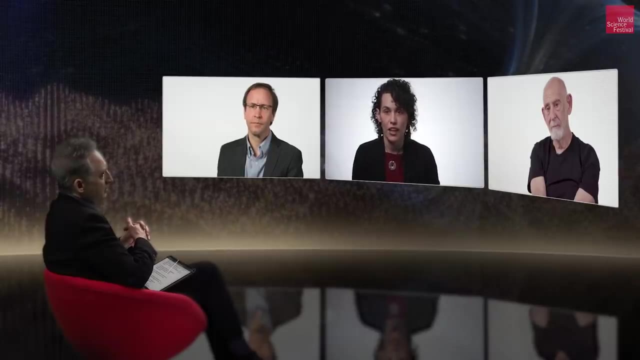 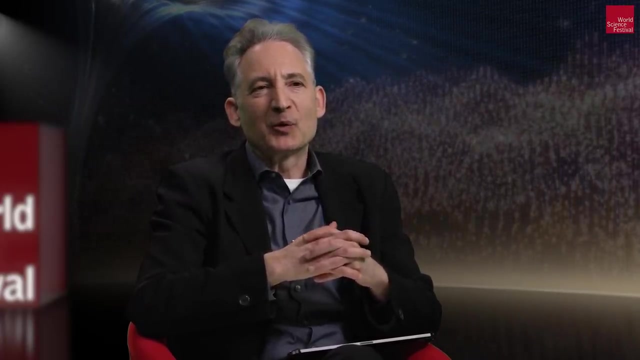 mechanics is giving us a the necessary tools to understand this connection between gravity and quantum realm in the sense of this, precisely this entanglement. So Lenny, big picture. people have been trying to put gravity and quantum mechanics together for a 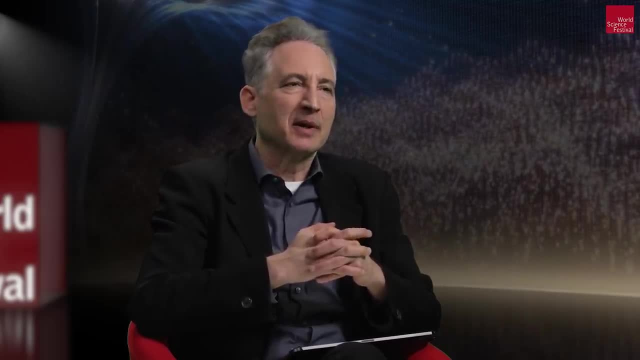 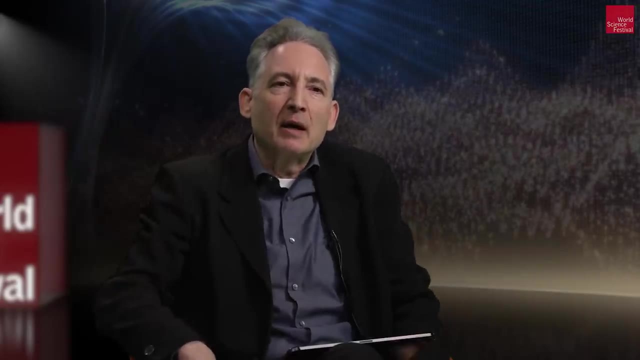 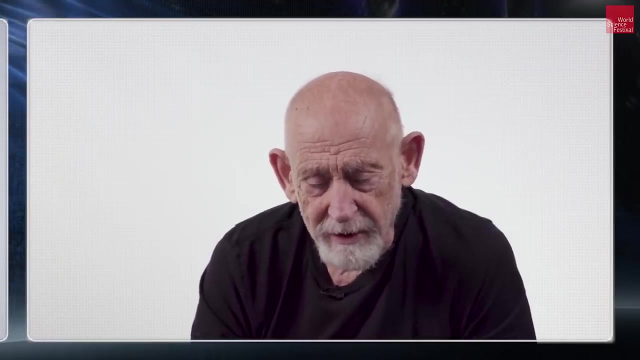 long time, You've, of course, spearheaded the most insightful approach to that which is string theory. But if theyszy Capion asks about quantum mechanics, please, Lenny, Do these recent developments? do they change your thinking on the relationship between? 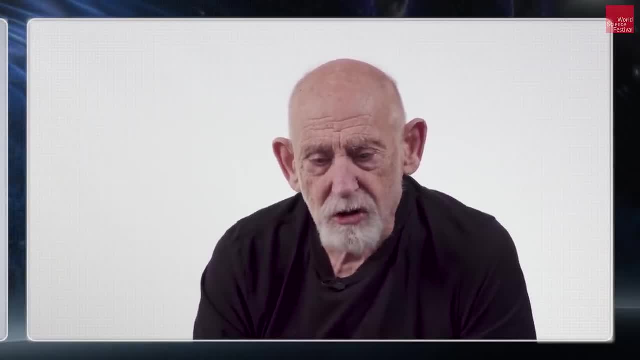 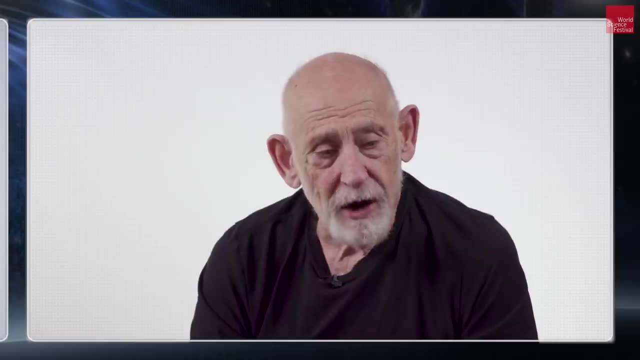 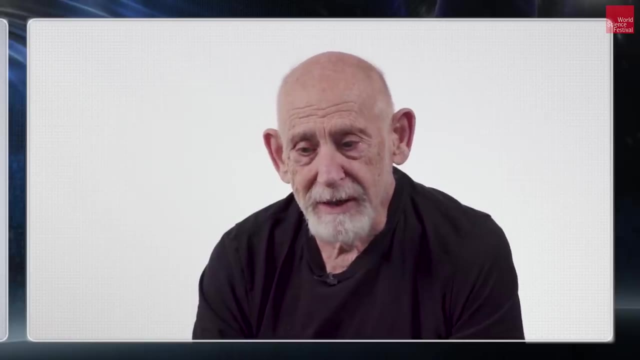 quantum mechanics and gravity. I think what's going on- and I very strongly believe what's going on- is that quantum mechanics and gravity are simply so deeply connected, so intimately connected, so inseparable, that trying to separate them into the classical theory of gravity and quantum mechanics will 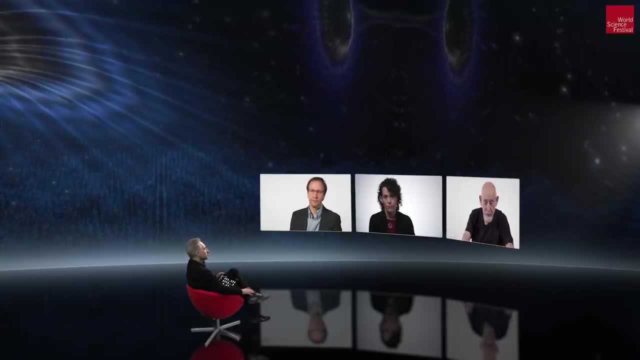 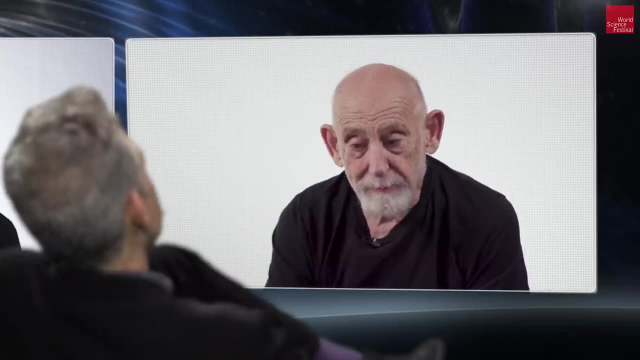 together again. Separate them into these two things and then put them back together by the procedure of quantization will just be the wrong thing, Except that quantum mechanics and gravity are almost the same thing, or that they're at least so closely linked that you can't pull them. 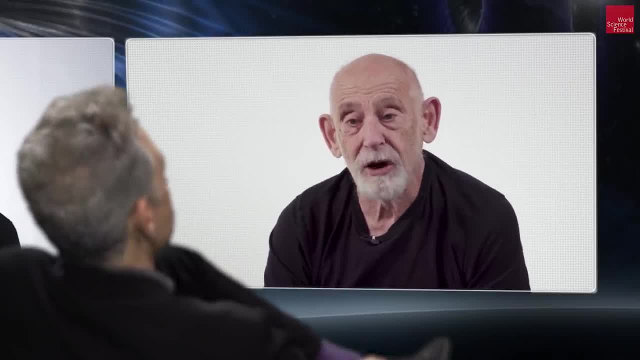 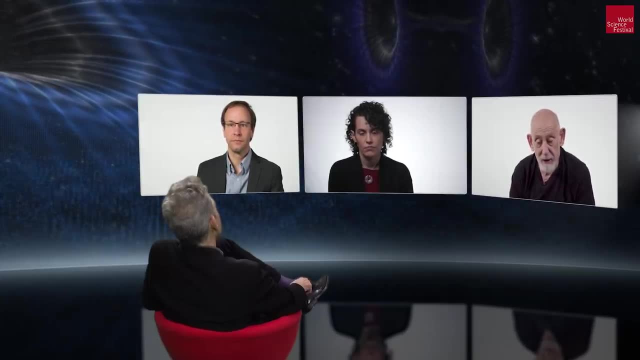 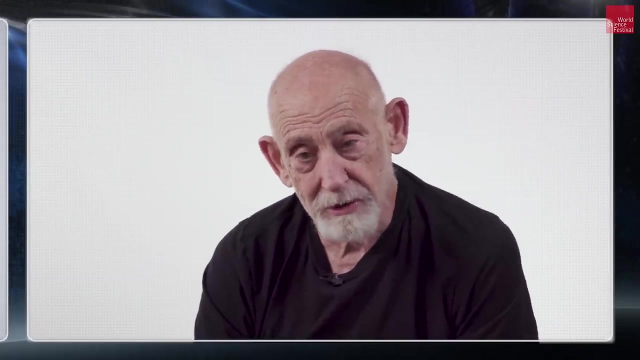 apart and you will never be led to the idea of trying to quantize gravity. So, yes, my opinion is that that's the direction things are going in, And it's why I said in the beginning that perhaps the ultimate mysteries of quantum mechanics will only be revealed when we much better understand. 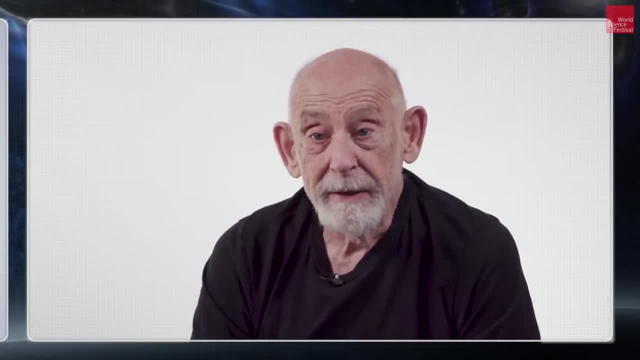 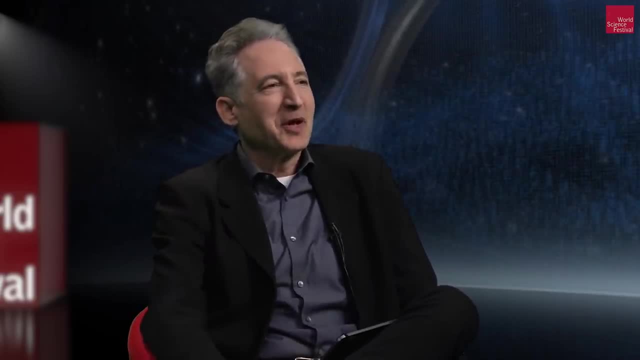 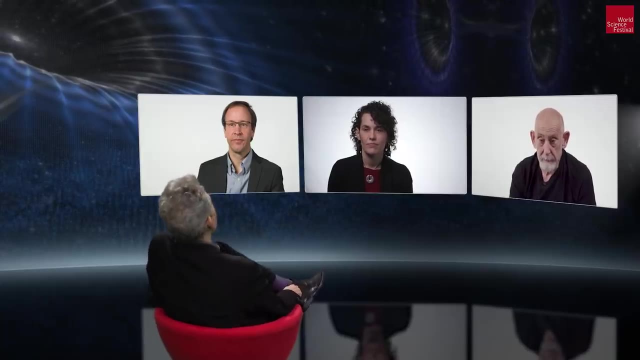 the connection with gravity. But we'll see. Yeah, absolutely So. it's been a fascinating conversation, covered a lot of ground, motivated by Einstein's 1935 papers, And it's an exciting time in physics and who knows where it's all going to lead. But it's so remarkable to me that we're 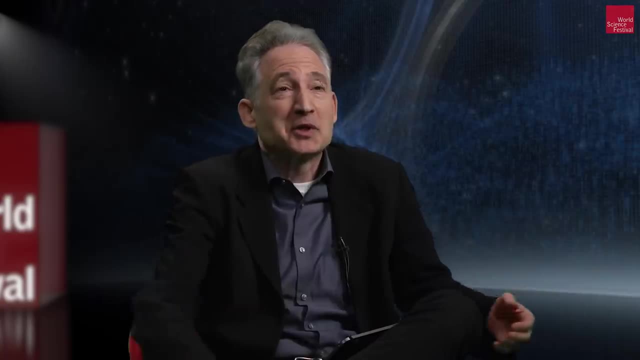 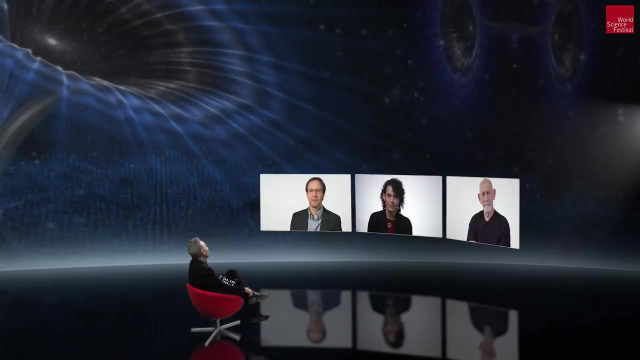 actually talking about things like what is space made of? the kind of question that, like as a high school kid, many of us worried about and thought about, but never thought there'd be any insight. So congratulations, all the work that you have all spearheaded to push the frontiers forward. 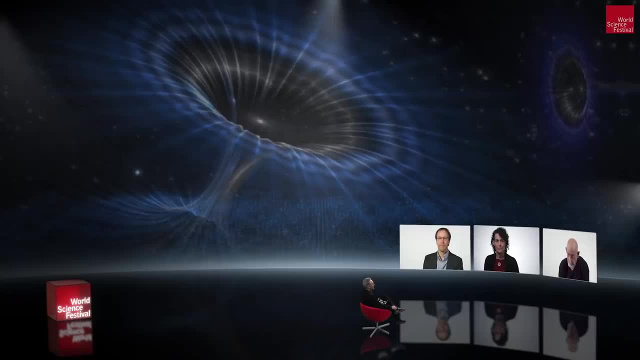 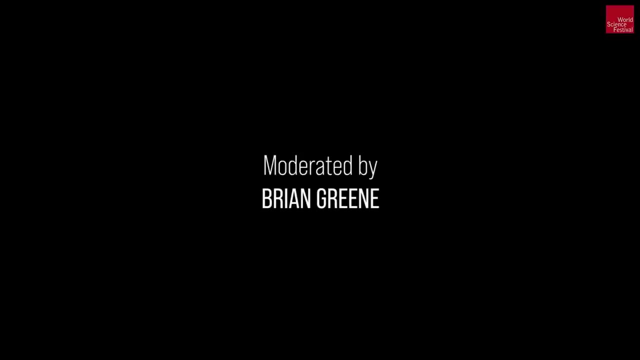 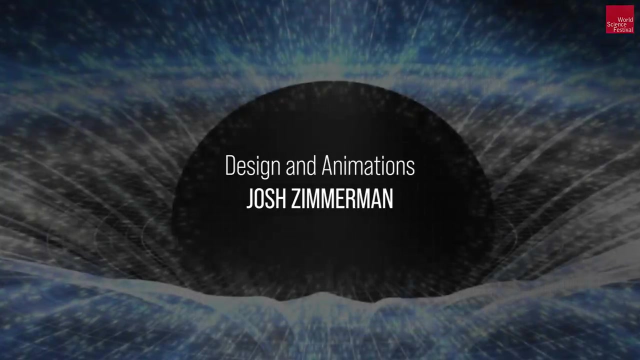 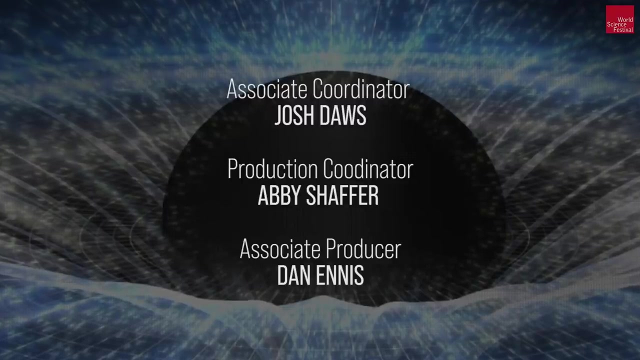 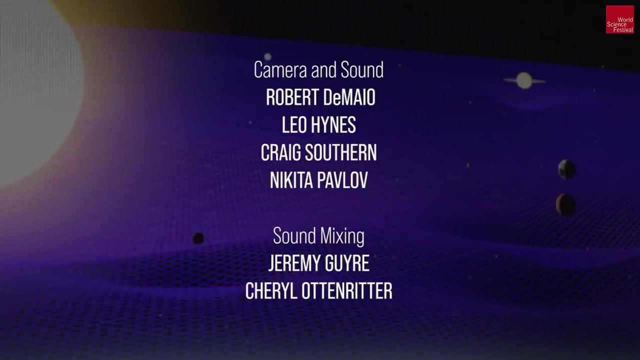 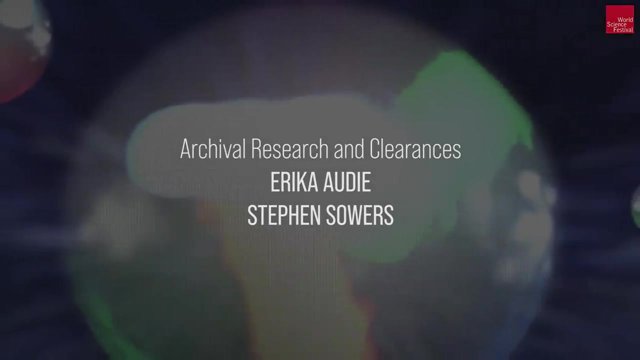 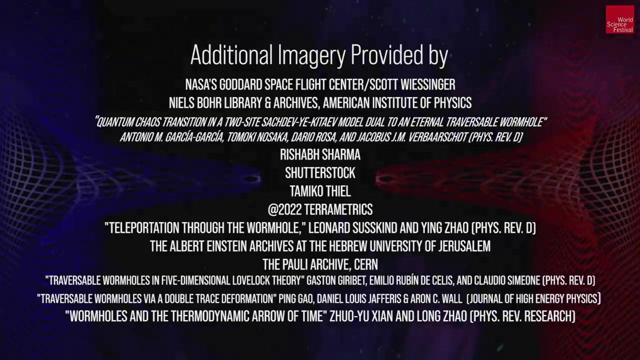 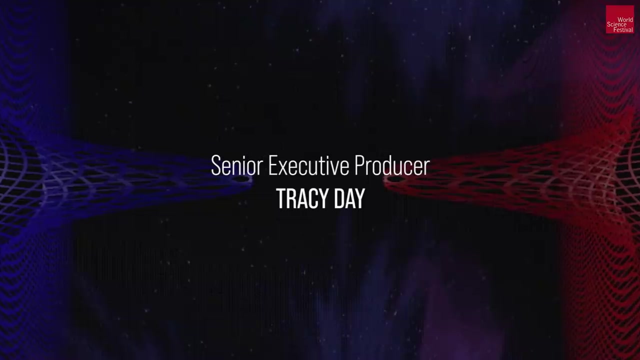 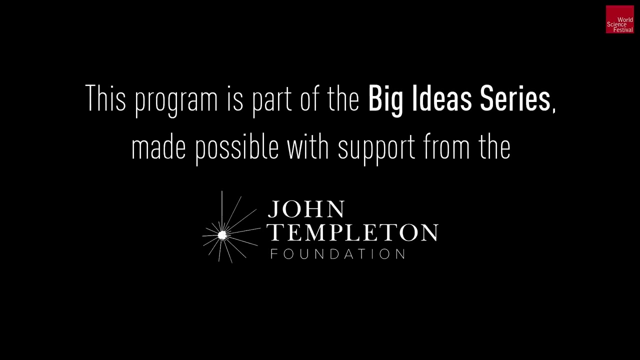 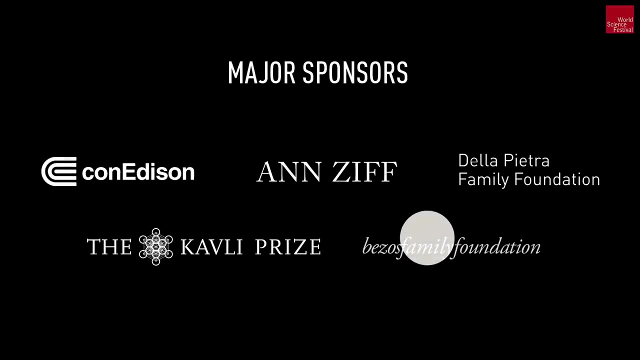 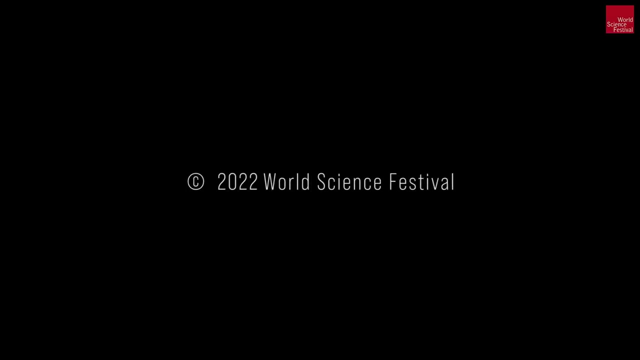 And thank you so much for spending some time today to talk about it. Thank you, Thank you, Thank you.